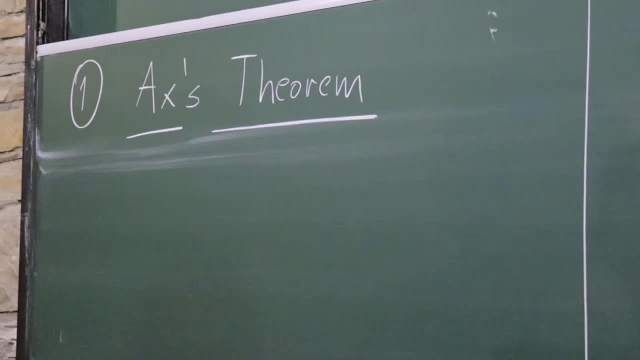 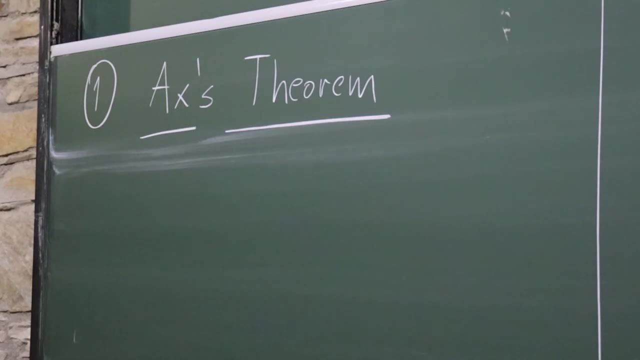 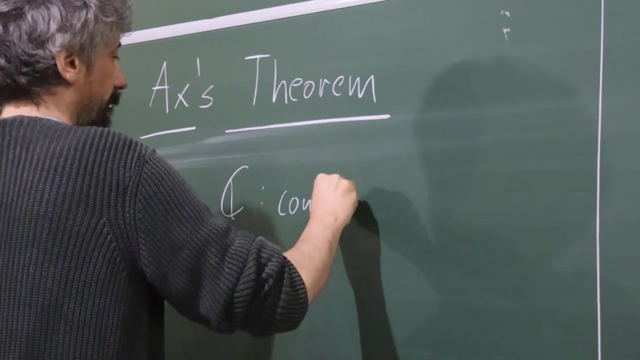 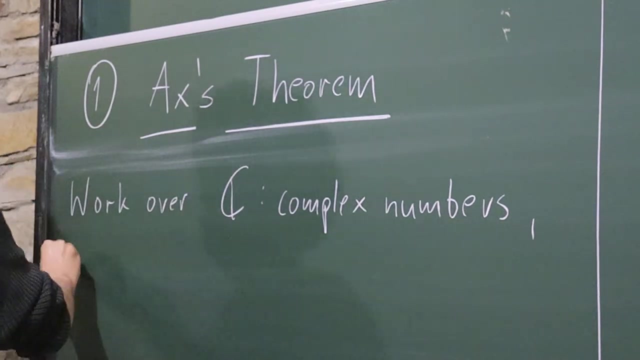 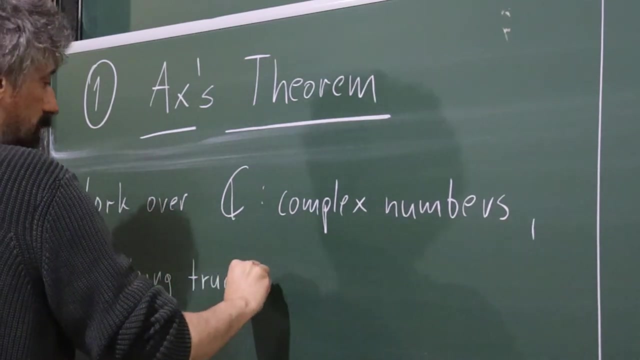 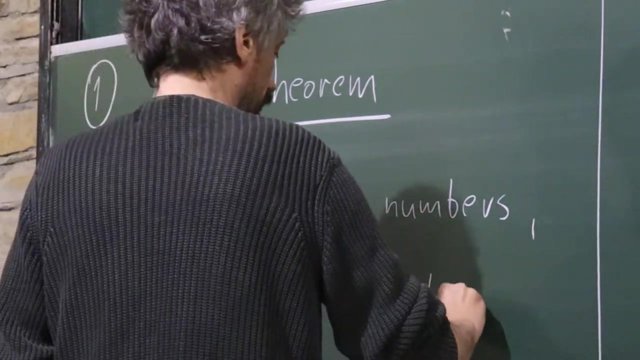 at the same time. so some people call it Ax's-Grotendieck theorem. So before stating it, Let us: Okay, We will work. so we will work over complex numbers, but everything will be true over any algebraically closed field. 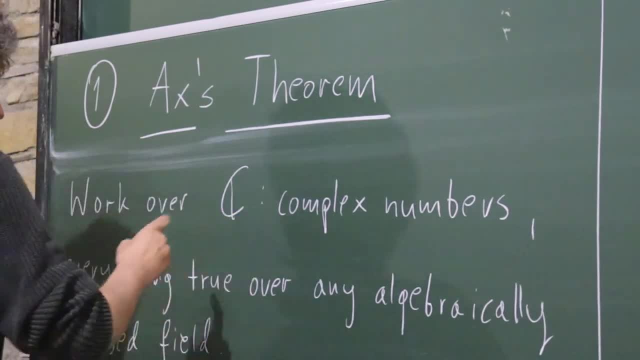 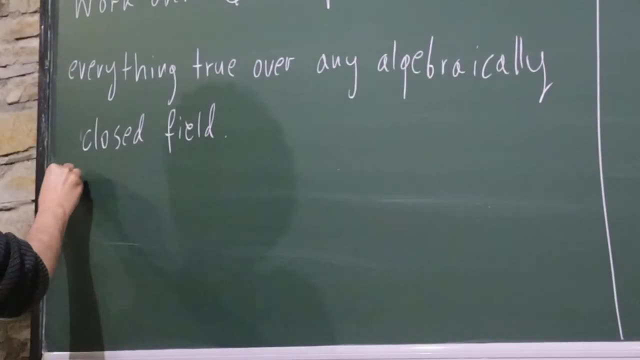 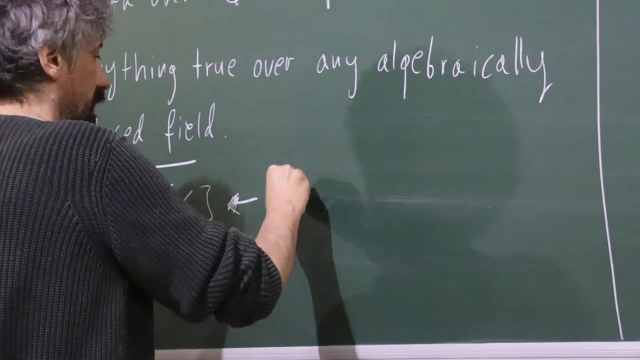 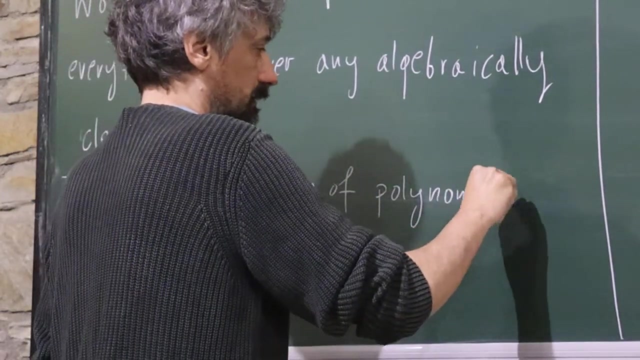 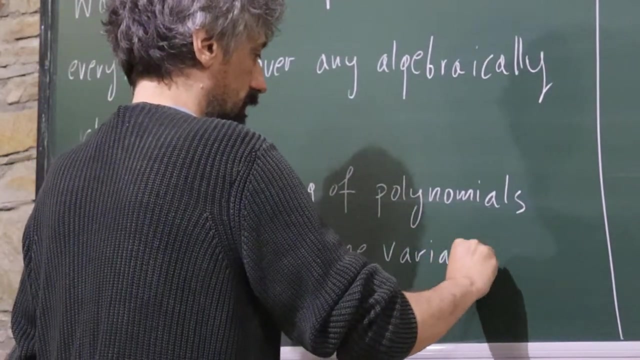 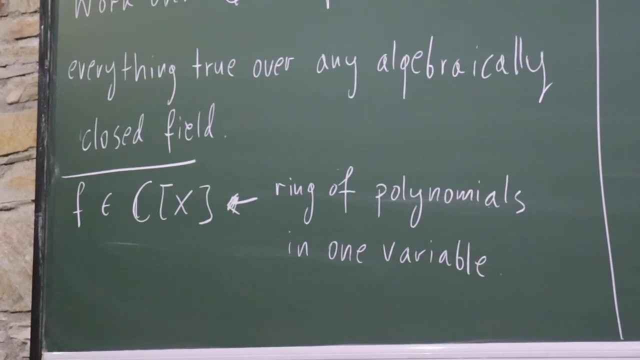 But to fix our attention, let us focus on this: complex numbers. So let us start from one polynomial. Okay, I am not sure, sure, so let me in the beginning try to describe everything. so this is ring of polynomials in one variable. how do I call it? okay, you remark, and also this f: 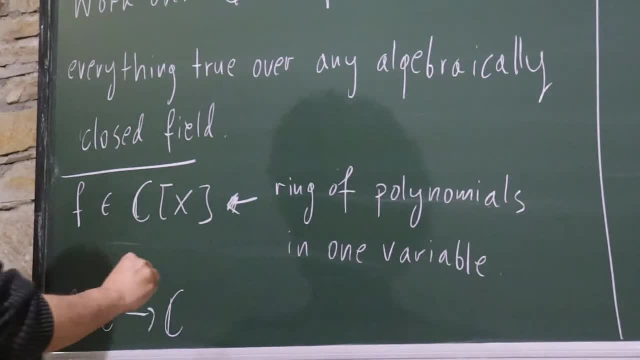 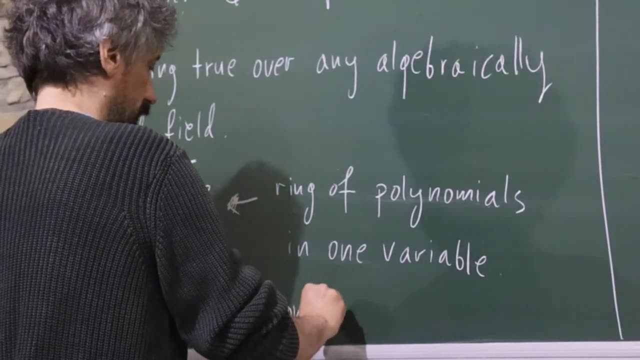 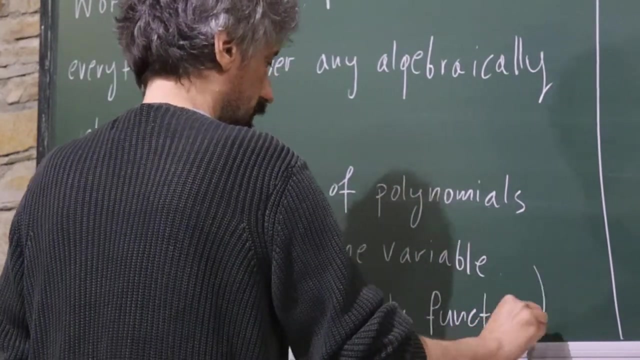 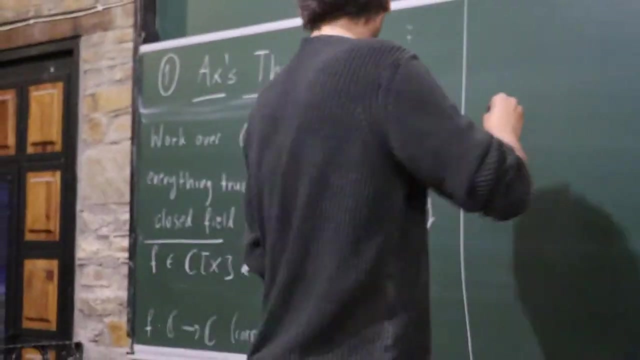 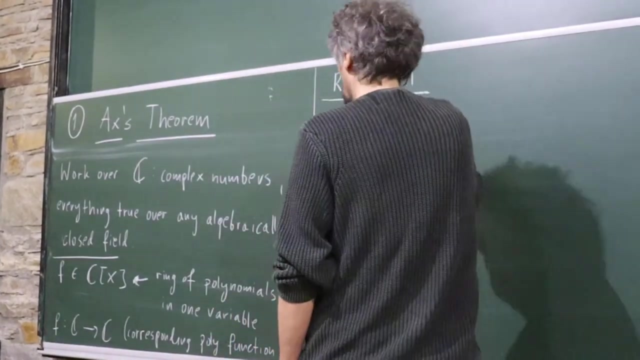 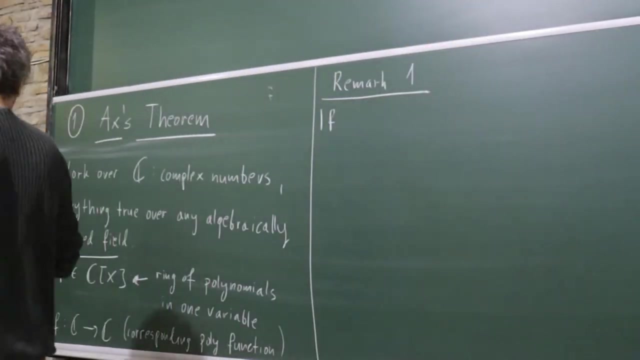 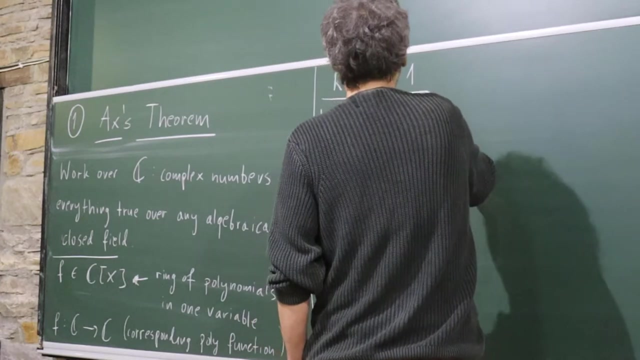 so by f I also denote the corresponding function, all right, so. so let's start from something very easy. so first remark, which is: may not look, it's not the best statement on its own, but it leads nicely to the access theorem. so it's quite easy to observe that if f is one to one, 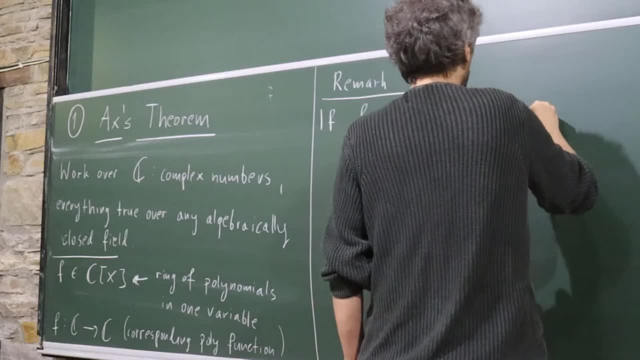 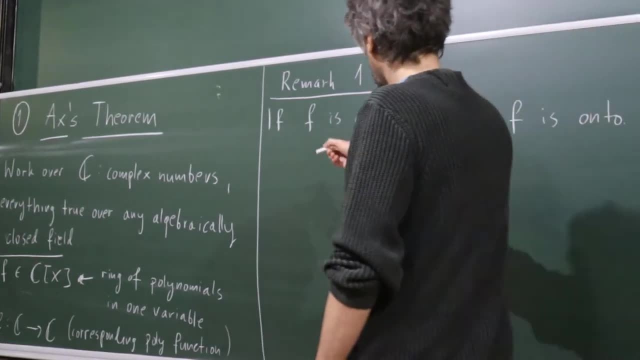 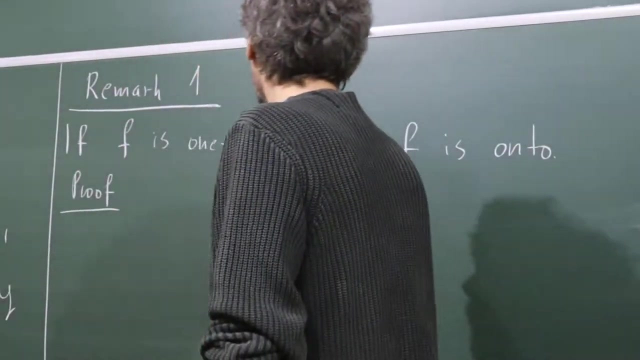 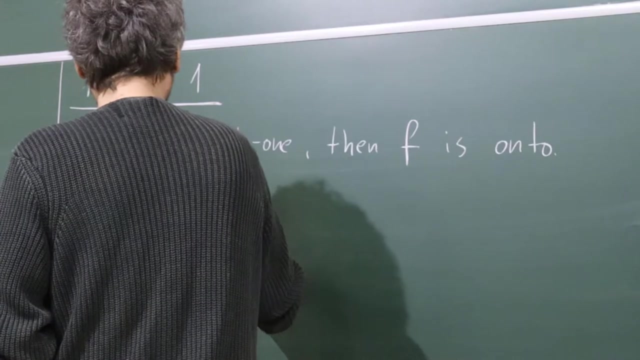 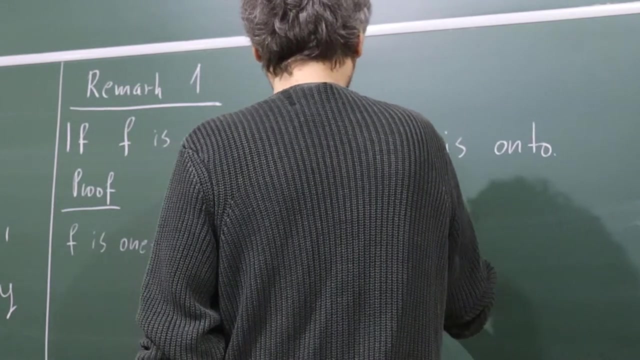 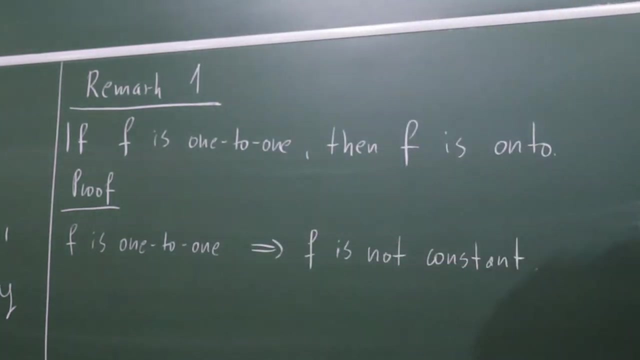 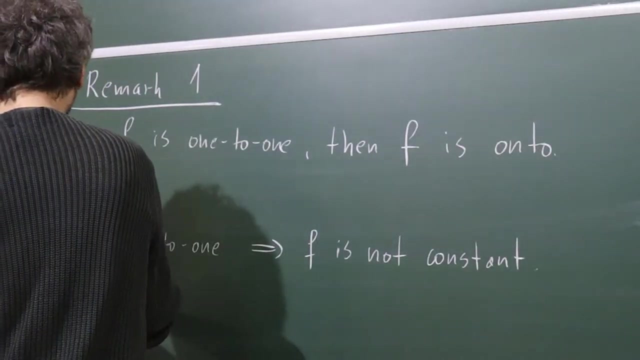 then f is onto. so let's prove it. actually, much less will be used than one to one. so prove so. if f is one to one, then of course f cannot be constant. so actually this will be enough to show over c that f is onto. so now take any element in c. 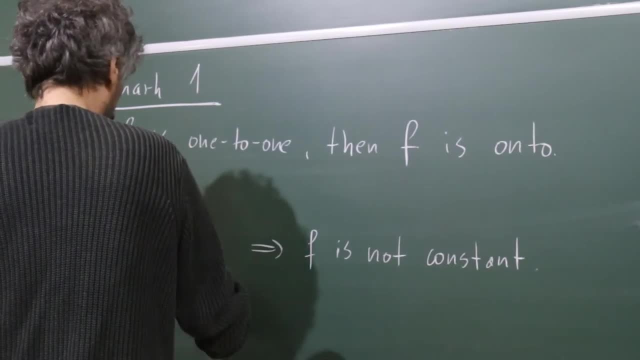 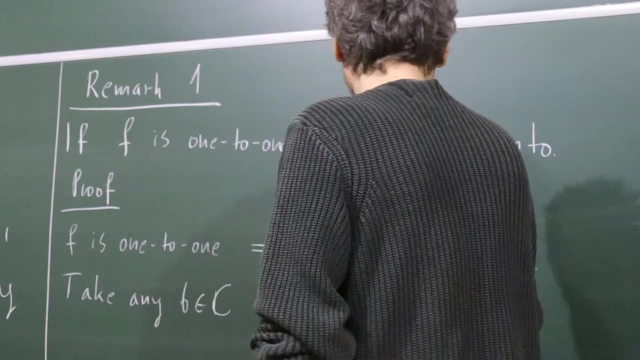 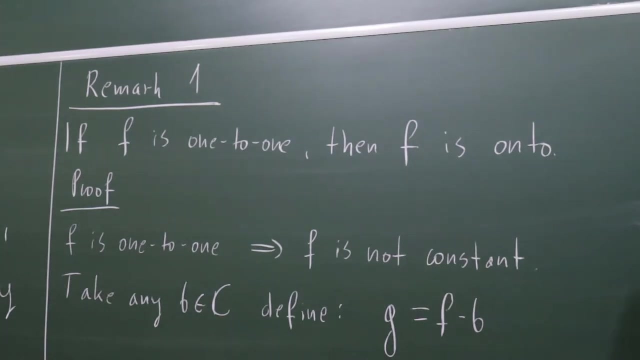 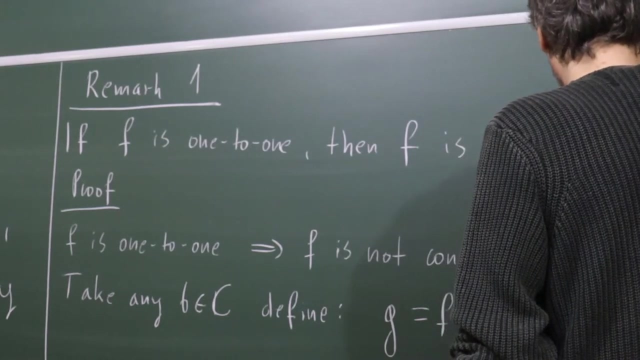 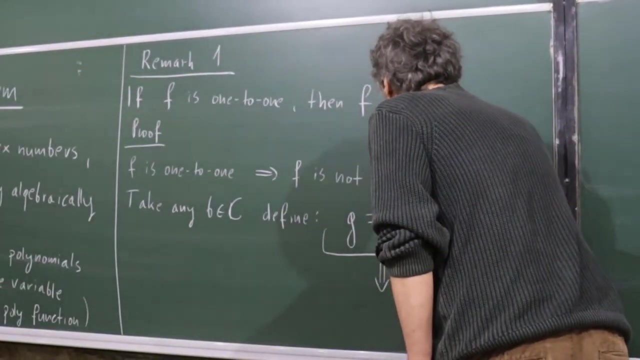 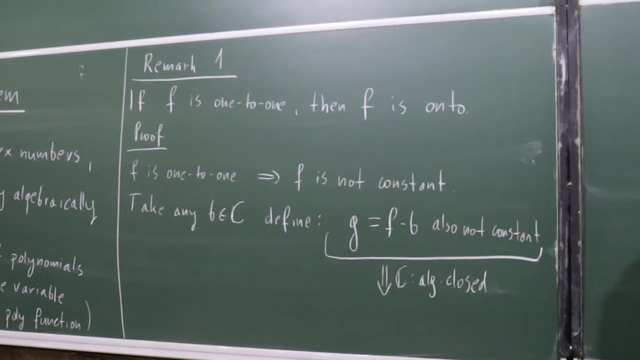 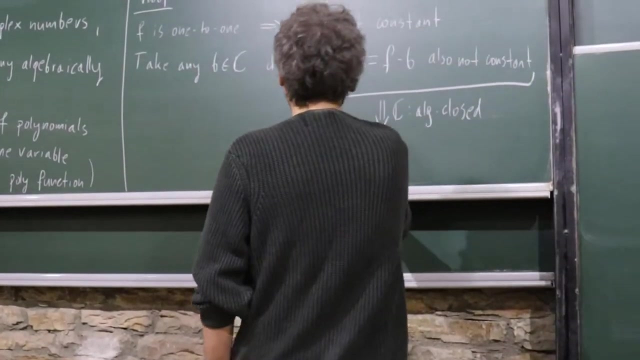 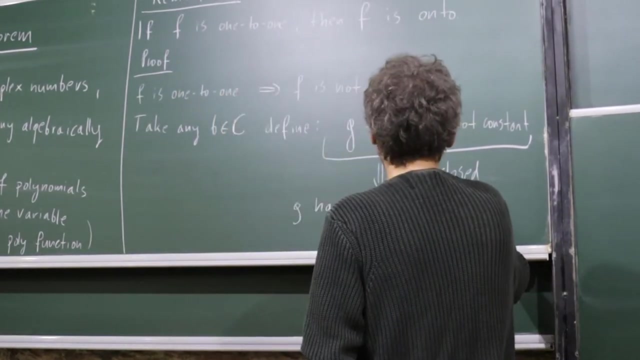 and define new polynomial. so this one, since we subtract constant, is also not constant. so, because c is algebraically closed, every non-constant polynomial has a zero. so this g has a zero. some zero, let's say z. so this g has a zero. so this g has a zero. 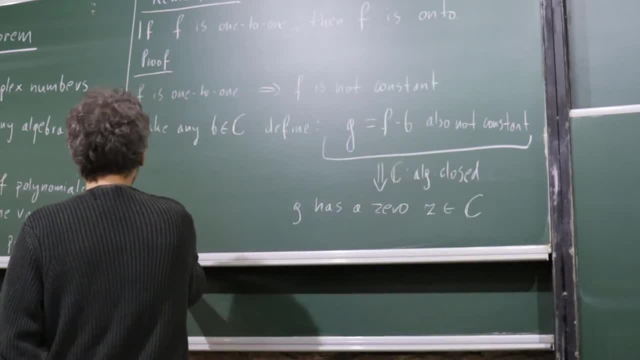 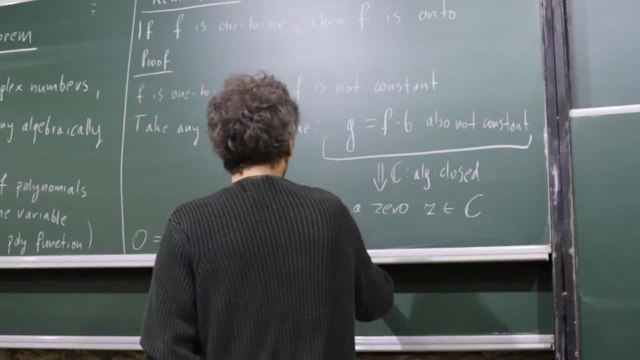 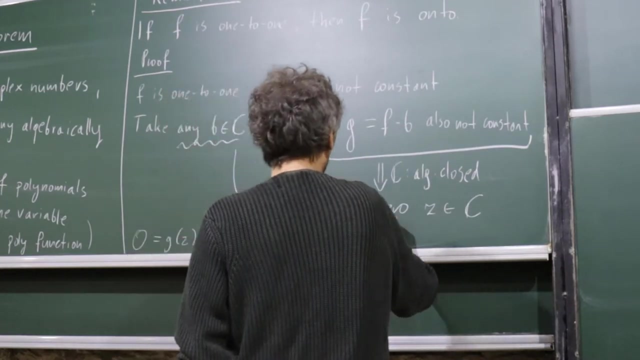 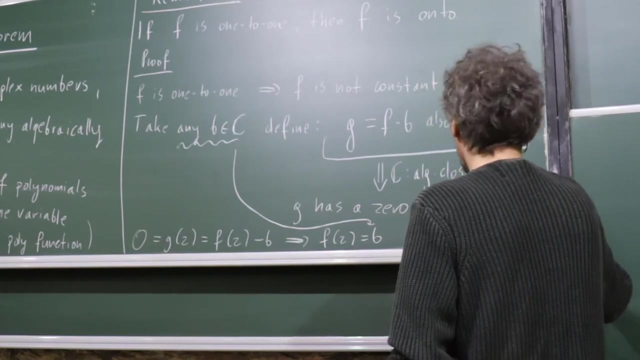 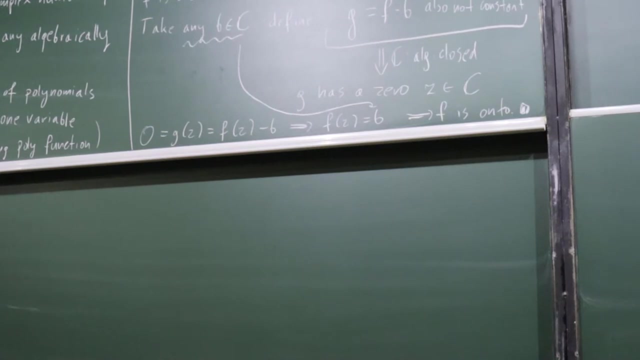 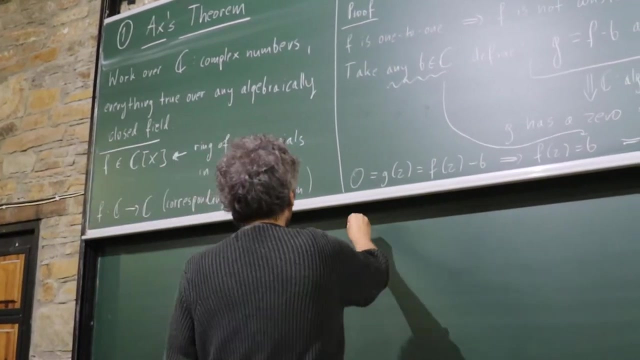 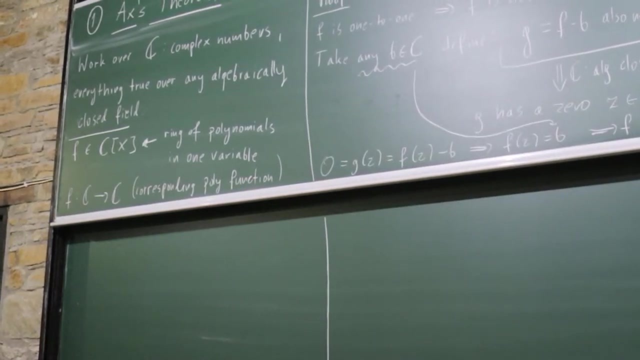 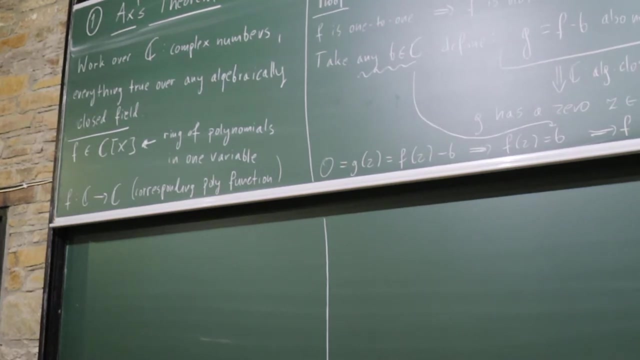 so then we see that zero g of z, so f of z is b, and this b was arbitrary, so f is onto, okay. so access theorem. so access theorem will be the statement, but generalized from one variable to n and variables. so now just some more remarks. so now, just some more remarks. 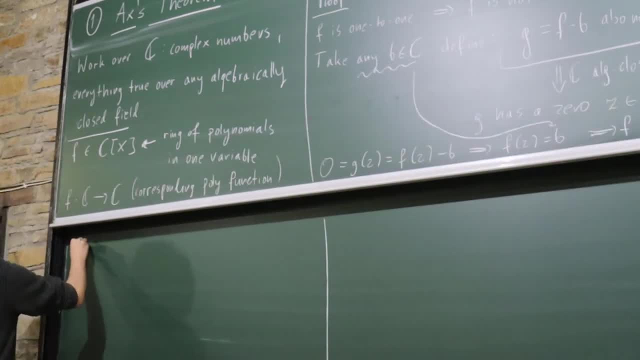 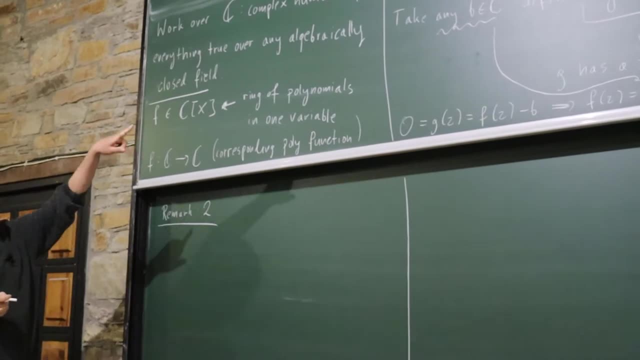 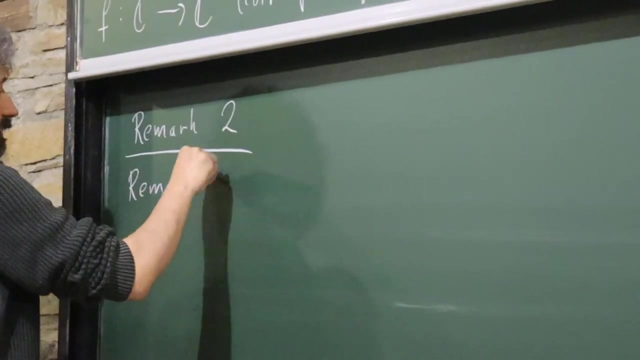 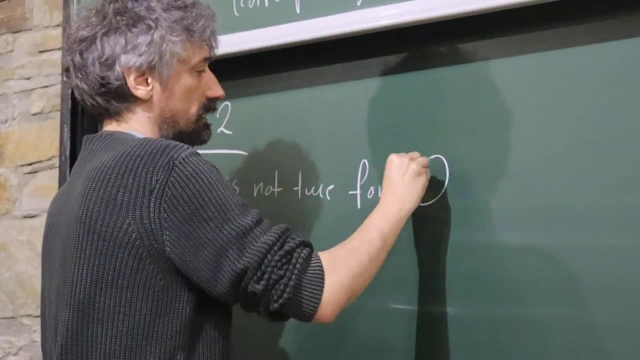 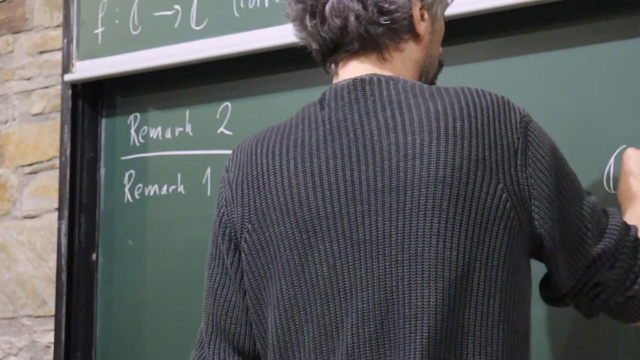 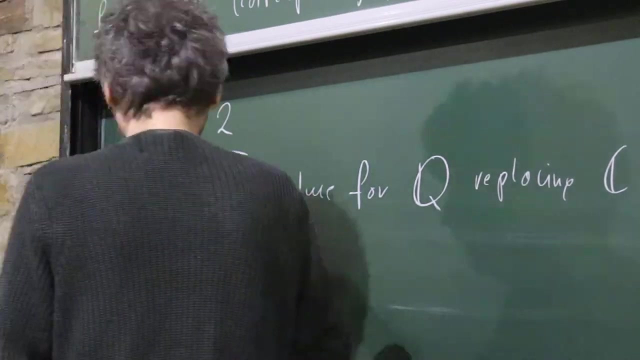 okay, so now just some more remarks. so remark two: it's of course not true for any field. so remark one is not true, for instance, for rationals replacing c. so take, so take, function x to power three. function x to power three. it is one to one, even on reals. 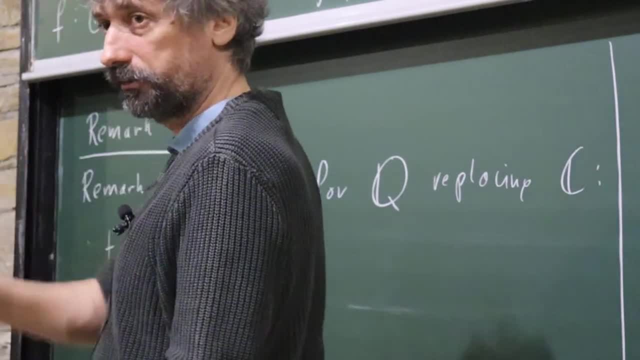 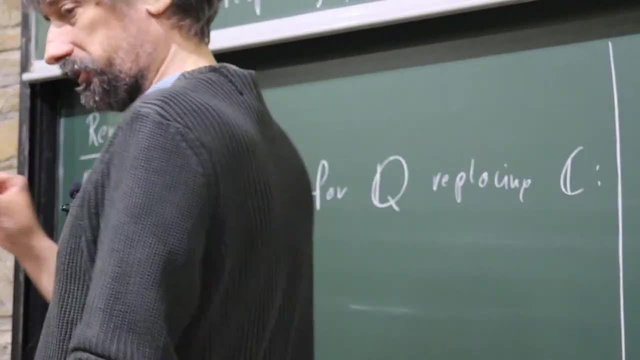 it is one to one, even on reals, but of course not every rational number is a third cube, but of course not every rational number is a third cube, so it's not always true. now problem, okay, so there will be problem. now problem, okay, so there will be problem. 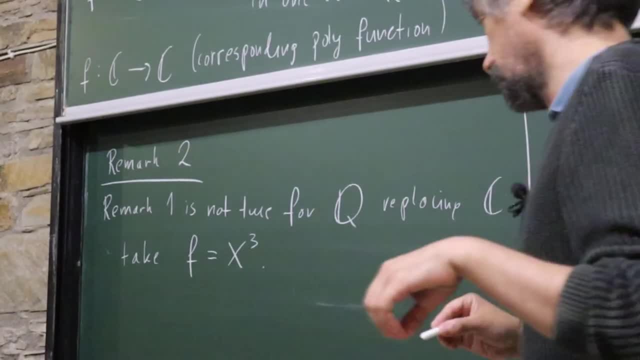 now problem. okay, so there will be problem. so problems will appear on the board. so problems will appear on the board. so problems will appear on the board. there is no problem list. there is no problem list. there is no problem list as such. so problem number one as such. so problem number one. 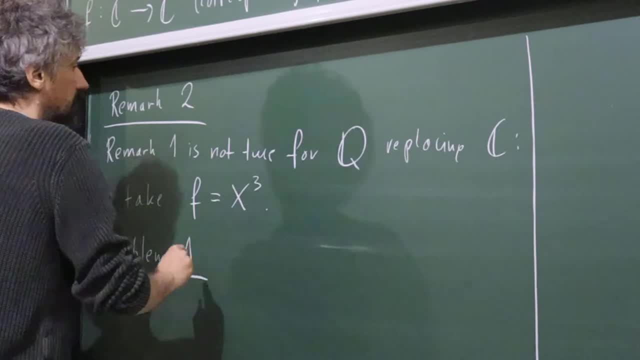 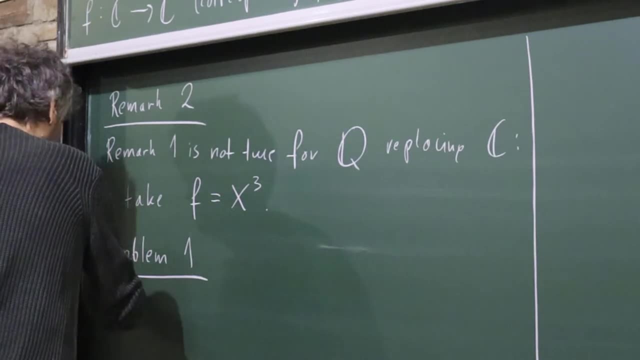 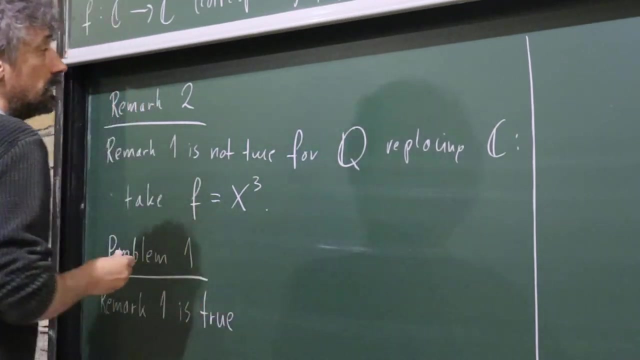 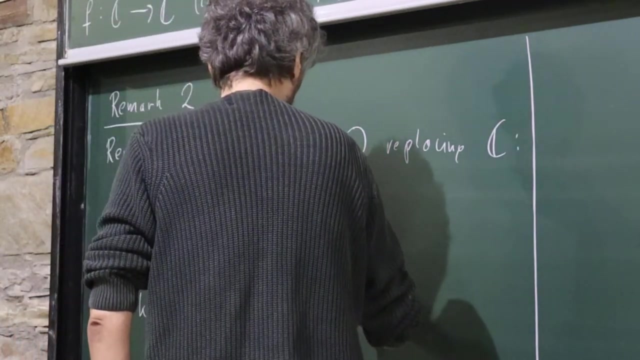 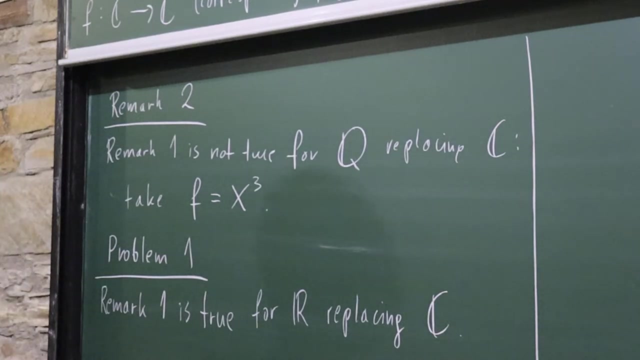 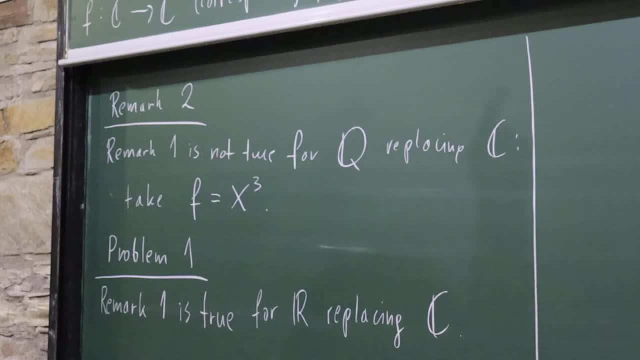 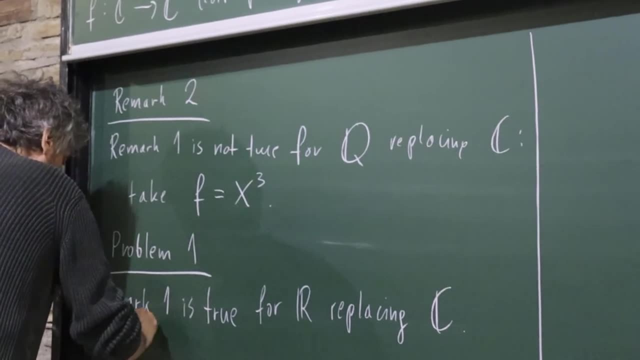 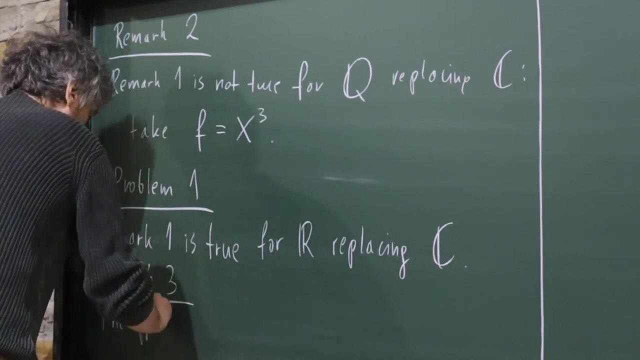 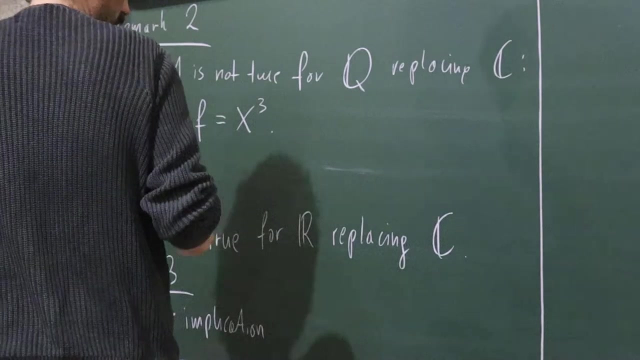 quite easy, quite easy, okay, and one can wonder, okay, and one can wonder, okay, and one can wonder: do we have opposite implication? do we have opposite implication? do we have opposite implication? but of course not. so let me write it: opposite implication in the reals. in the reals, mark one: 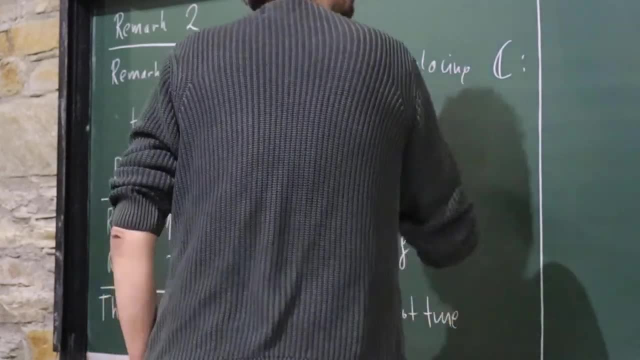 mark one. mark one is of course not true. is of course not true. is of course not true. let's take any polynomial of degree at. let's take any polynomial of degree at. let's take any polynomial of degree at least two, least two, least two. since he is algebraically closed, it is. 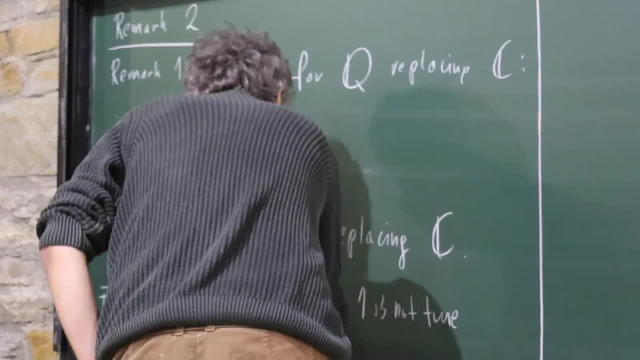 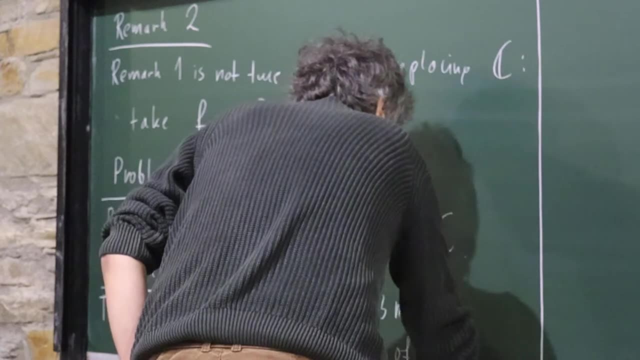 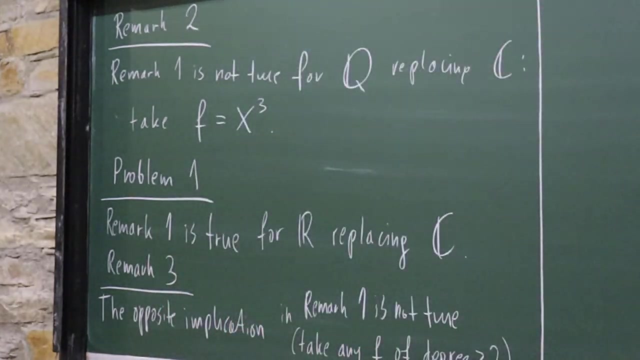 since he is algebraically closed. it is, since he is algebraically closed. it is onto, but it's not one to one onto, but it's not one to one. okay, any questions so far? this should be okay. any questions so far? this should be okay. any questions so far? this should be pretty easy. 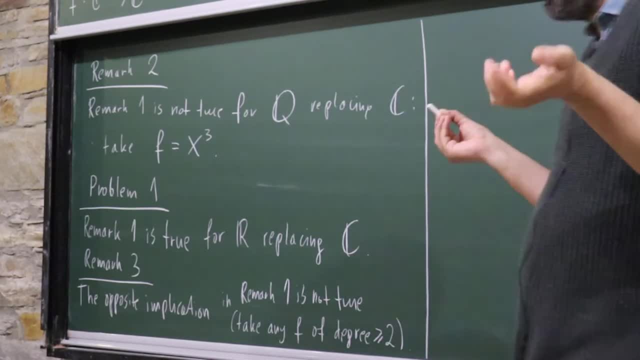 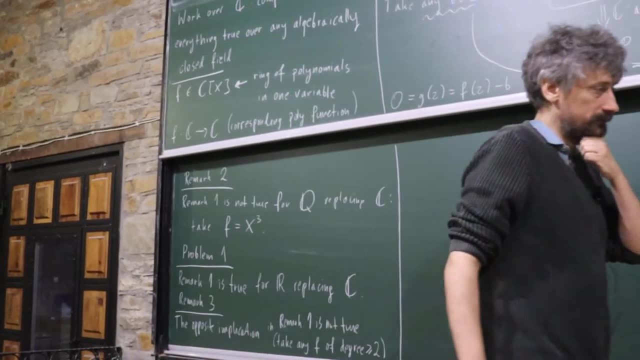 pretty easy, pretty easy, yes. so any non-constant polynomial on: yes. so any non-constant polynomial on: yes. so any non-constant polynomial on algebraic closed field is onto algebraic closed field is onto algebraic closed field is onto. but just linear ones are one-to-one. 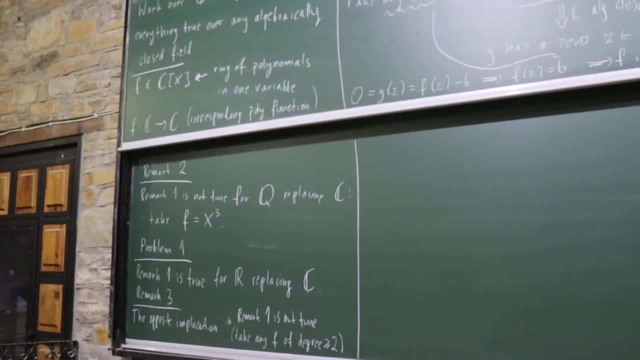 but just linear ones are one-to-one, but just linear ones are one-to-one. but the other one is true, so now. but the other one is true, so now. but the other one is true, so now, the axis theorem, as i said, would be. the axis theorem, as i said, would be. 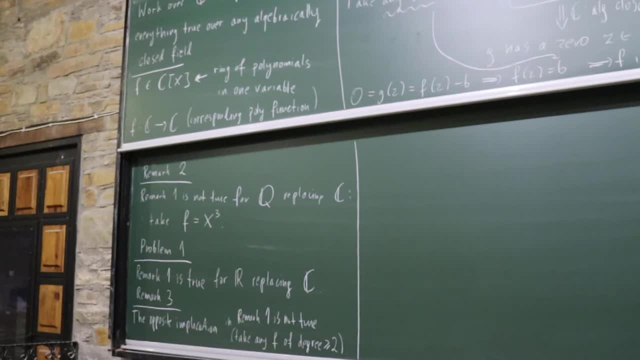 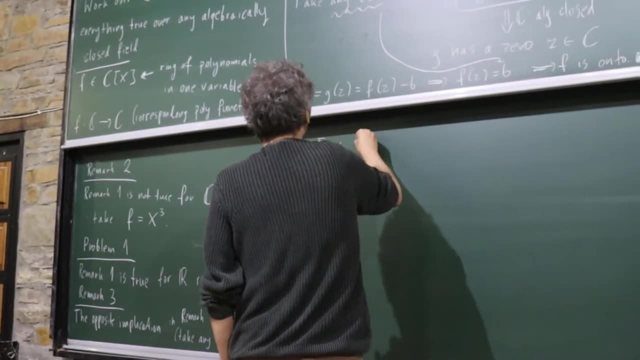 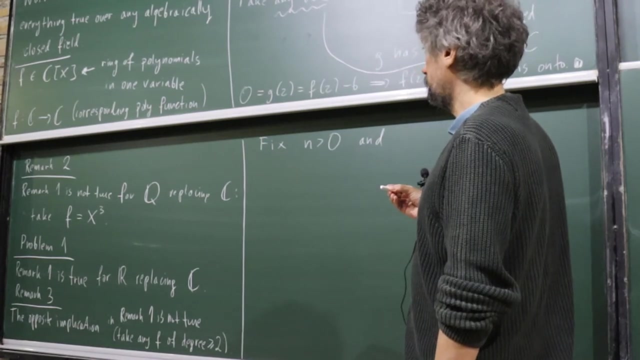 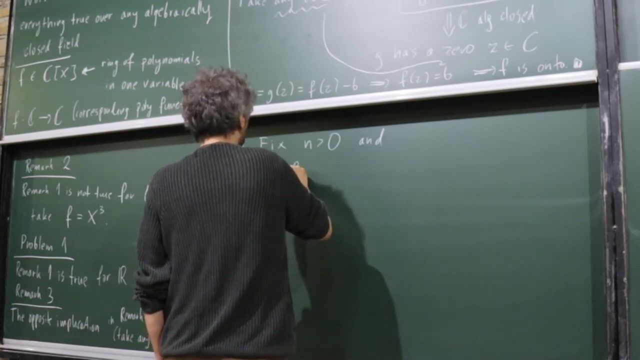 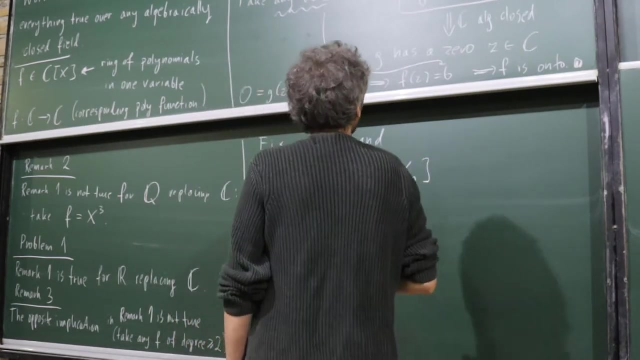 the axis theorem, as i said, would be generalization, generalization, generalization from one, from one, from one to to to more variables. so let us fix and fix now n polynomials in n and fix now n polynomials in n, and fix now n polynomials in n. variables over c. 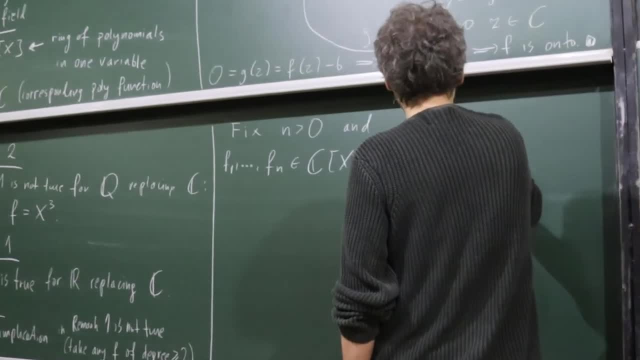 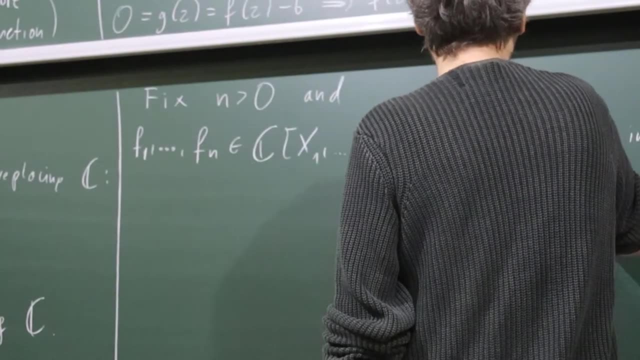 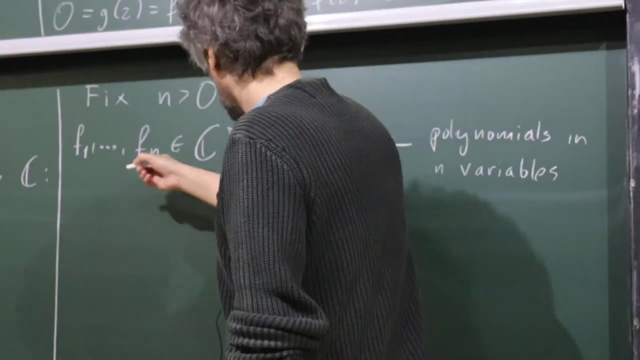 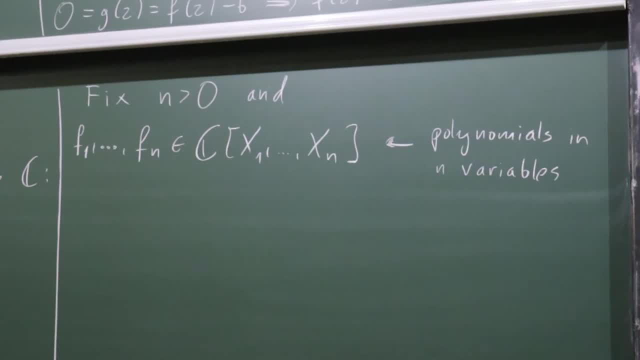 index appears twice, but it's not a index. appears twice, but it's not a mistake here. mistake here, mistake here: as many polynomials, as many variables, as many polynomials, as many variables, as many polynomials, as many variables. and now consider a function. and now consider a function. 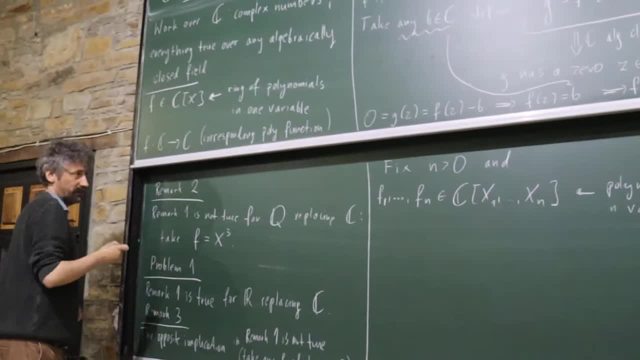 and now consider a function: okay, in this case, this function was okay, in this case, this function was okay. in this case, this function was basically the same as the polynomial, basically the same as the polynomial, basically the same as the polynomial. now we take, now we take. now we take one function using function. 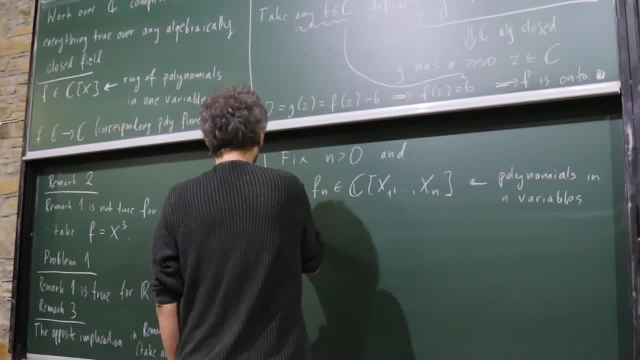 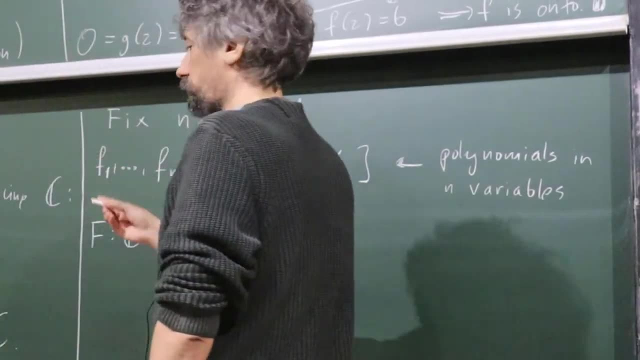 one function using function. one function using function, using this n polynomials, using this n polynomials, using this n polynomials. so consider, so consider. so consider capital f. just on each coordinate, it has this f1 up to. just on each coordinate, it has this f1 up to. 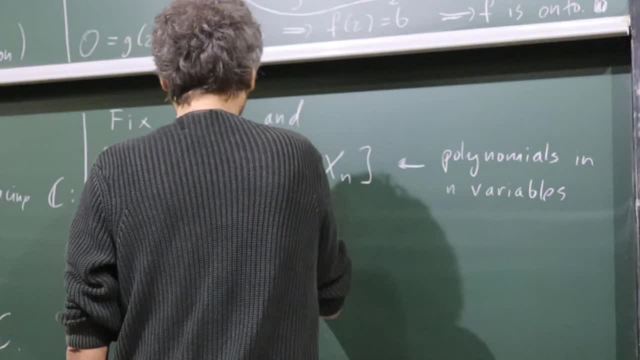 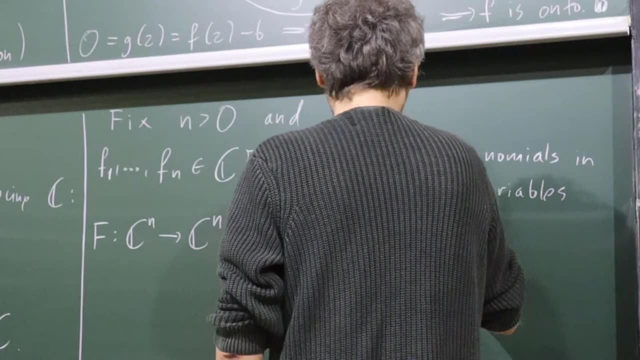 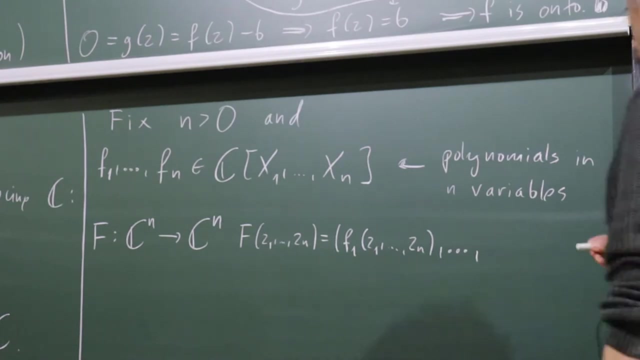 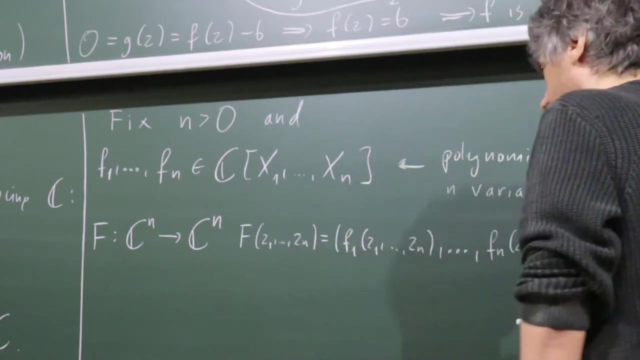 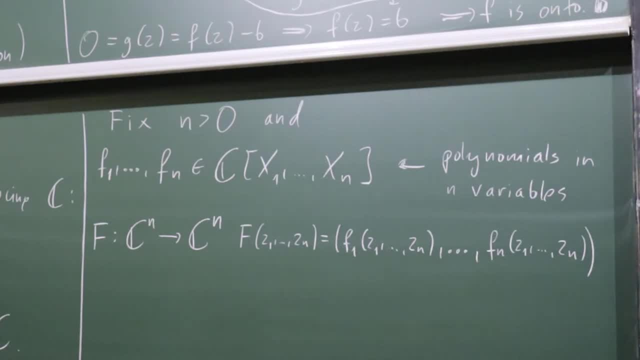 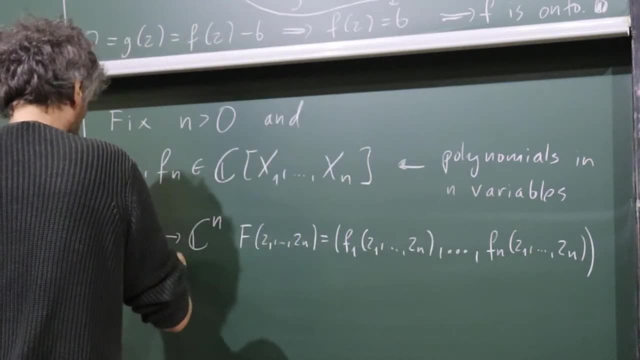 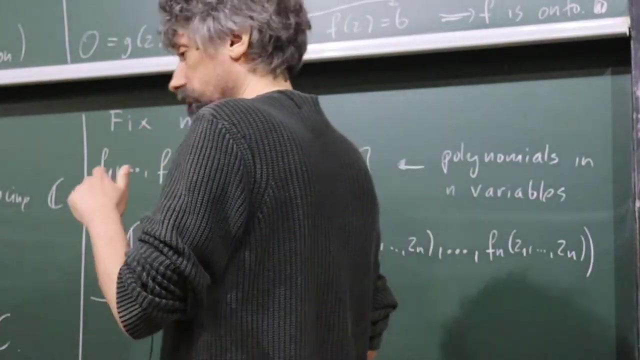 so the axis theorem is now like we mark. so the axis theorem is now like we mark. so the axis theorem is now like we mark one, but for capital f. so, as i said, some people say ax got. so, as i said, some people say ax got. so, as i said, some people say ax got and dick. but let me say just x. 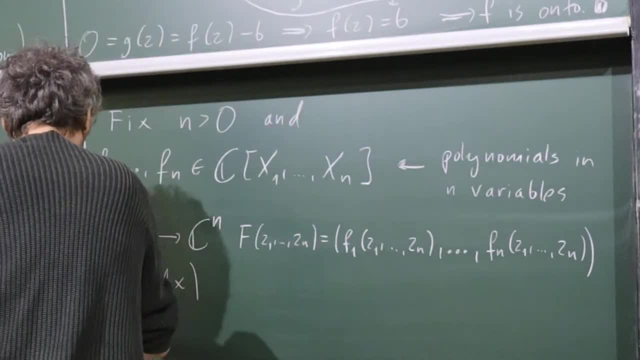 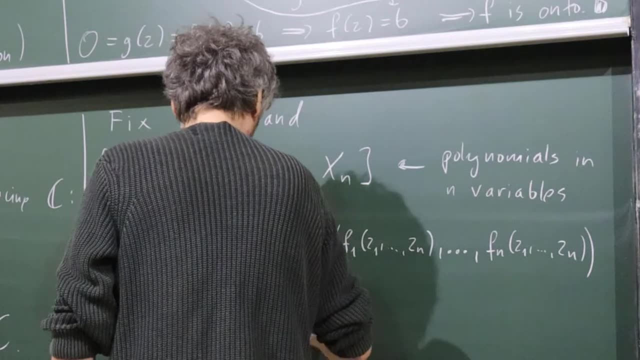 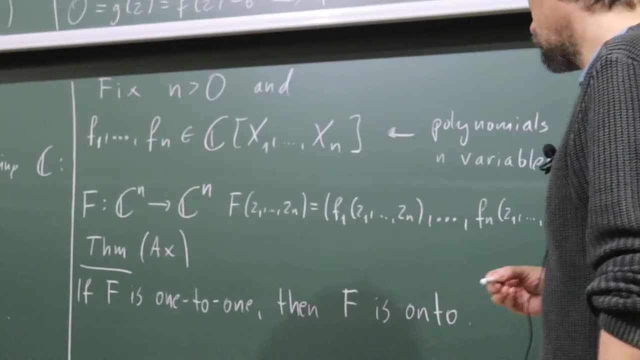 and dick, but let me say just x and dick, but let me say just x- sorry rotten dick, sorry rotten dick, sorry rotten dick. so if f is one to one, then f is on to okay. so we want to prove it. so this is okay. so we want to prove it. so this is. 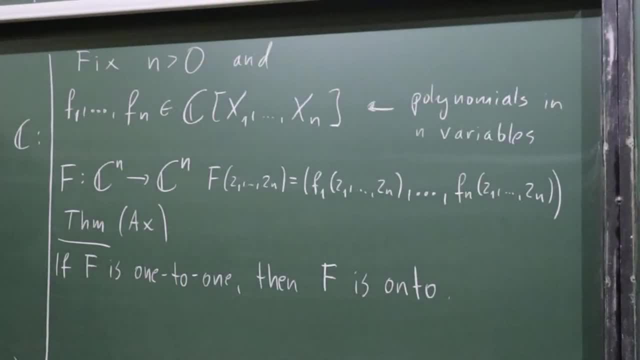 okay, so we want to prove it. so this is this first theorem. i want to prove this first theorem. i want to prove this first theorem, i want to prove using some model theory and that will using some model theory and that will using some model theory and that will motivate this. 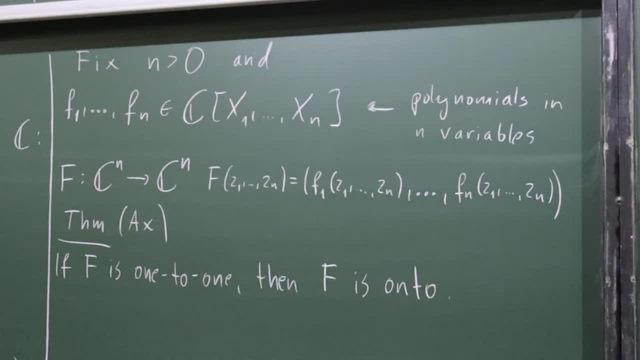 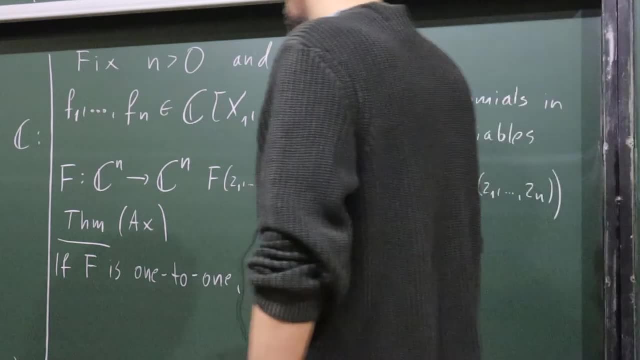 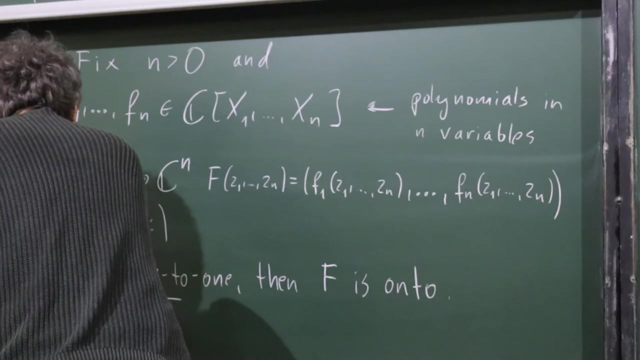 motivate this, motivate this notion, notion, notion, and statements from other theory which, and statements from other theory which and statements from other theory which will be used here, will be used here, will be used here. i need one, i need one, i need one little technical thing. so i will say: 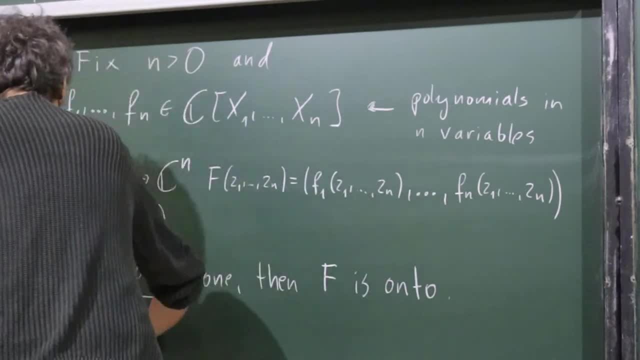 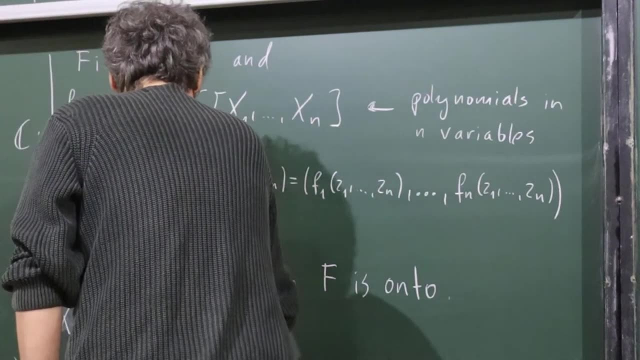 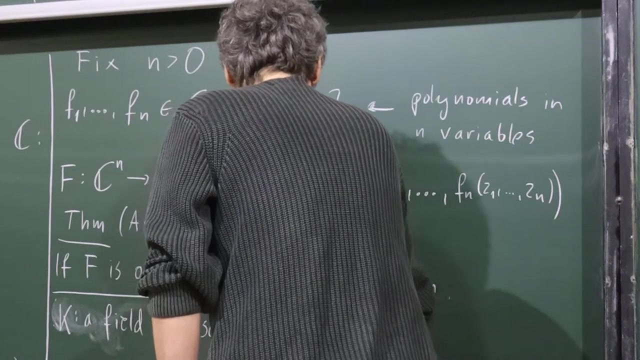 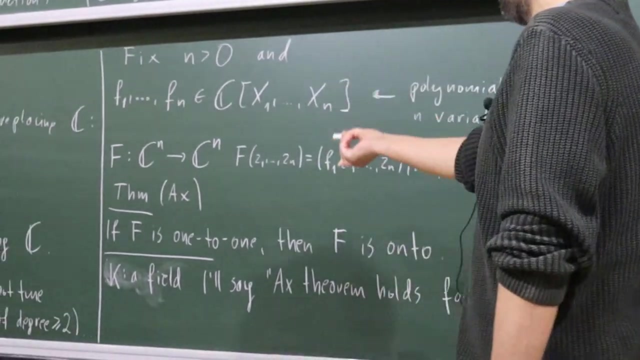 okay, let's okay, let's okay, let's now. k be any field. now, k be any field, now k be any field. so i say that x theorem holds for k, holds for k, holds for k. well, if, well, if well, if. if it holds for k, yes, if. 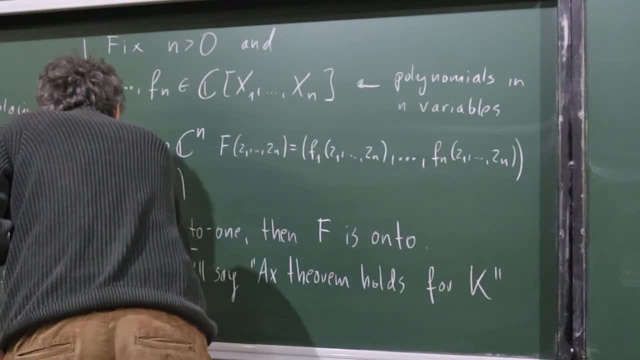 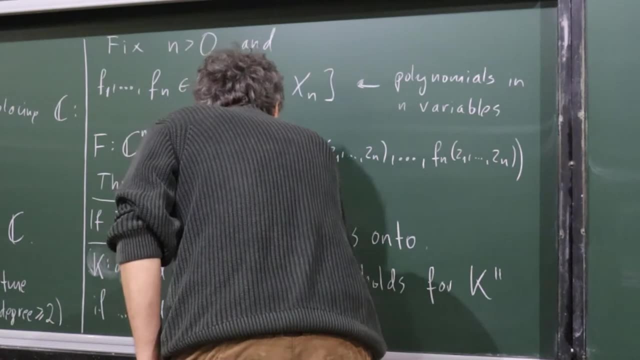 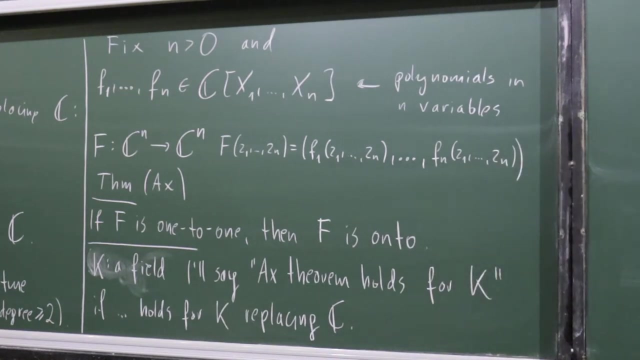 if it holds for k, yes. if. if it holds for k, yes. if. if the above statement is okay, replacing c is okay, replacing c is okay replacing c. so of course, it's also interesting to ask so, of course it's also interesting to ask. so of course, it's also interesting to ask, for which other fields? 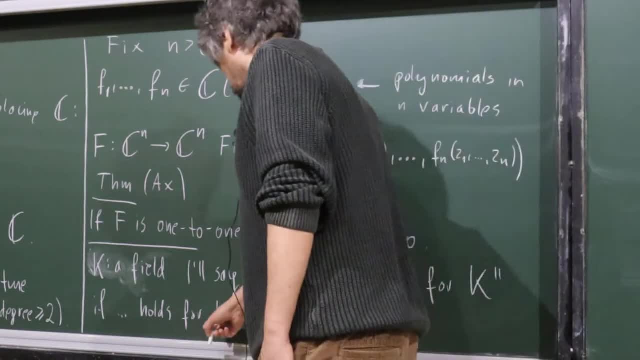 for which other fields? for which other fields? this is true, this is true. this is true, but in the proof i will need to use. but in the proof i will need to use. but in the proof i will need to use, i will. first i will show that axis theorem. 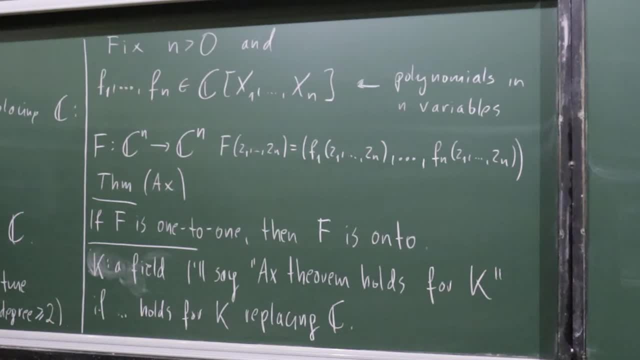 i will first i will show that axis theorem. i will first i will show that axis theorem: holds for some other fields and from holds for some other fields and from holds for some other fields and from these other fields, i will get into c, these other fields, i will get into c. 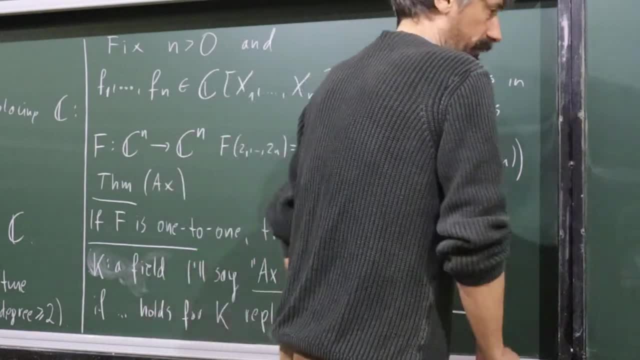 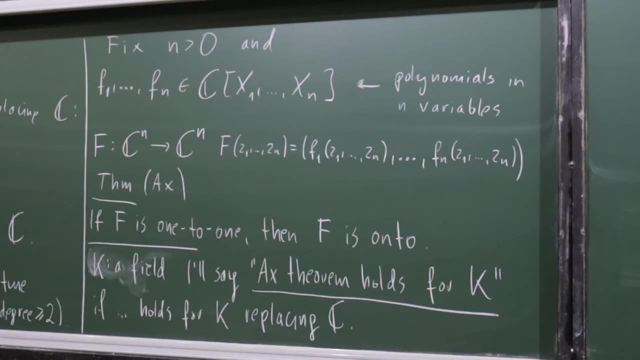 these other fields i will get into c. that's why i need to have, that's why i need to have, that's why i need to have such a notion, such a notion, such a notion, so maybe first before the proof, so maybe first before the proof, so maybe first before the proof, kind of examples, when it holds. 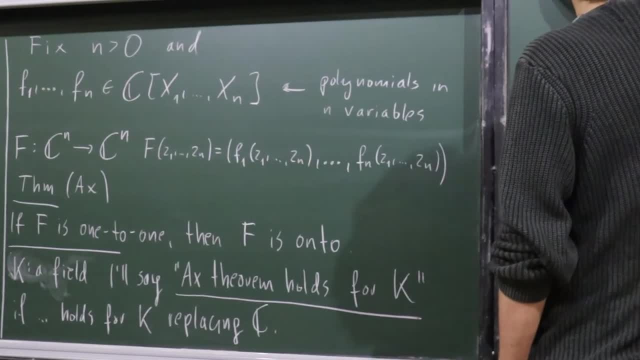 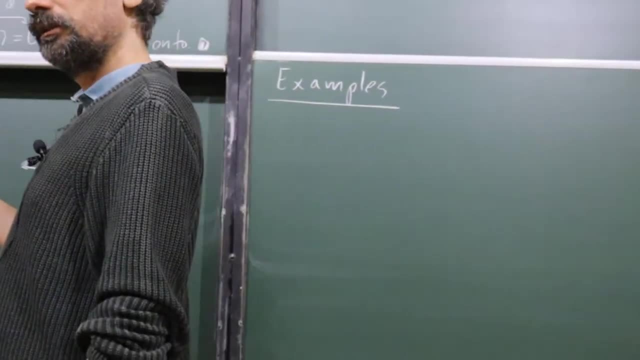 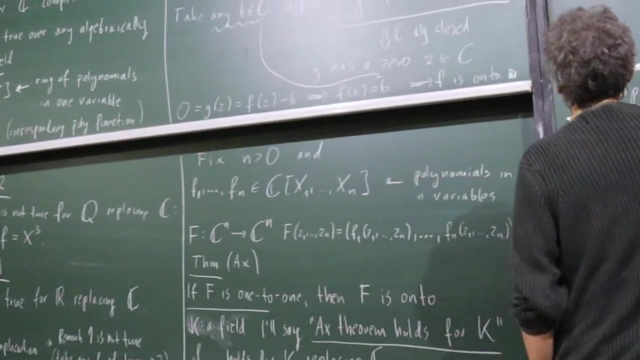 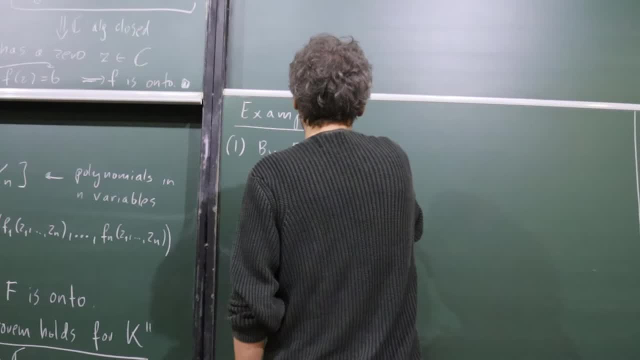 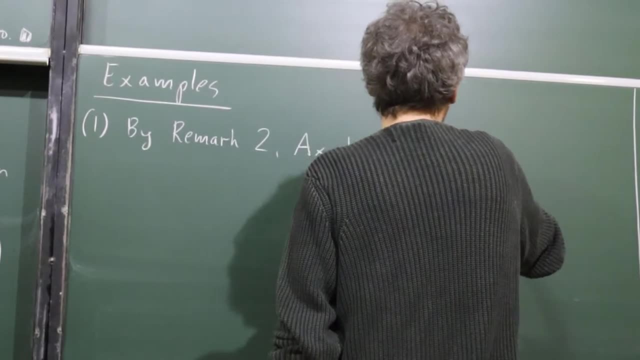 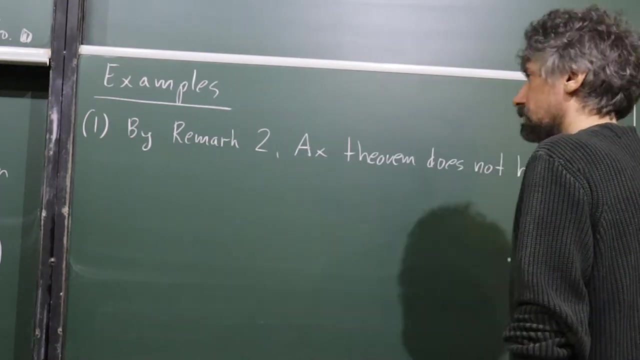 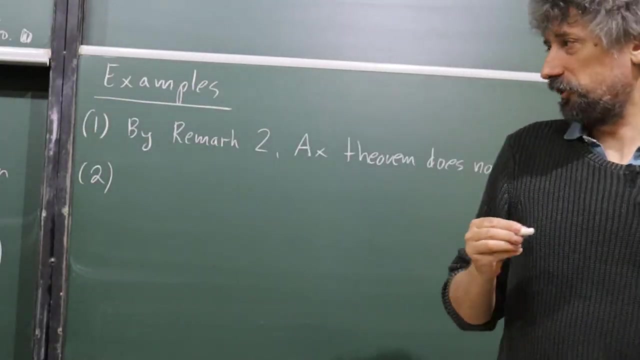 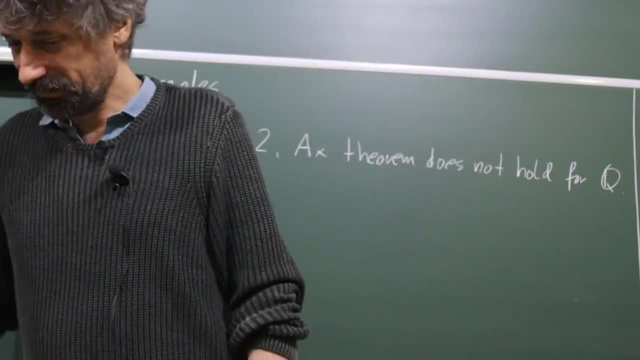 that probably it also does not hold for r, r, r, but i couldn't find any example, but i couldn't find any example, but i couldn't find any example, and then i started to search and it, and then i started to search and it, and then i started to search and it turns out that it holds for r. 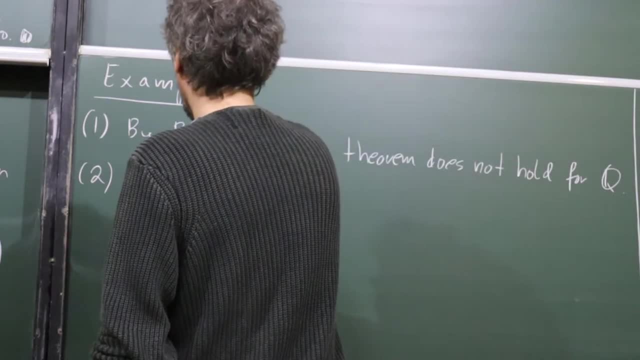 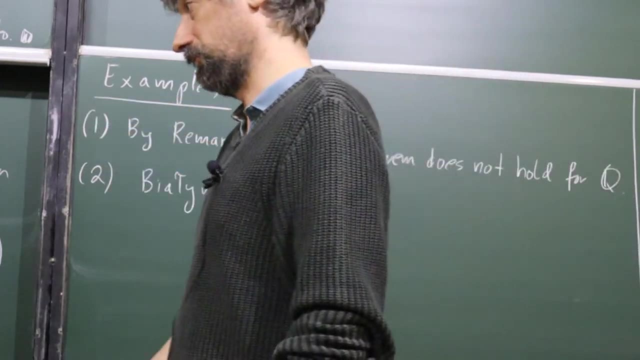 turns out that it holds for r, turns out that it holds for r. so there is quite, quite, quite, and funny thing is it was proved even. and funny thing is it was proved even. and funny thing is it was proved even before x prove it for c, before x prove it for c. 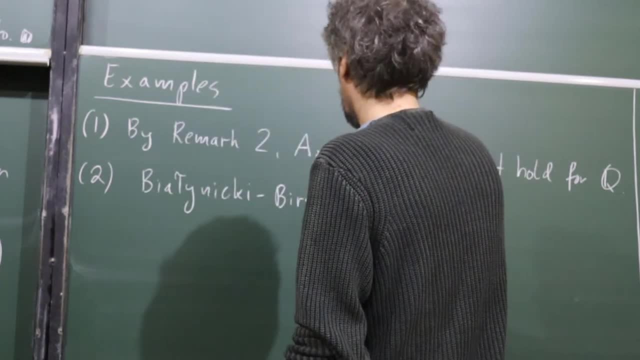 before x. prove it for c. i didn't know that, i didn't know that. i didn't know that, just just just. yeah, we need to keep it all out together. yeah, we need to keep it all out together. yeah, we need to keep it all out together. where? 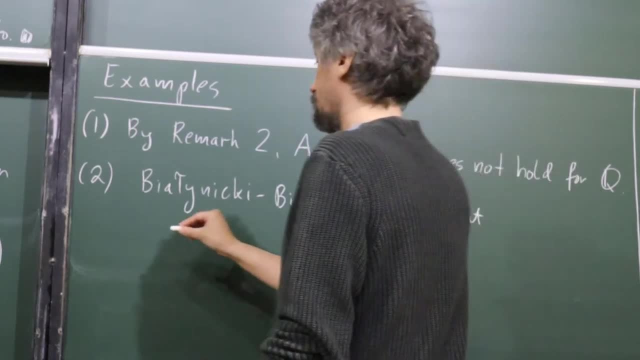 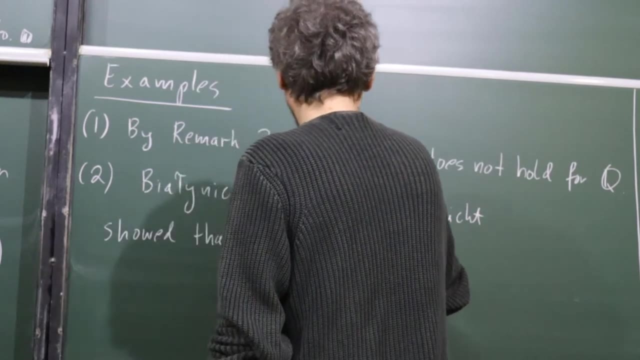 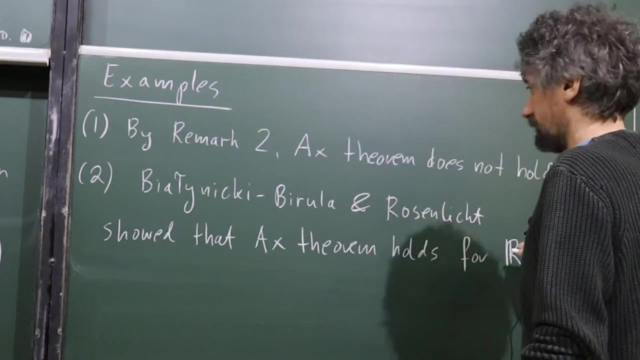 where? where? rosenlicht, rosenlicht, rosenlicht. so that, so that, so that ax theorem holds for r, holds for r, holds for r. so i'm just saying it on the side, we will. so i'm just saying it on the side, we will. so i'm just saying it on the side, we will not discuss it. 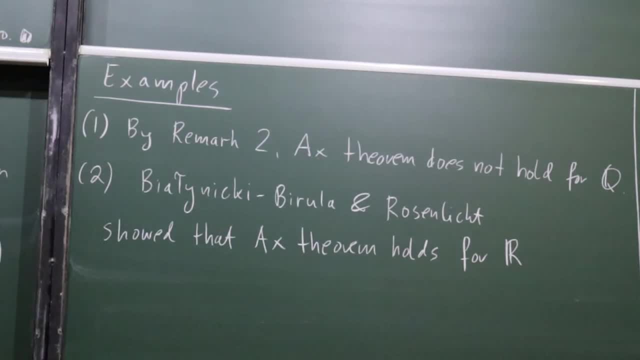 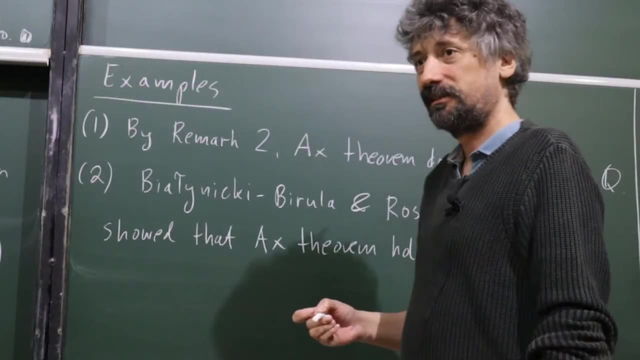 not discuss it. not discuss it, but okay, it's more complicated. more, but okay, it's more complicated more, but okay, it's more complicated. more complicated argument than for c. complicated argument than for c. complicated argument than for c, but it also holds for r, but it also holds for r. 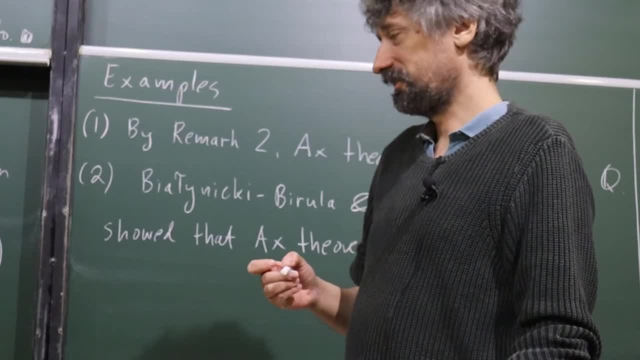 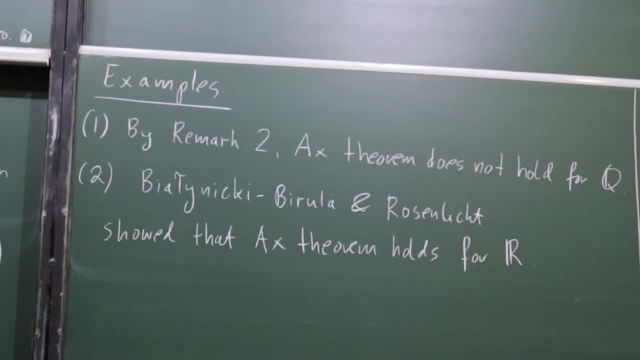 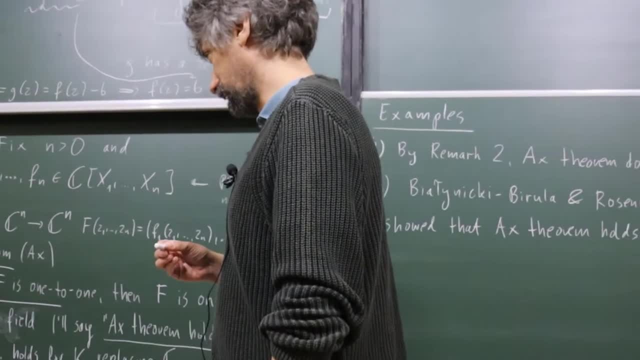 called brauer invariance of domain. so it says so. it says so. it says there is a old theorem of brauer saying there is a old theorem of brauer saying there is a old theorem of brauer saying that any, that, any, that, any, any continuous one-to-one function from 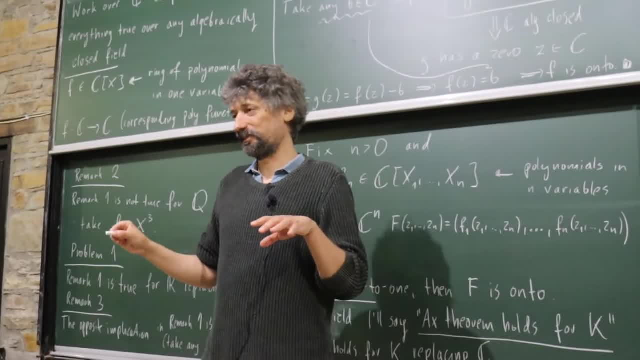 any continuous one-to-one function from. any continuous one-to-one function from rn to rn is open. rn to rn is open. rn to rn is open. takes open sets to open sets and then takes open sets to open sets, and then takes open sets to open sets and then, using this- i didn't look at the full- 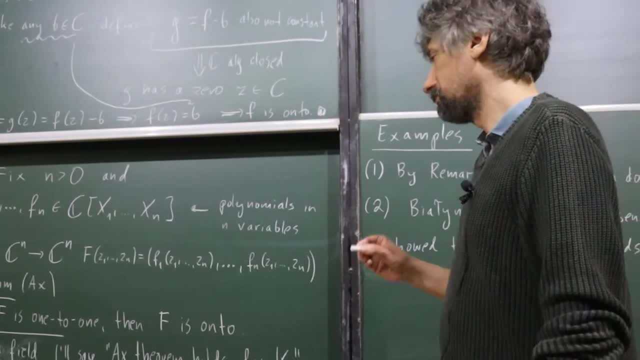 using this, i didn't look at the full. using this, i didn't look at the full argument. awesome cohomology, it's it's argument. awesome cohomology, it's it's argument. awesome cohomology, it's it's topological, geometric argument and such. 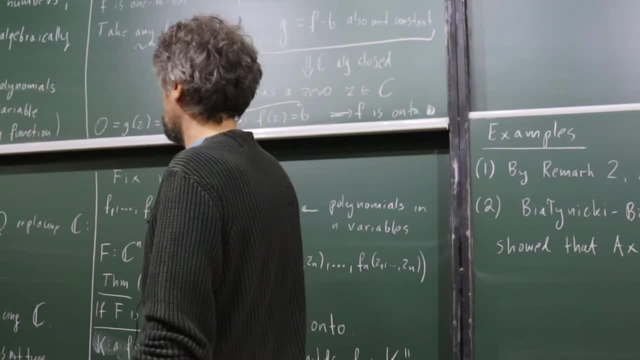 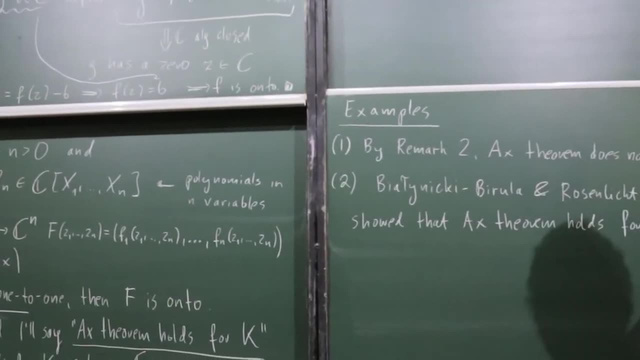 topological geometric argument and such topological geometric argument and such arguments also, arguments also, arguments also also may work for axiom. also may work for axiom, also may work for axiom, but i will show the other, but i will show the other, but i will show the other. another argument: 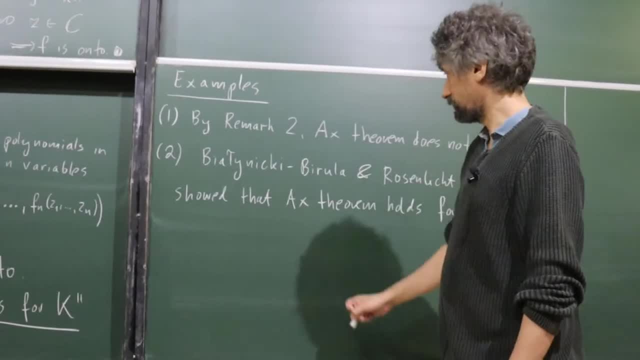 another argument. another argument and, just by coincidence, so this is, and just by coincidence, so this is, and just by coincidence, so this is. this was pretty famous polish algebraic. this was pretty famous polish algebraic. this was pretty famous polish algebraic. geometry, geometry, geometry. and i just got an email. 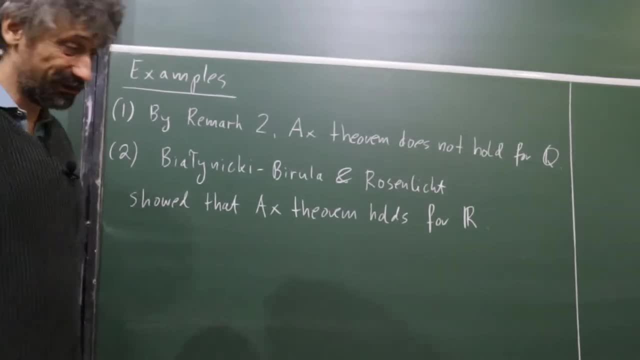 and i just got an email. and i just got an email that he died on monday, that he died on monday, that he died on monday, 85 years old, 85 years old, 85 years old. so so so. somehow his name often pops up like in: somehow his name often pops up like in: 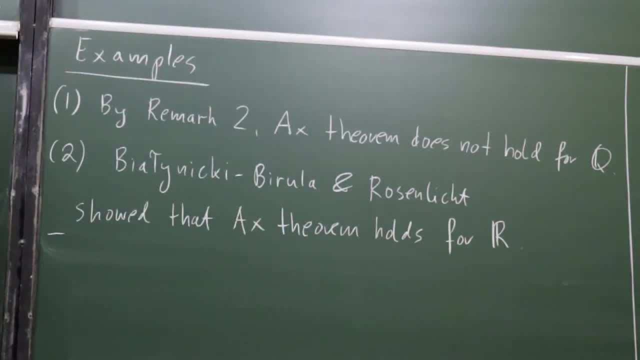 somehow his name often pops up like in 60s he was doing things which had kind 60s. he was doing things which had kind 60s. he was doing things which had kind of flavor of model theory, of flavor of model theory, of flavor of model theory. also some like: okay, it's another topic. 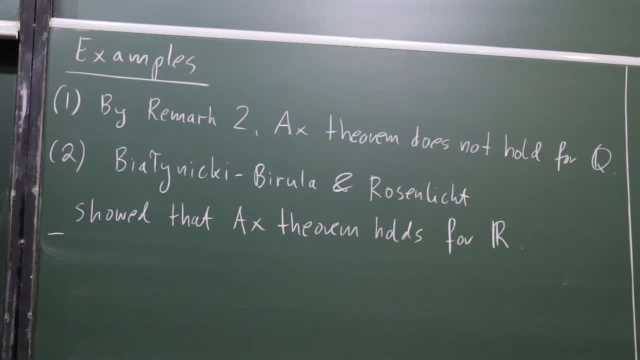 also some like: okay, it's another topic. also some like: okay, it's another topic, like like like difference differential galois theory, difference differential galois theory, difference differential galois theory, some things with operators also, some some things with operators also, some some things with operators, also some universal algebra, and then he moved to. 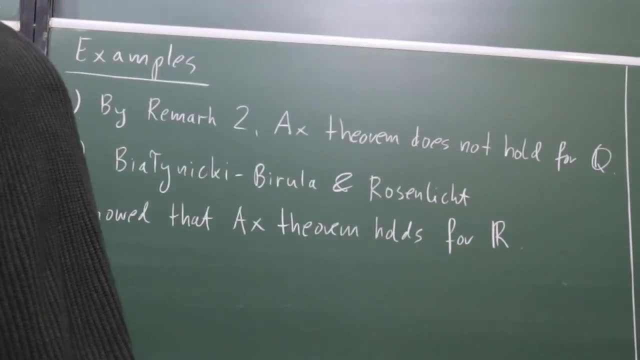 universal algebra and then he moved to universal algebra and then he moved to algebraic geometry, i think. or he was algebraic geometry, i think, or he was algebraic geometry, i think, or he was interesting in more topics before, interesting in more topics before, interesting in more topics before, but anyway he. 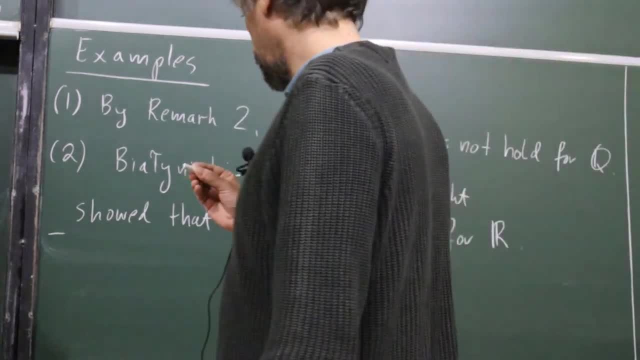 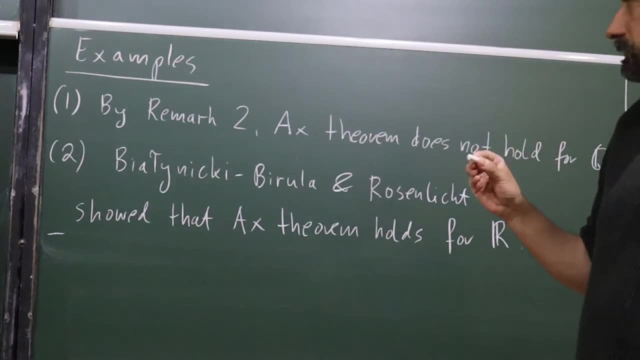 but anyway, he, but anyway. he unfortunately passed away at the age of 85. unfortunately passed away at the age of 85. unfortunately passed away at the age of 85 on monday, on monday, on monday, uh, uh, uh, okay. so now okay, so now okay. so now let's start proving access theorem. 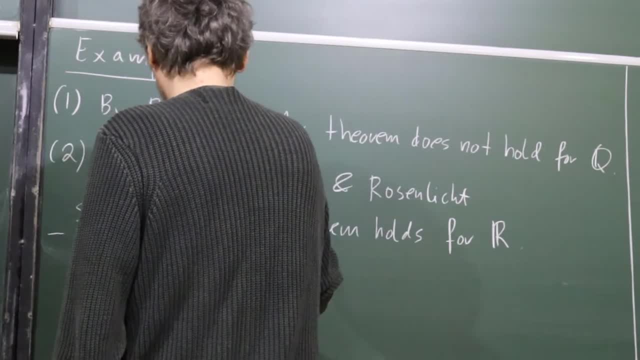 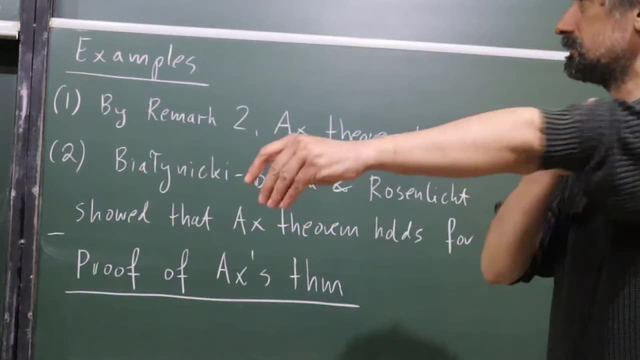 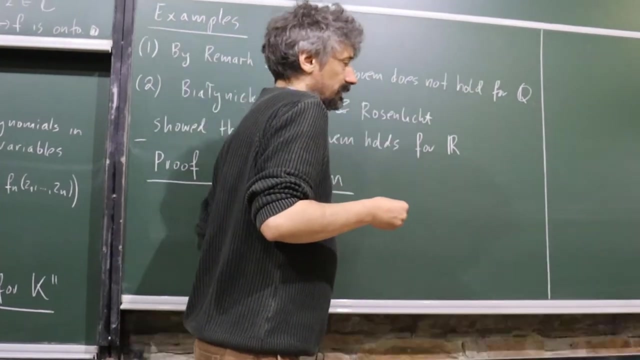 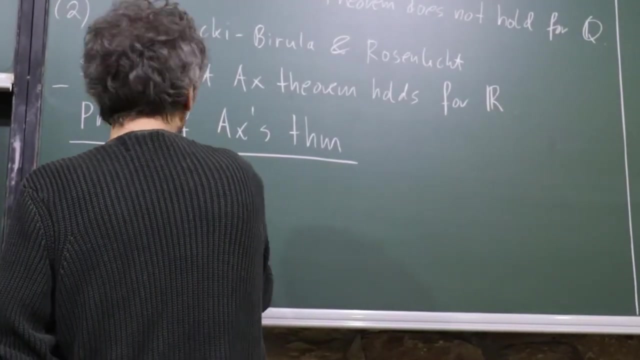 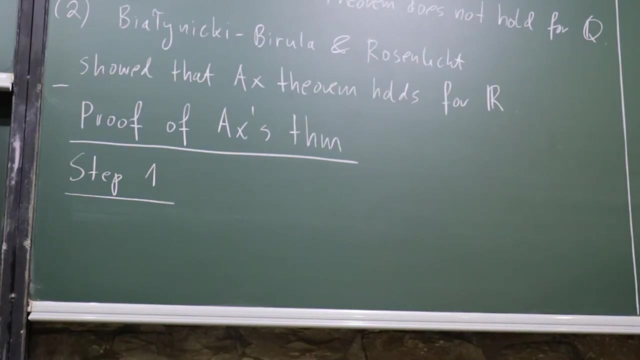 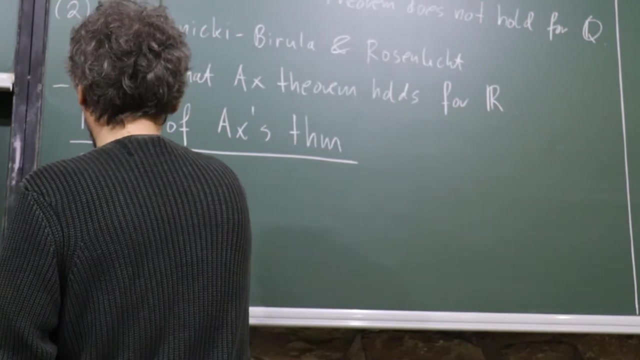 let's start proving access theorem. let's start proving access theorem. it will be in three steps. it will be in three steps. it will be in three steps. okay, step one. so so so, step one that access theorem. step one that access theorem. step one that access theorem. 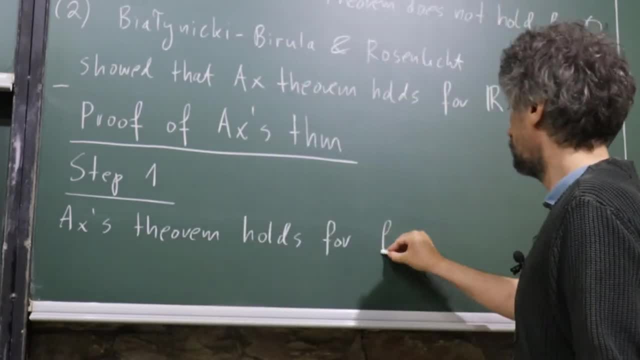 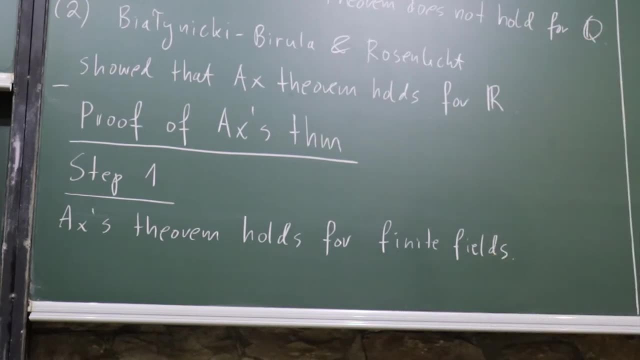 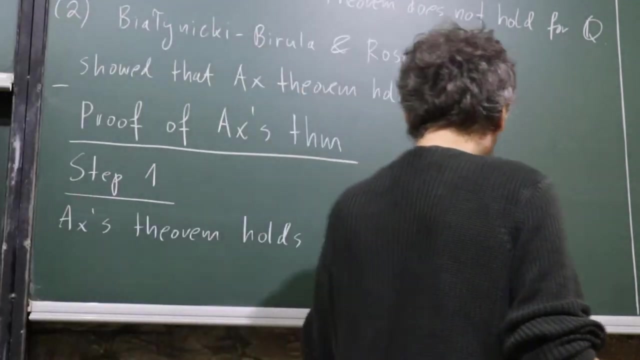 holds for finite fields, and actually that's the main reason, and actually that's the main reason, and actually that's the main reason, which is quite obvious, which is quite obvious, which is quite obvious, okay, okay, okay. so actually we use this and after that. so actually we use this and after that. 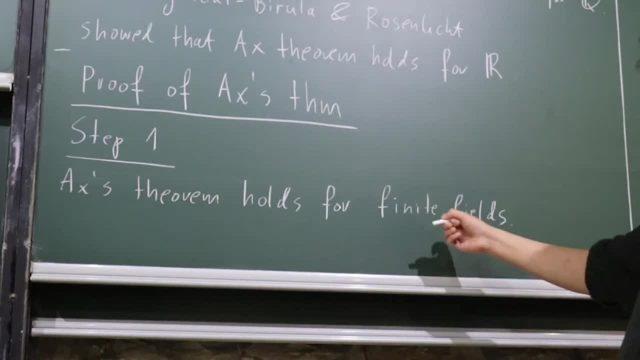 so actually we use this and after that there will be two more steps which will. there will be two more steps which will. there will be two more steps which will be kind of be kind of be kind of formal manipulations, but one can say formal manipulations, but one can say: 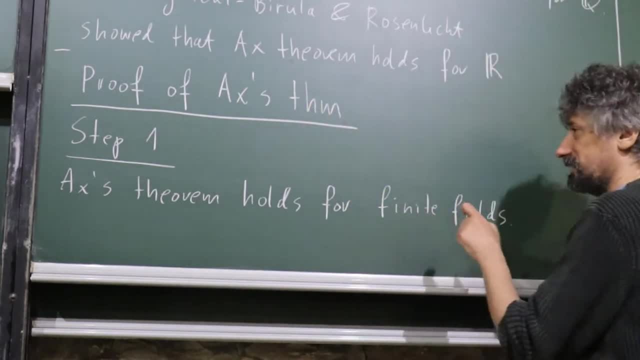 formal manipulations, but one can say: that's, that's, that's somehow, somehow, somehow. it's a very strange thing that it's a very strange thing that it's a very strange thing that this is a kind of statement. this is a kind of statement, this is a kind of statement that if we show first it holds for. 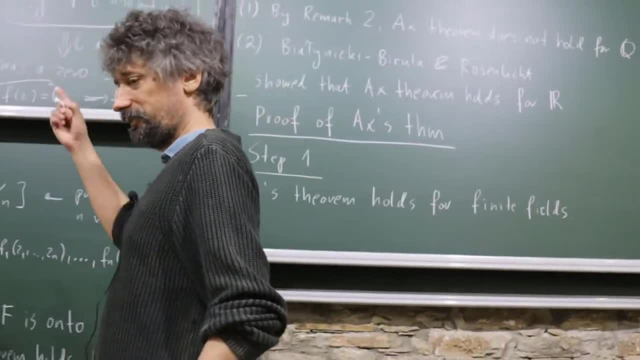 that if we show first it holds for that, if we show first it holds for finite fields, finite fields, finite fields, then we can conclude from that it it also. then we can conclude from that it it also. then we can conclude from that it it also holds for this very infinite fields of. 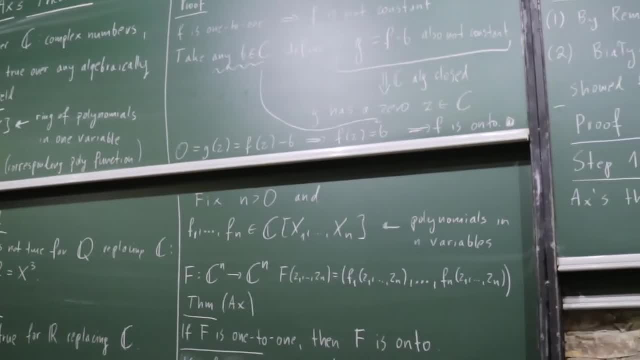 holds for this very infinite fields of holds for this very infinite fields of complex numbers, complex numbers, complex numbers, and you will see how, and you will see how, and you will see how. and i think sir has a paper about more and i think sir has a paper about more. 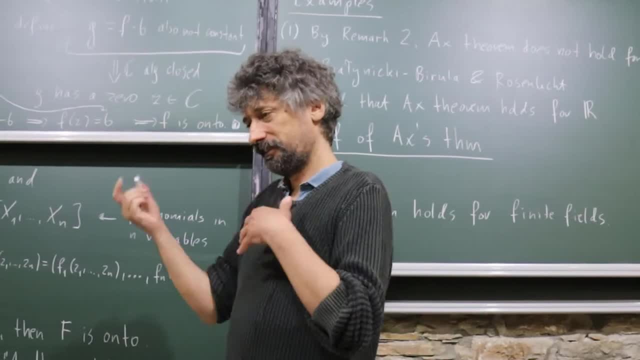 and i think sir has a paper about more statements like this, statements like this, statements like this. the title is something like how to. the title is something like how to. the title is something like how to prove theorems about infinite fields. prove theorems about infinite fields. 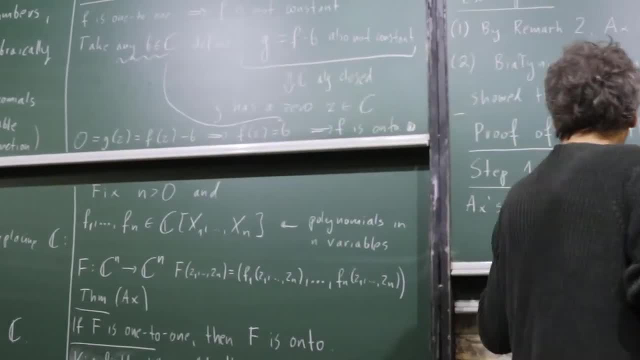 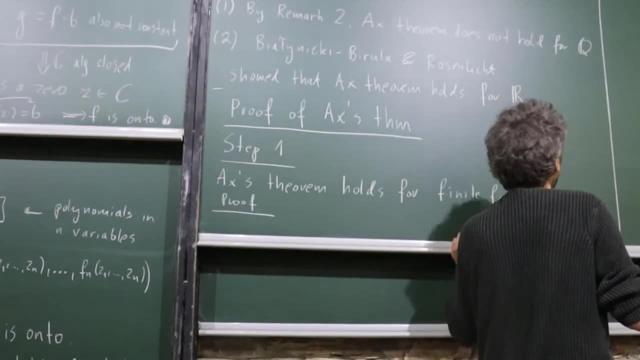 prove theorems about infinite fields using finite fields. and he also gives using finite fields and he also gives using finite fields, and he also gives this example, this example, this example proof, proof, proof of step one. so this is quite clear for any finite. so this is quite clear for any finite. 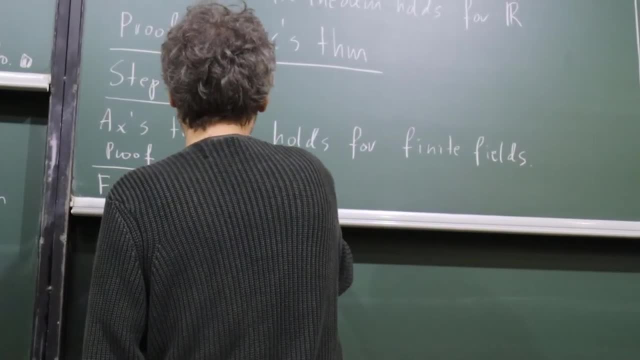 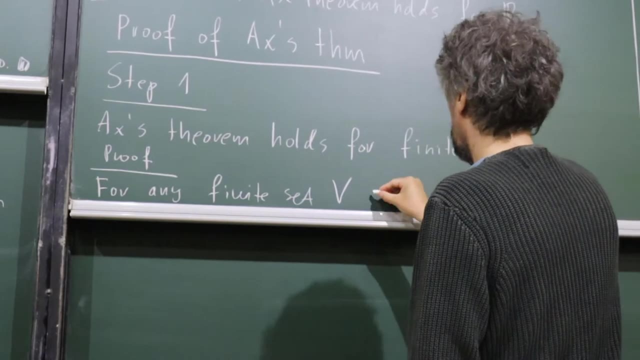 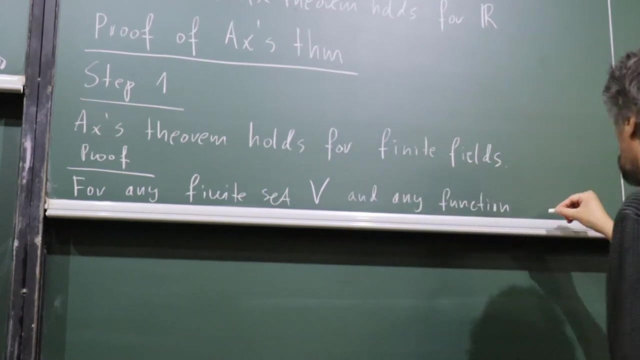 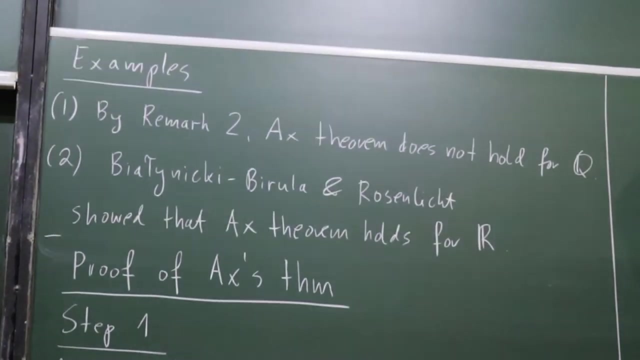 so this is quite clear: for any finite set, for any finite set v, for any finite set v, for any finite set v, and and and, any function, let's say denoted, let's say denoted, let's say denoted. the same way, i hope we all know very well that even 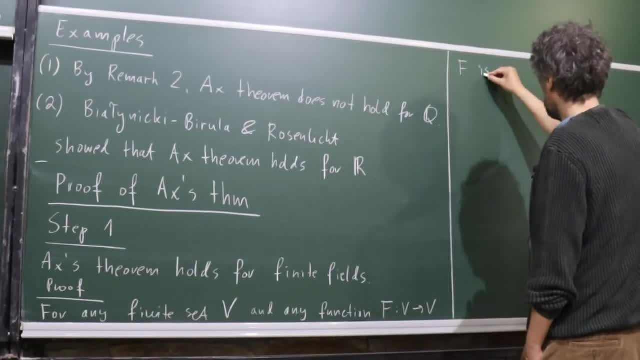 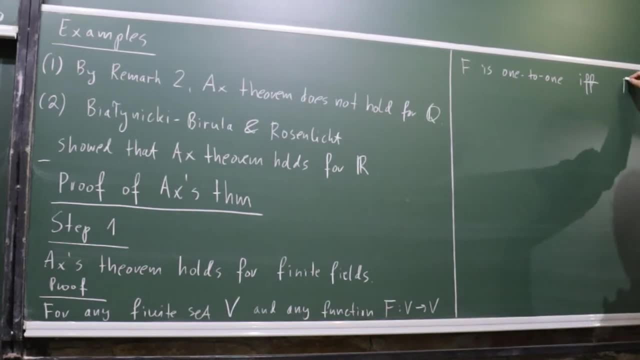 i hope we all know very well that even i hope we all know very well that even equivalence is true, equivalence is true, equivalence is true. so f is one to one, f is onto even, even only f is onto even, even only f is onto even, even only. but this other implication somehow does. 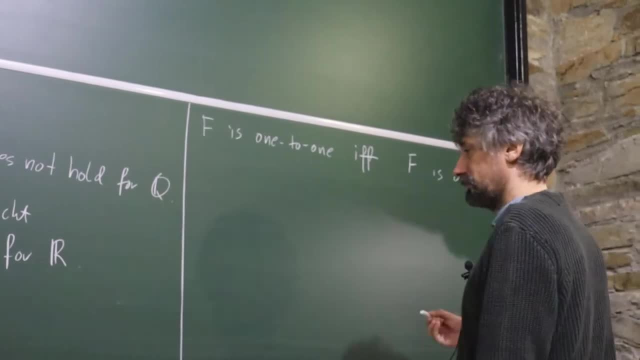 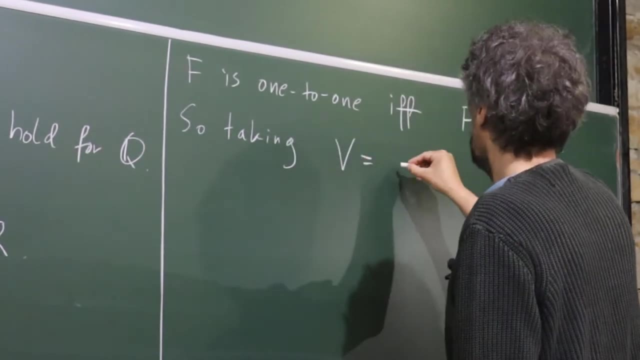 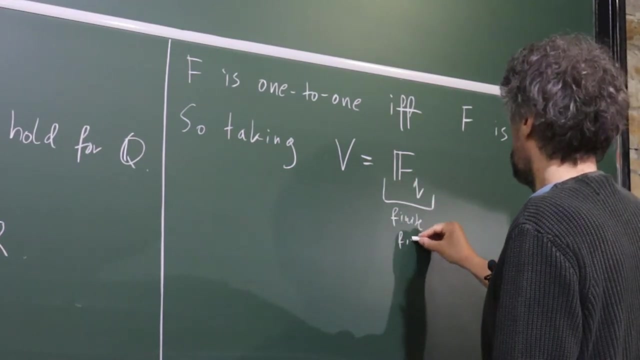 but this other implication somehow does, but this other implication somehow does not transfer to infinite fields. not transfer to infinite fields, not transfer to infinite fields. so, taking v, taking v, taking v, equal, equal, equal, some fq, some fq, some fq, this is a finite field. this is a finite field. 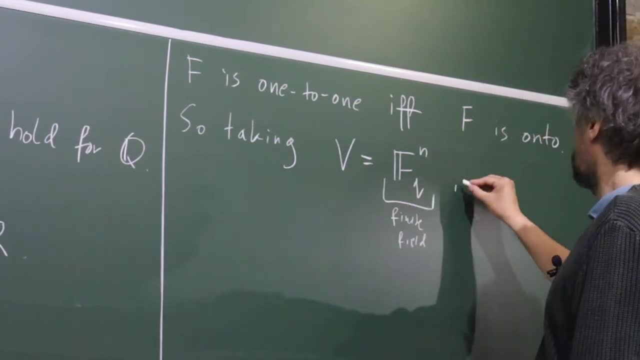 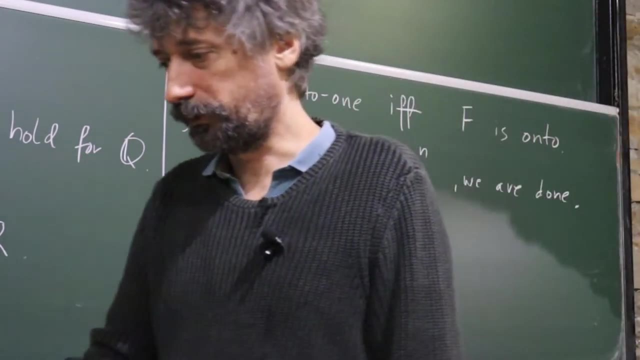 this is a finite field to n. we are done. we are done. we are done. in particular, if it's one to one, it's on to. in particular, if it's one to one, it's on to. we are done. in particular, if it's one to one, it's on to any function. 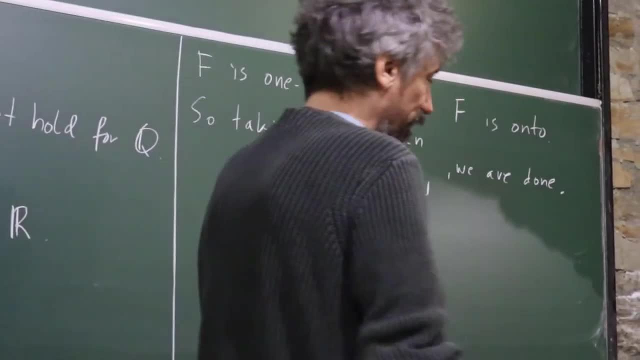 any function, any function, but also any function, but also any function, but also any function on fields is a polynomial function, so on fields is a polynomial function, so on fields is a polynomial function. so any function is not a great generality, any function is not a great generality. 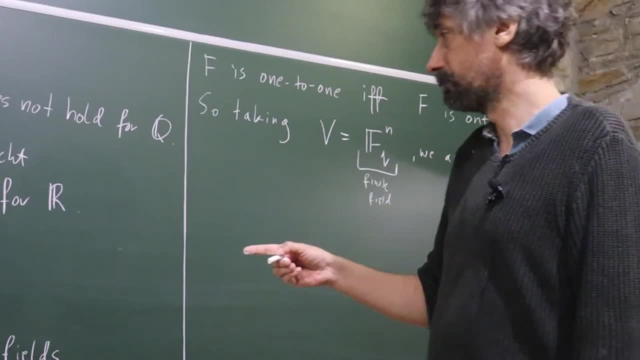 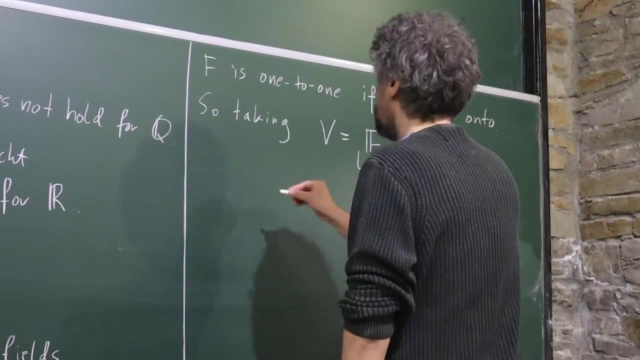 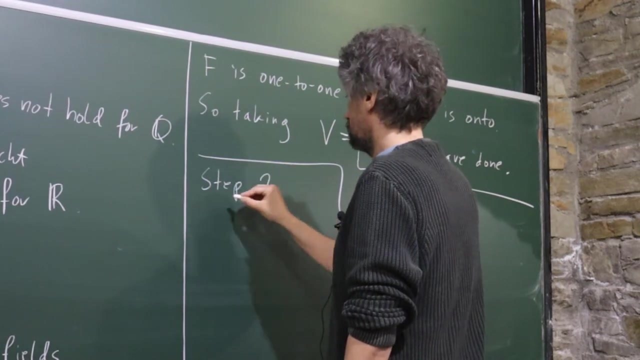 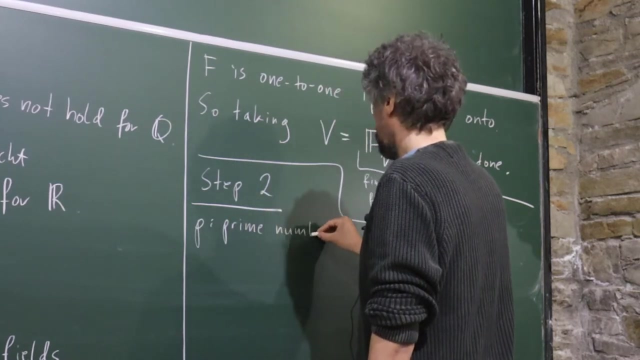 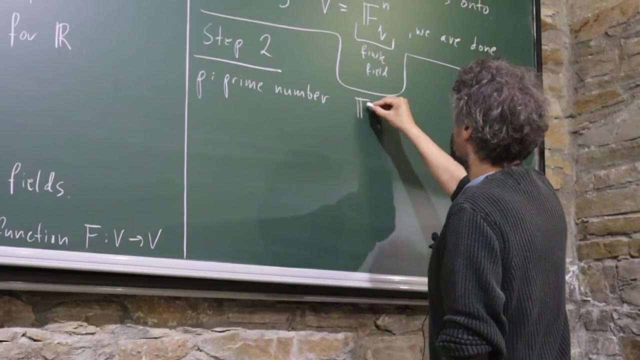 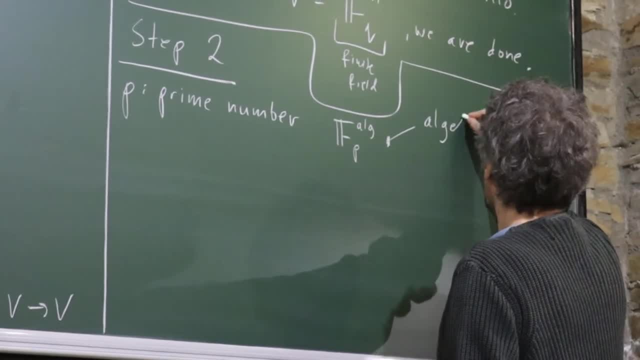 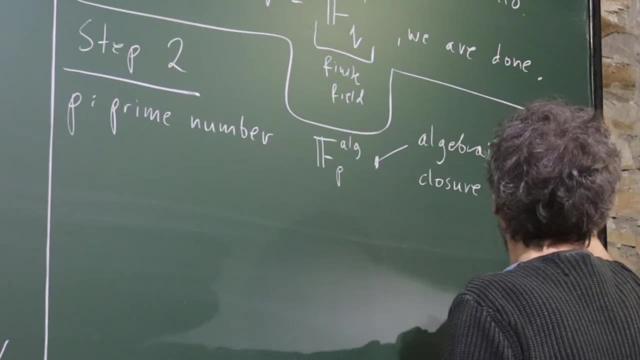 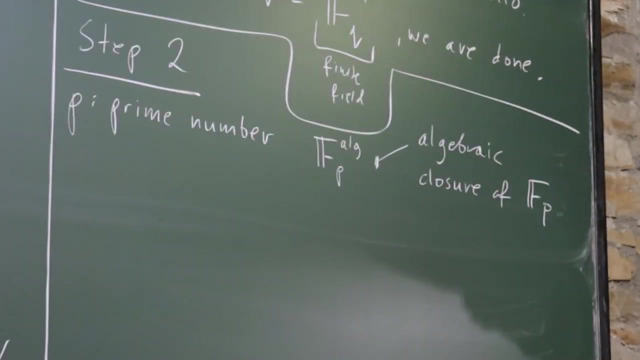 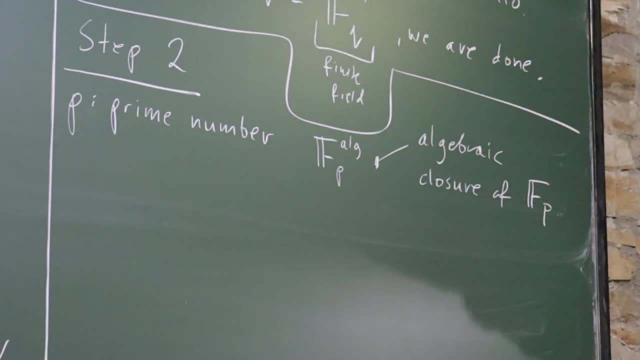 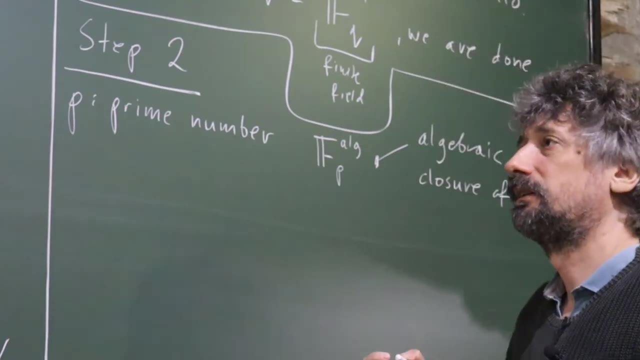 maybe most of you have now a course in. maybe most of you have now a course in galva theory, actually galva theory, actually galva theory, actually. okay, yes, so it's the smallest. yes, so it's the smallest. yes, so it's the smallest, smallest algebraic close field containing: 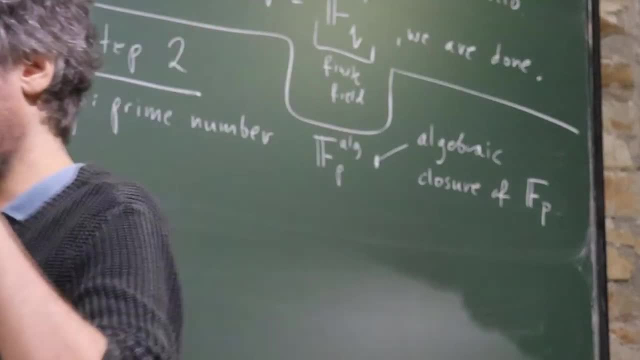 smallest algebraic close field, containing smallest algebraic close field, containing this field of p elements. so it's a union, this field of p elements. so it's a union, this field of p elements. so it's a union of all finite extensions of fp, of all finite extensions of fp. 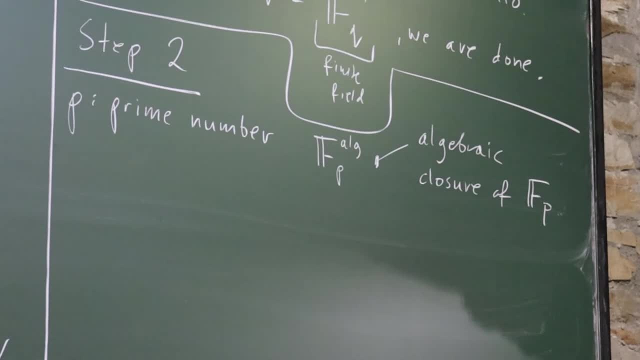 of all finite extensions of fp. so, in other words, so, in other words, so, in other words, it's a union, it's a union, it's a union of all finite fields of characteristic p, of all finite fields of characteristic p, of all finite fields of characteristic p which we will use. okay, but i hadn't. 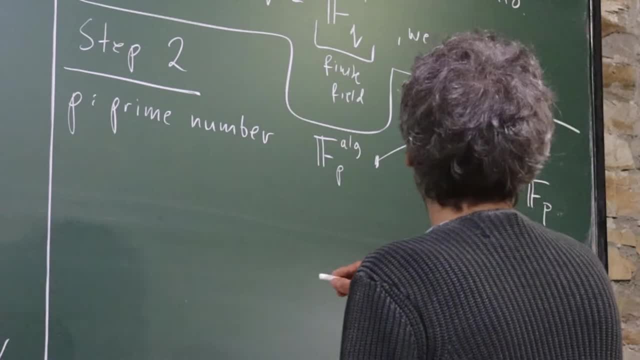 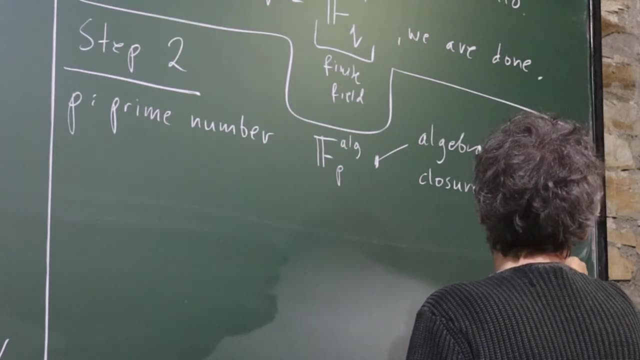 which we will use, okay, but i hadn't, which we will use okay, but i hadn't finished the statement, finished the statement, finished the statement then, then, then, so this is of course field, so this is of course field, so this is of course field of p elements. 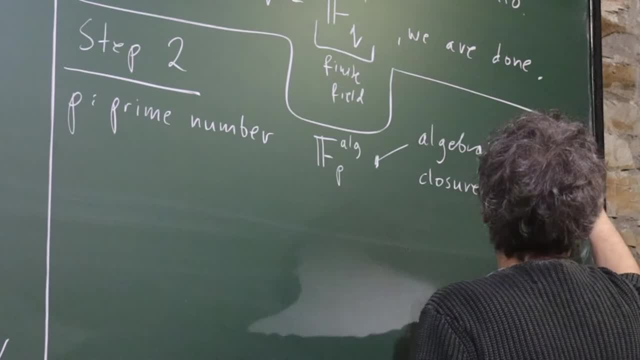 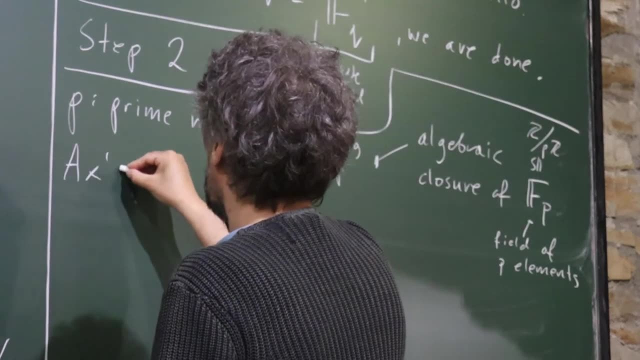 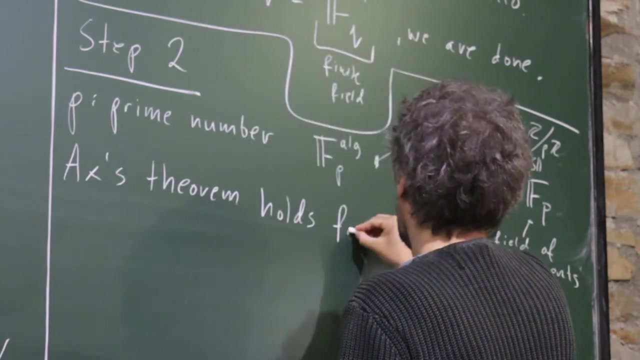 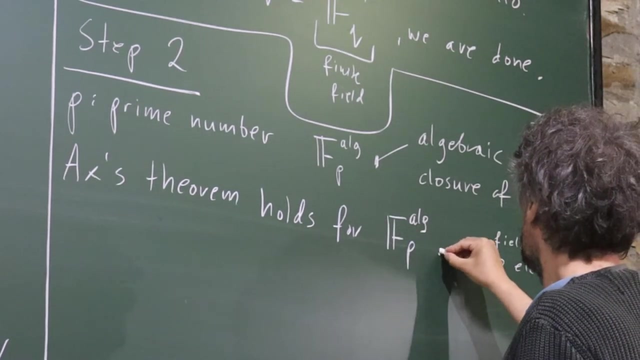 which is the same, which is the same, which is the same, instead of lpz, then, then, then, access, access, access, access theorem holds for this field, which is now infinite. so it's a union of finite fields, but of. so it's a union of finite fields, but of. 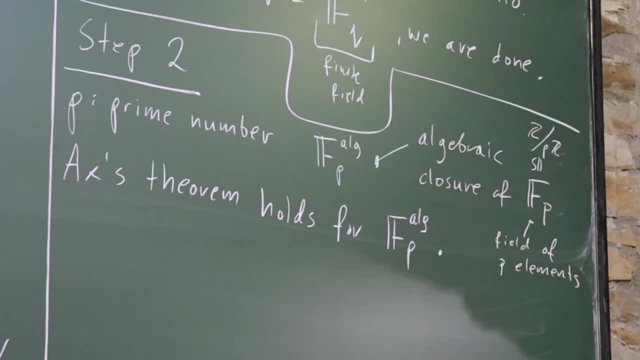 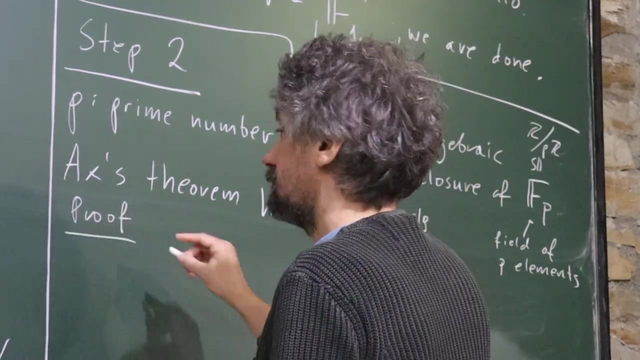 so it's a union of finite fields, but of course it's infinite, course, it's infinite, course it's infinite. each algebraic closed field must be, each algebraic closed field must be, each algebraic closed field must be infinite, infinite, infinite, infinite. so proof of this step: 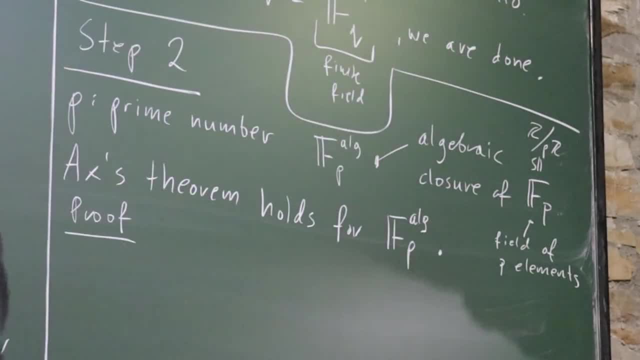 yes. so you can see we are getting kind of yes. so you can see we are getting kind of yes. so you can see we are getting kind of closer and closer to c in a way, closer and closer to c in a way, closer and closer to c in a way, first we have finite field, which is quite 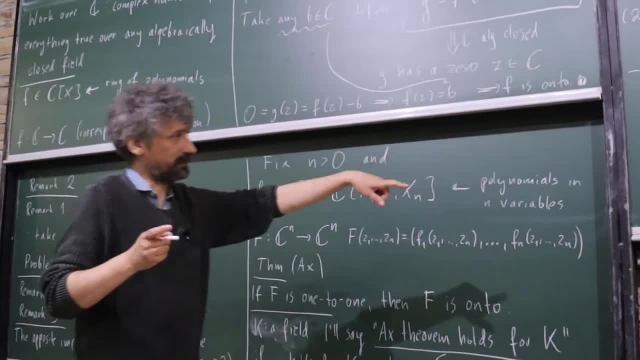 first we have finite field, which is quite. first. we have finite field which is quite far, far far conceptually from complex numbers, but conceptually from complex numbers, but conceptually from complex numbers. but now, now, now you get something looking a bit similar. you get something looking a bit similar. 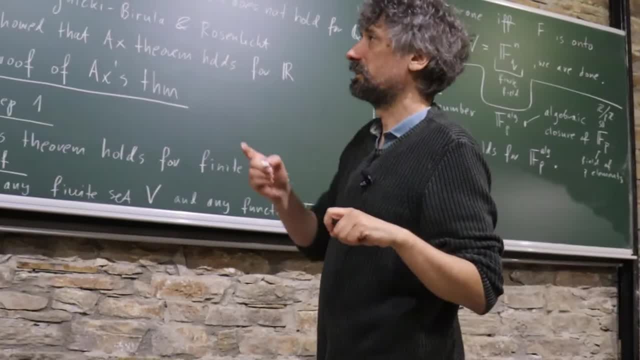 you get something looking a bit similar, because this one is also algebraically, because this one is also algebraically, because this one is also algebraically closed, closed, closed, like complex numbers, like complex numbers, like complex numbers, okay, okay, so i need you to, so i need you to. 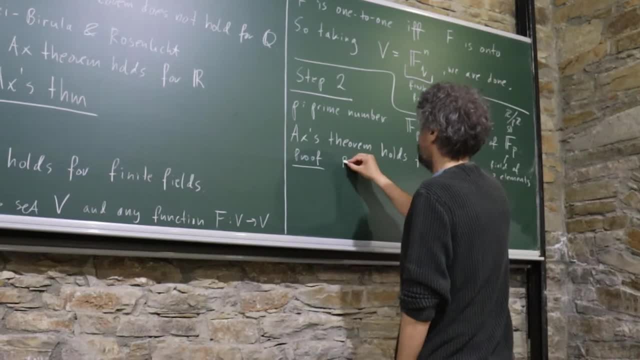 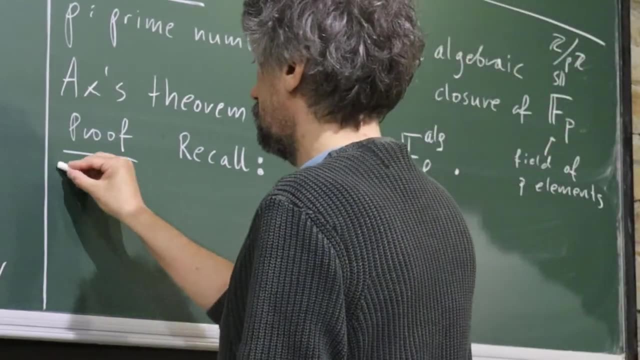 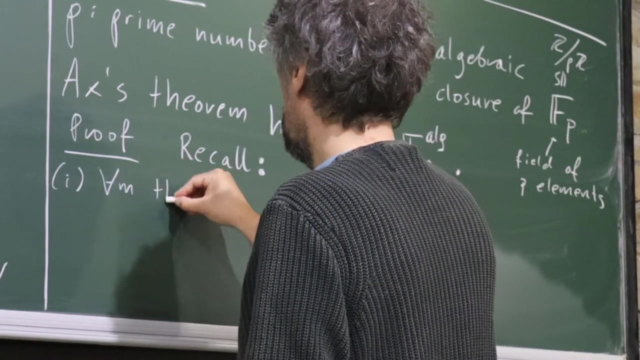 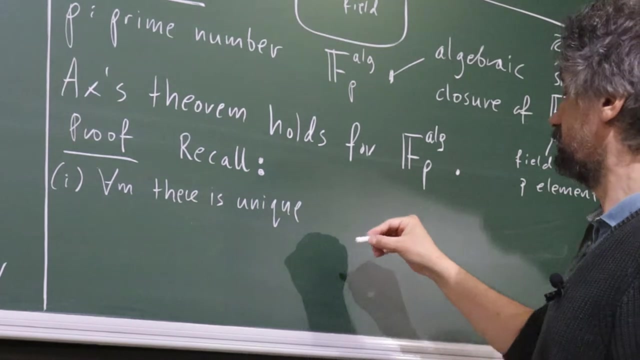 so i need you to recall some facts about finite fields. so first, so first, so first, okay for each m. probably you know it, but let me make. probably you know it, but let me make. probably you know it, but let me make sure, sure, sure, there is a unique. 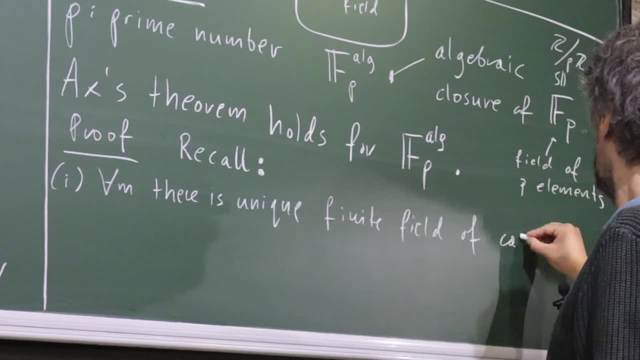 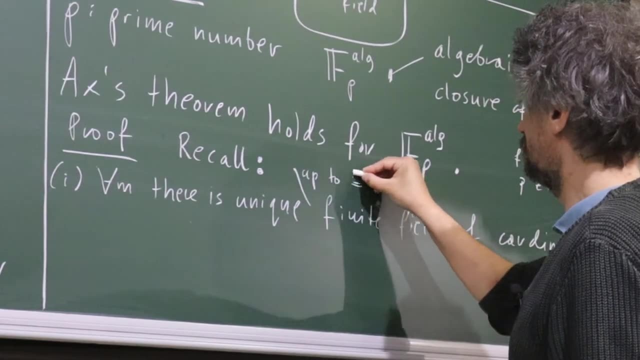 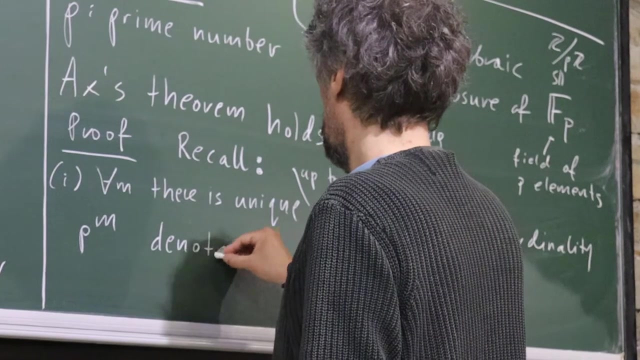 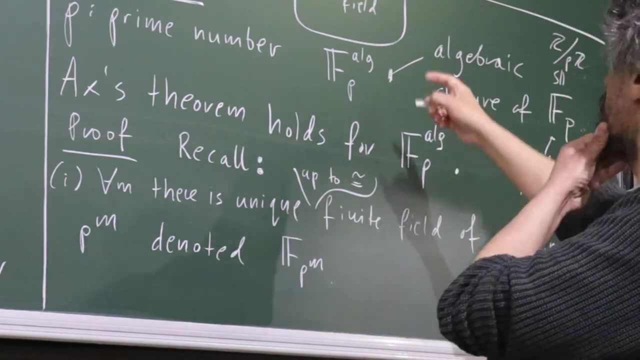 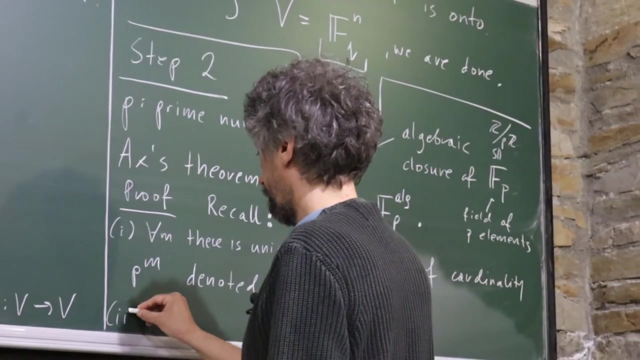 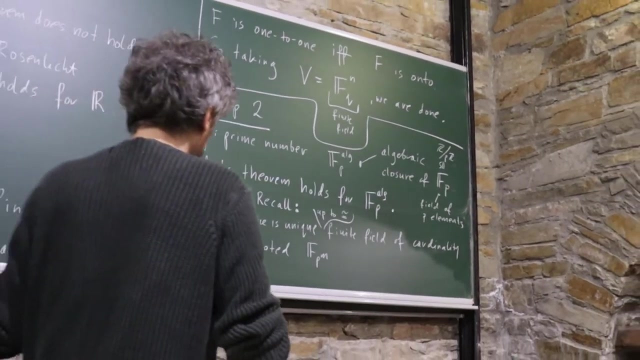 finite field. finite field field of cardinality unique up to isomorphism of cardinality, p to the m denoted fpm, which I already used, this notation here. okay, now the question is where, when two such fields embed into each other, so not always one, this exponent, one exponent, has to divide the other. 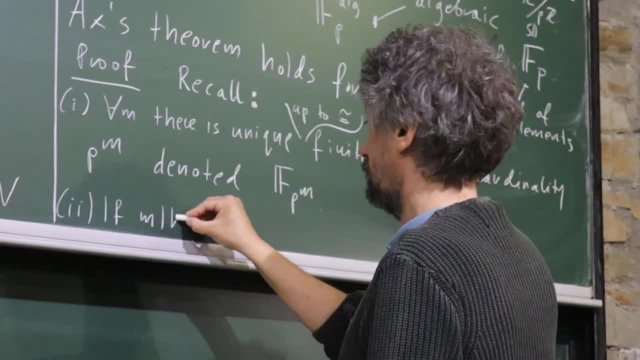 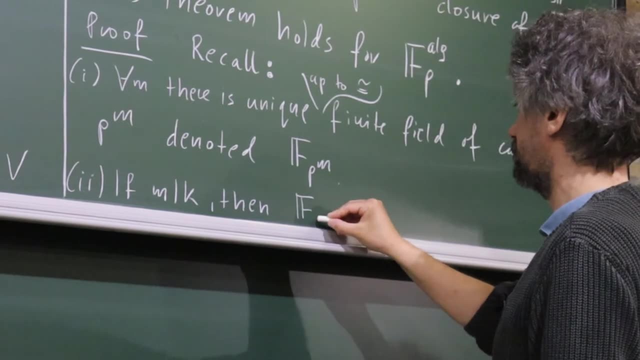 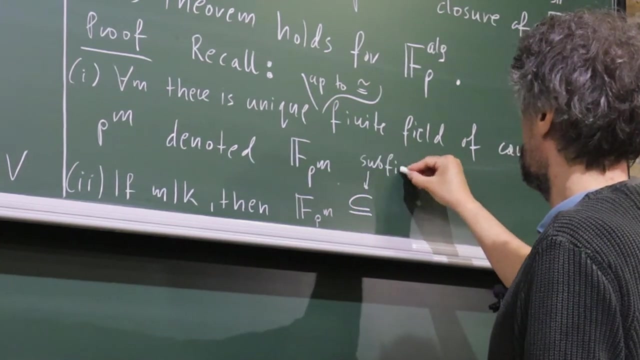 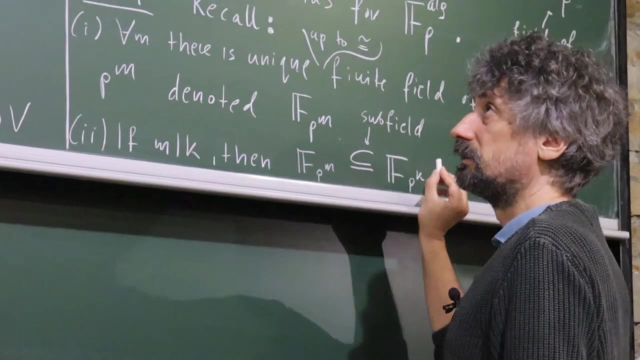 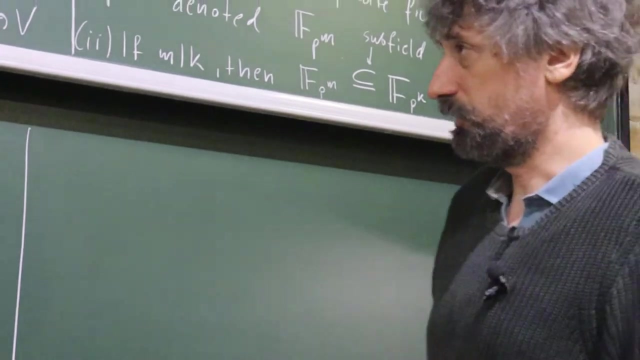 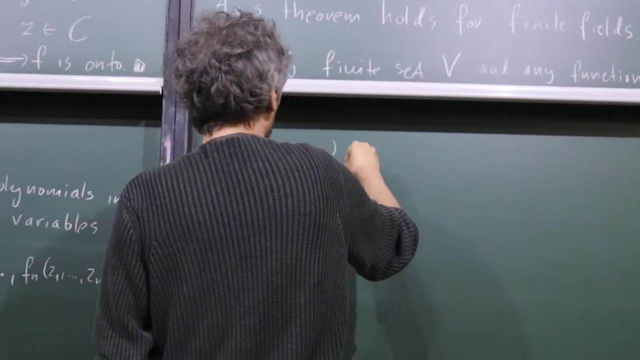 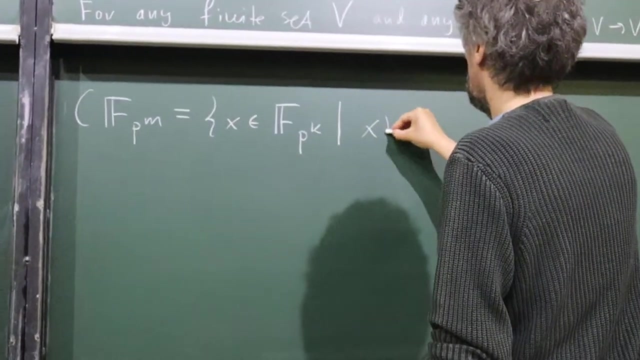 so if m divides k, then we can think that one of them is a subfield of the other, and you can write it explicitly. so, actually, if you want to know how exactly exactly, then these are those elements from fpk, such that X to power, p is X. 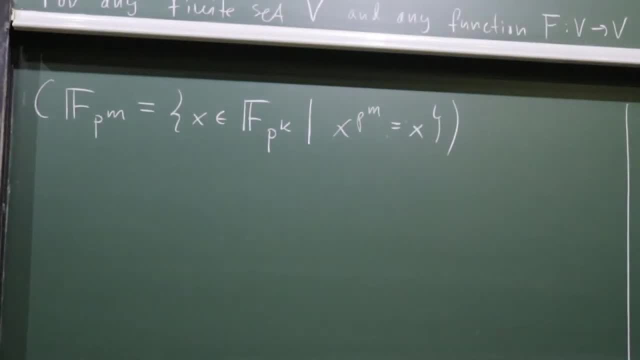 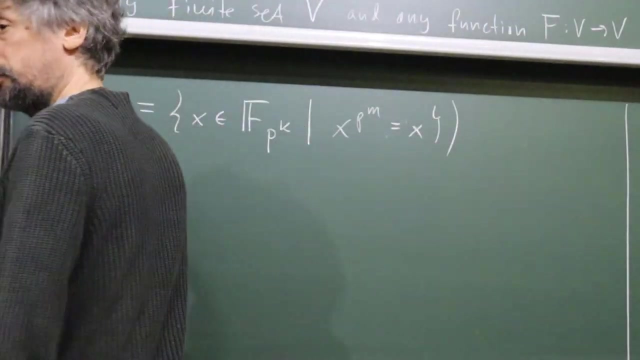 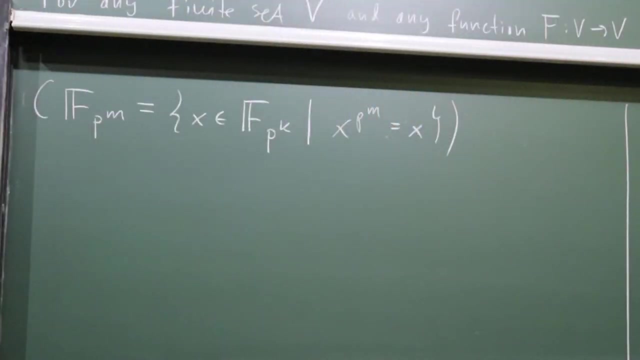 so splitting field of this x PM to minus X polynomial. okay, so this is how one finite field is embed into another: k, huh, k kan. a one plus a eight, multiplied by a APA, by a m divides k. so it's often confusing. so, for example, f4 does not embed into f8. 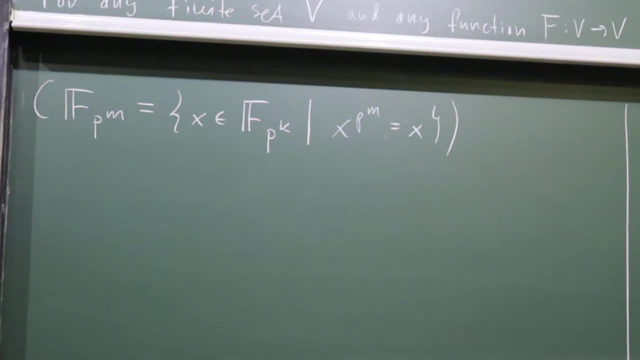 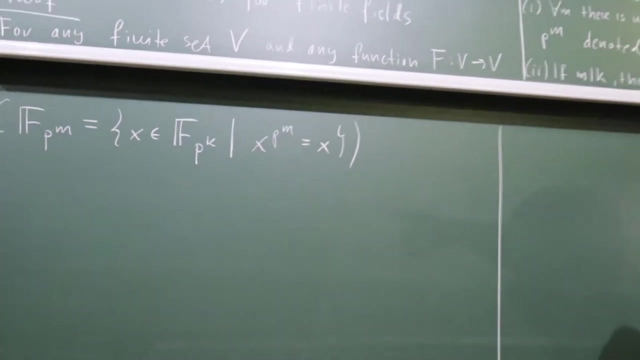 because 2 does not divide 3, but 4 divides 8, but 2 does not divide 3. i mean, i guess every year i'm at least once confused about it. but so this is, this is like a divisibility relation, like they are included in each other. 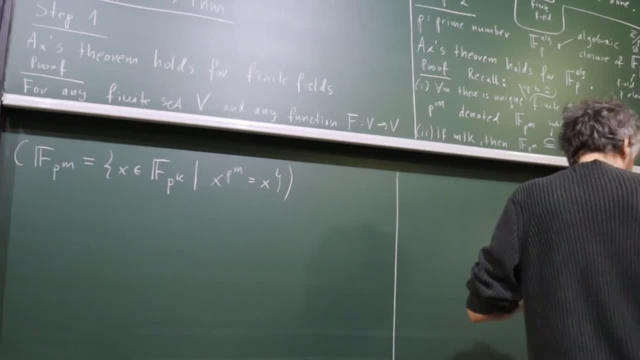 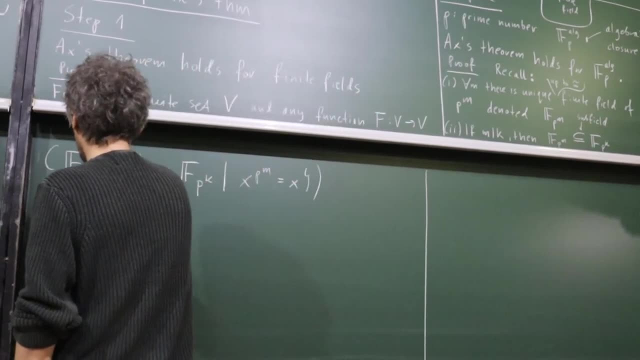 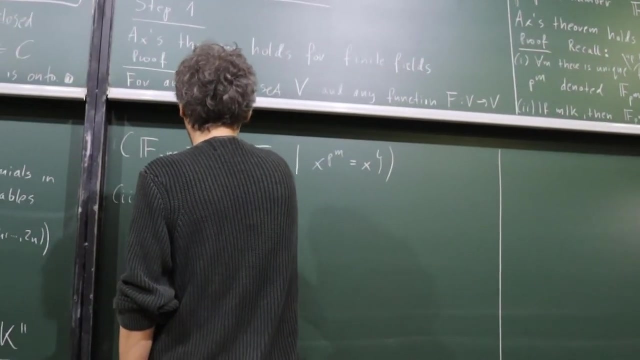 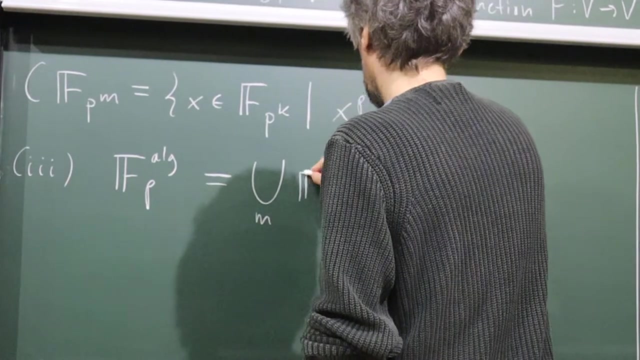 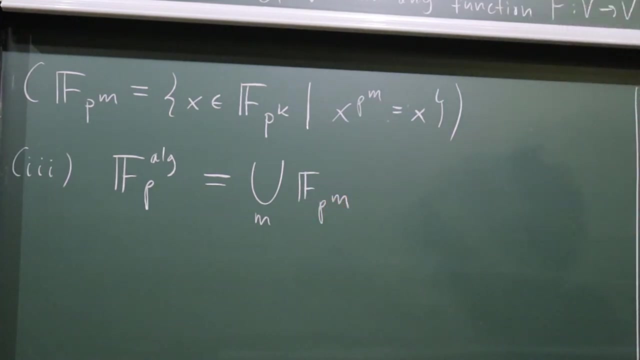 okay, and then we can. if we understand that, then we can kind of understand what is fp arch. so, as i said, fp arch is the union one can say of all this fpm. but then we have to understand in what sense it's a union, so how one is included into another. 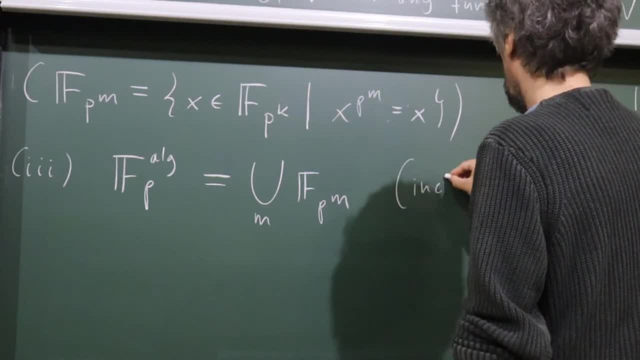 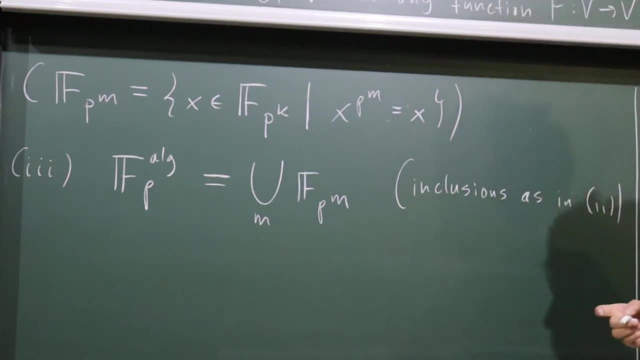 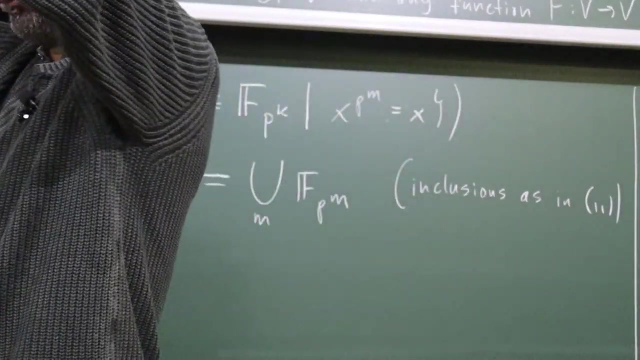 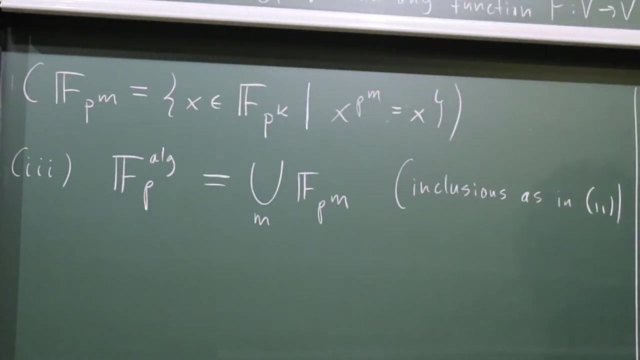 so in this way. so inclusions, as in part two. so it's not an increasing union. it's like this divisibility relation: every two finite fields are embedded into another one. but it's not true that it's an increasing union. but we can make it increasing union, which will be convenient. 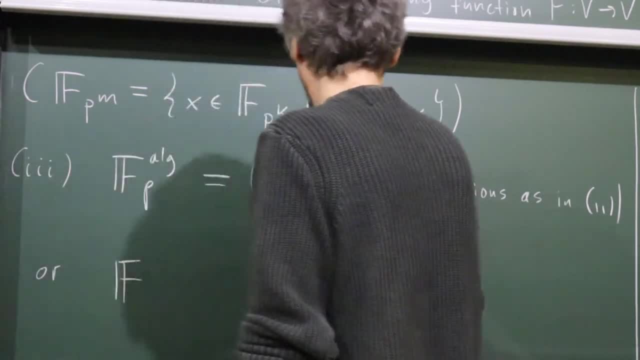 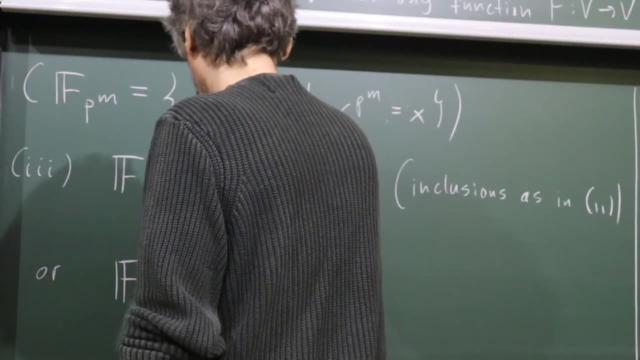 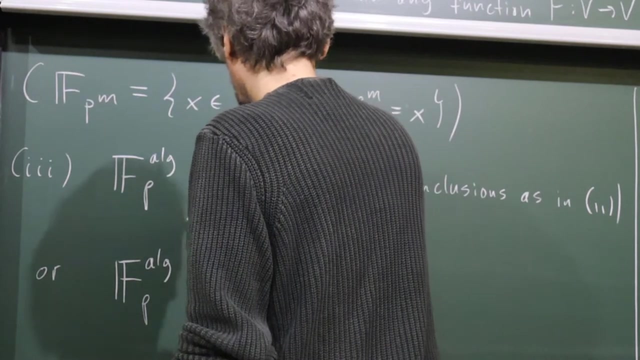 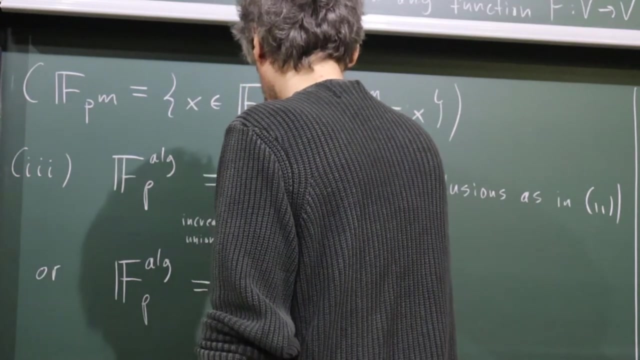 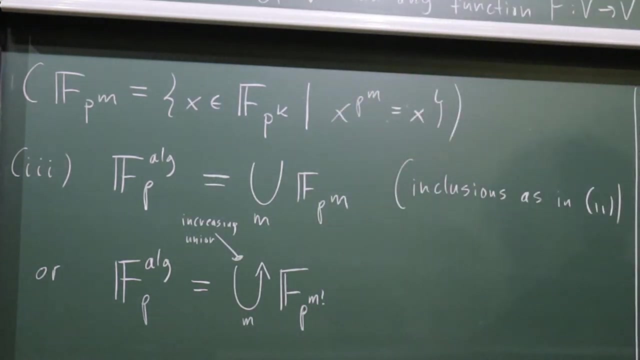 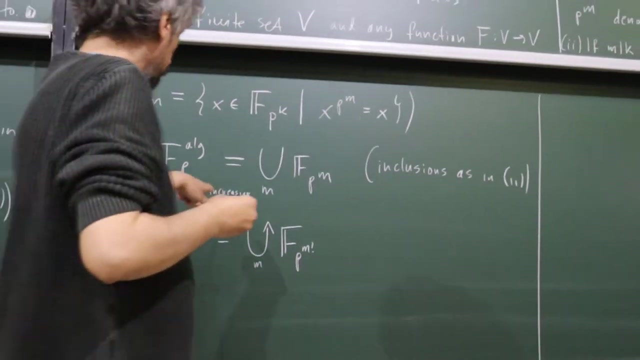 just if we take bigger and bigger numbers which divide each other. so if we take factorials, okay, these things revolve around this data. now this denotes increasing union. yes, because of course m factorial divides m plus one factorial. so now i made it in such a way: it is increasing union. 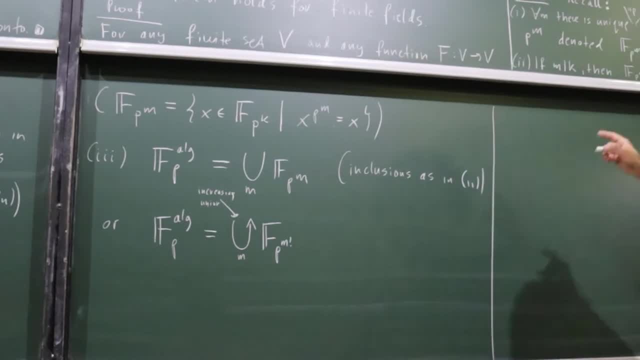 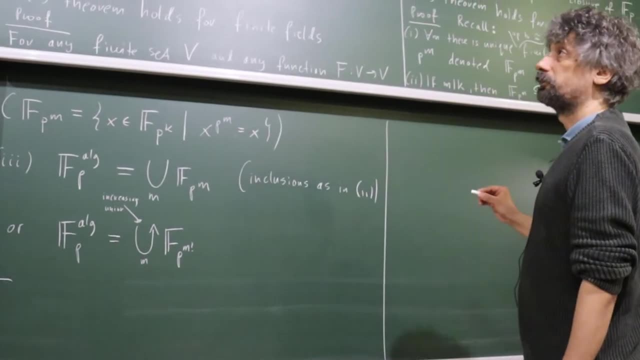 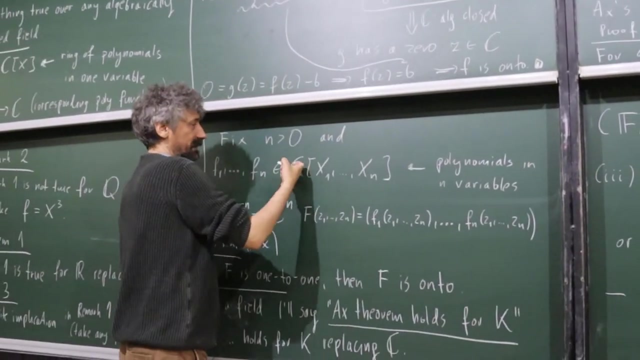 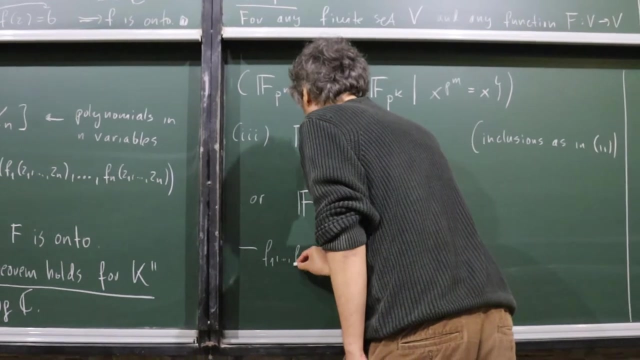 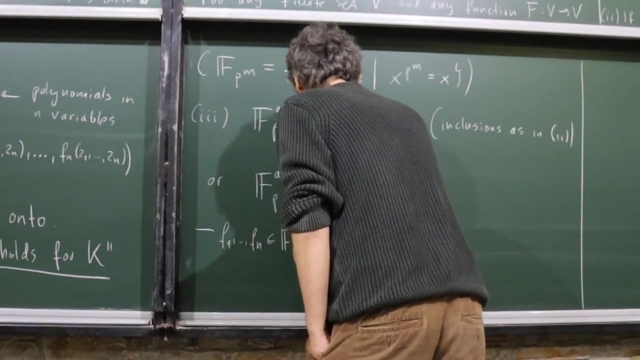 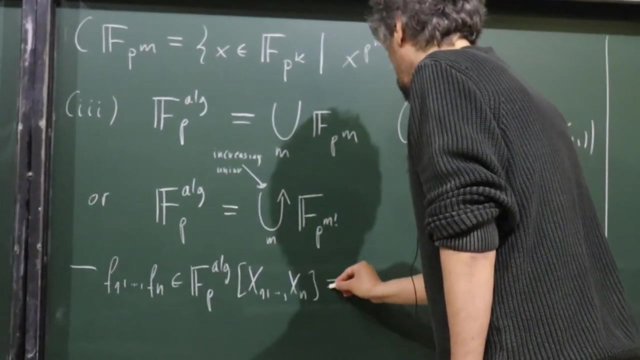 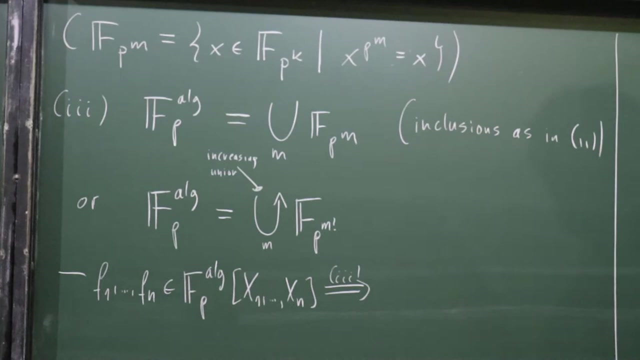 just by skipping some fields, things I wanted you to recall. so now the actual argument starts. okay, so we are proving this x, so we have this polynomials f1 fn in f, the arch x1, xn by because of this. yes, so they have all these n polynomials. they have 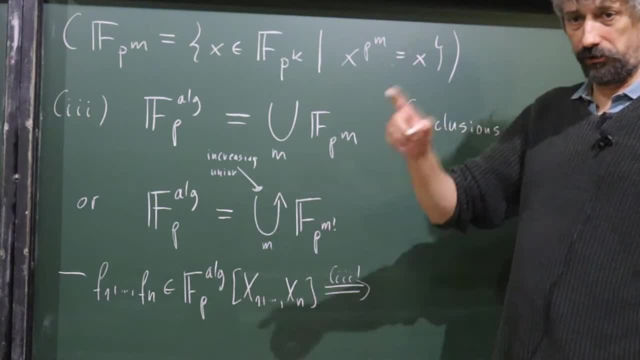 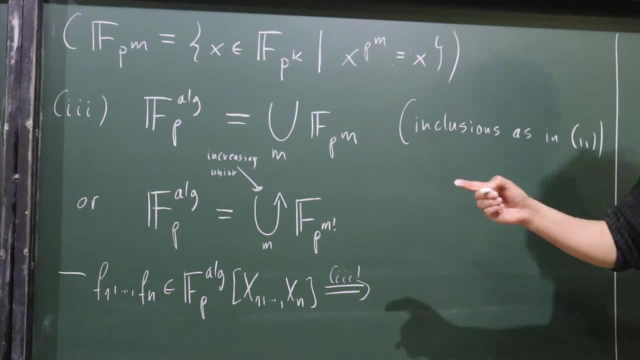 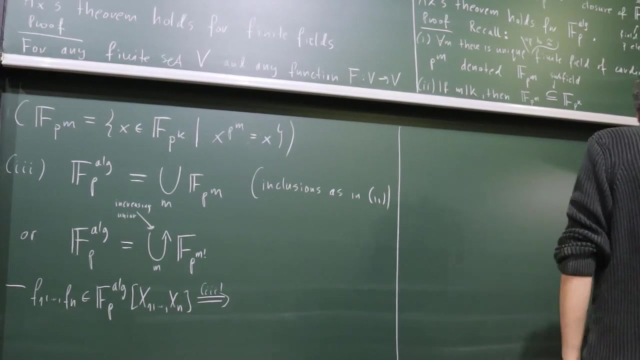 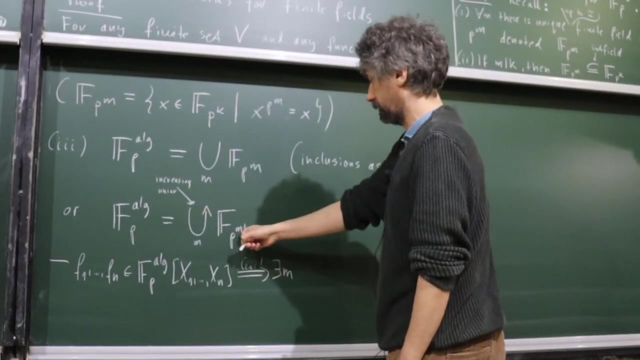 coefficients which live in this increasing union. so there are finitely many polynomials. together they have finitely many coefficients, so they must live on some finite level. so there is some, so there is some m, such that they all go to this fpm factorial. 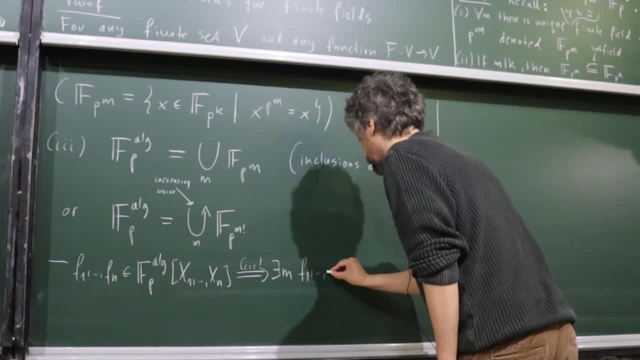 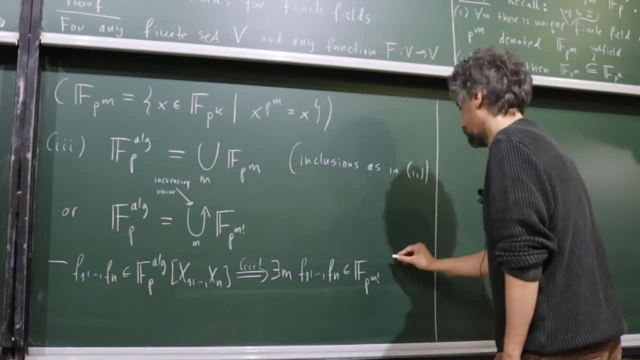 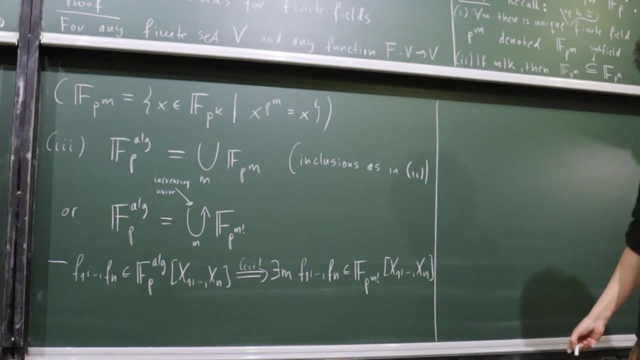 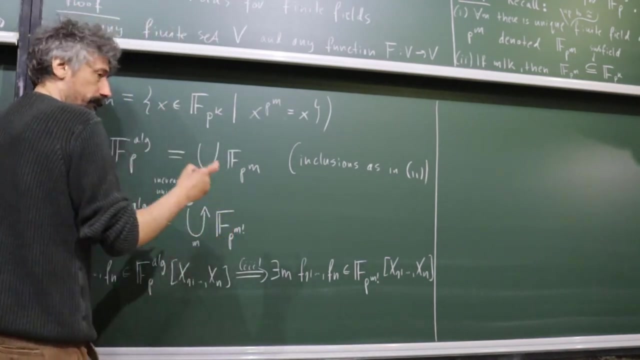 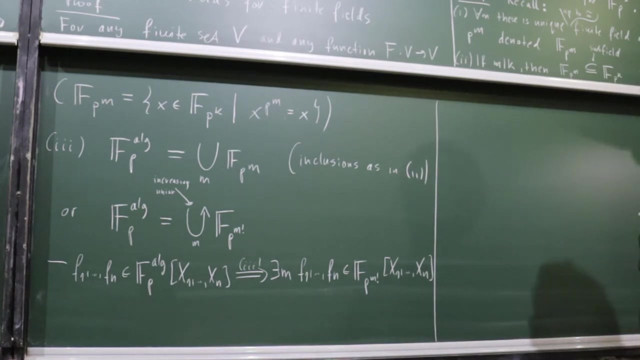 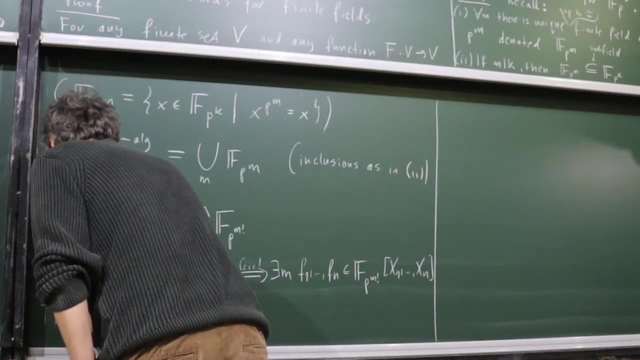 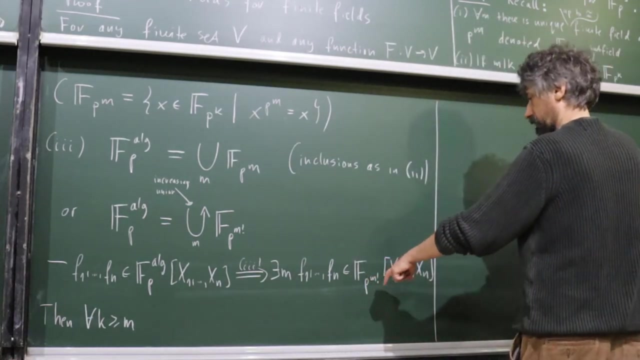 okay, all the coefficients I can find on some finite level, just picking questions, just picking questions one by one and waiting where they finally, all of them, fall into one of this finite fields. so then, also for all k later than m, since this field- fpk factorial- is bigger, they belong. 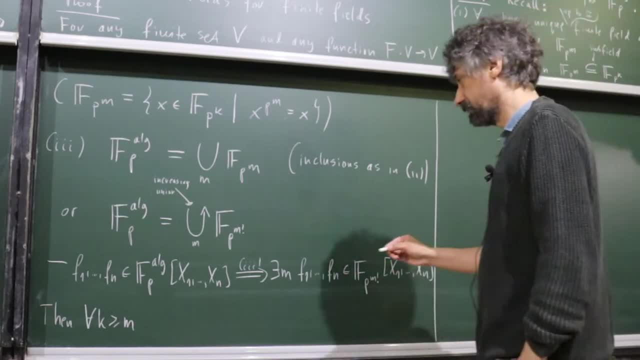 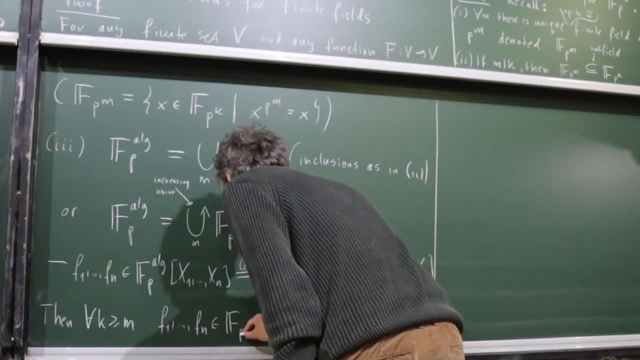 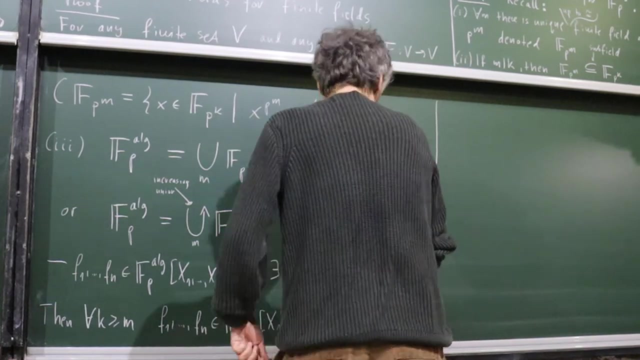 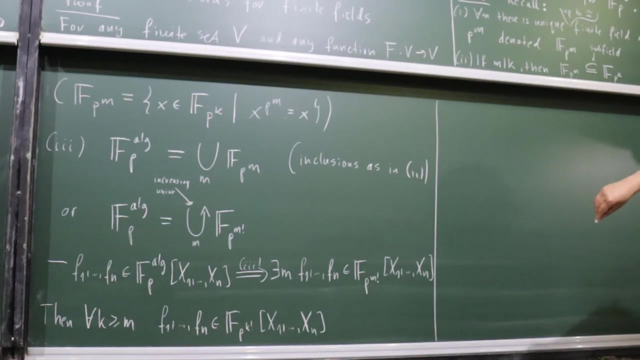 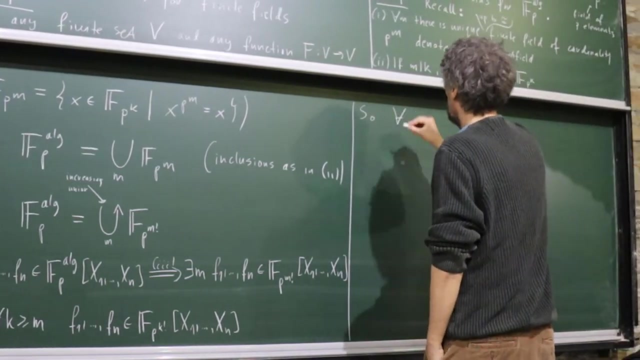 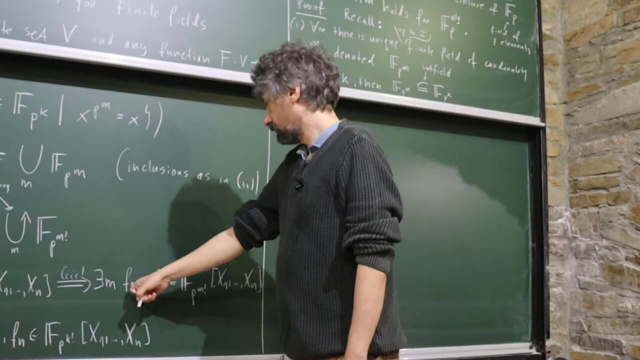 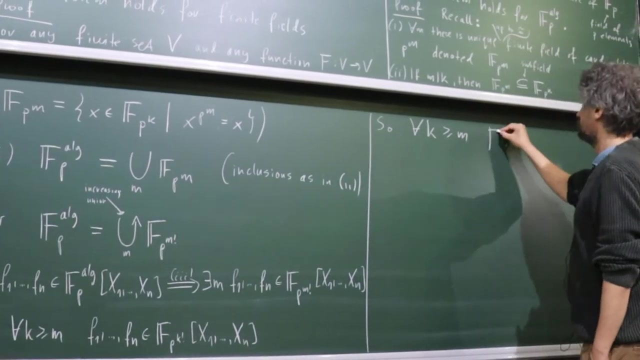 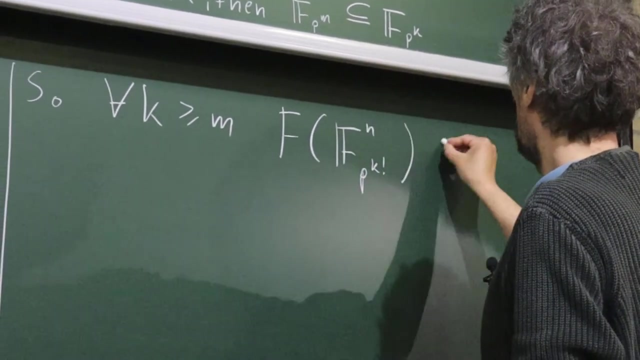 to the coefficients are also in the, also in the bigger field. but that means okay. but then the function F. so it means that for all k greater than n, yes, this function, they all have coefficients from this: F, p, k, factorial. so the function F takes this, the same field. 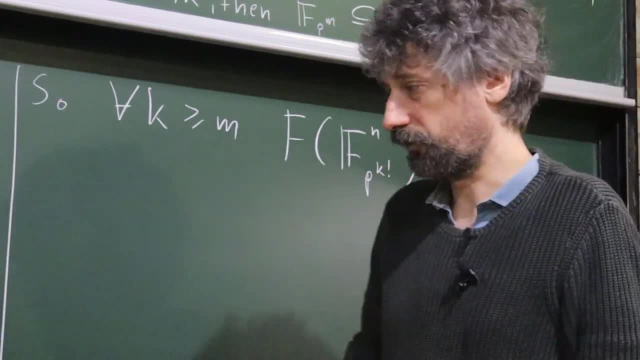 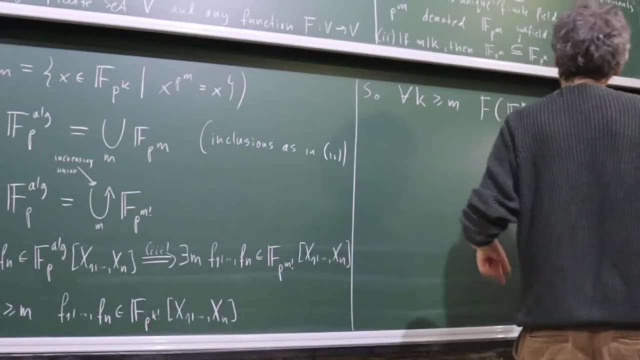 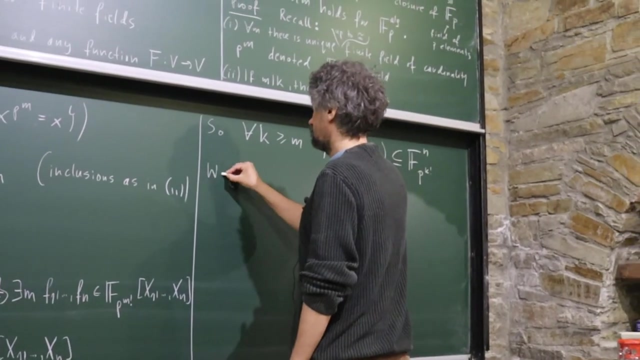 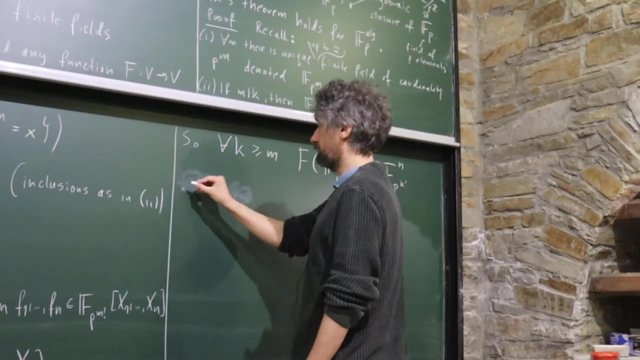 yes, because everything, everything, everything is the same, everything is the same, everything is happening always on the same, on the same field. for this chosen k, which is at least m, so we can. and, of course, since F is okay, let me write everything, since F is one to one. 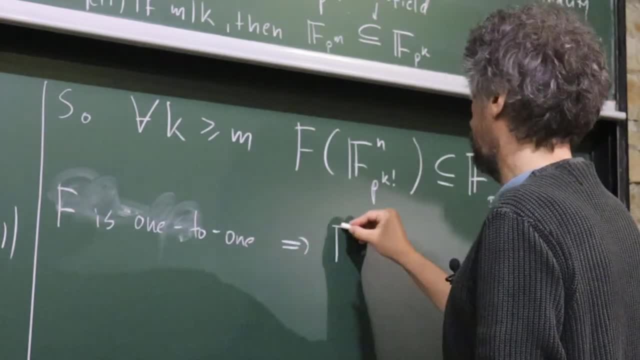 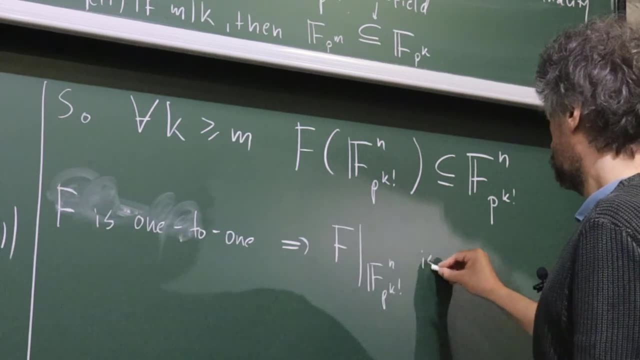 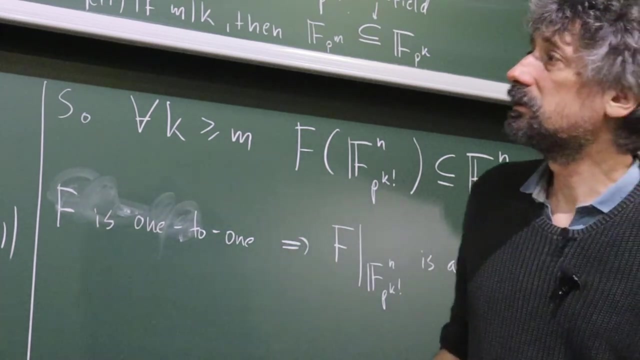 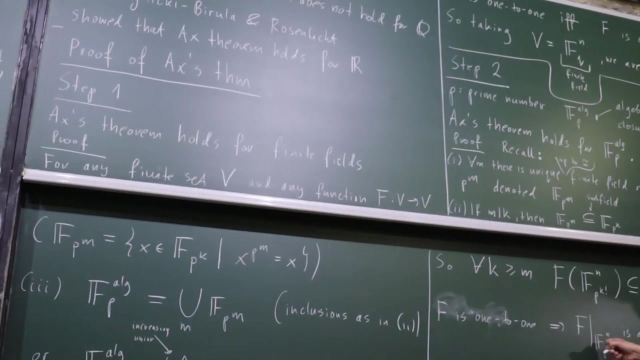 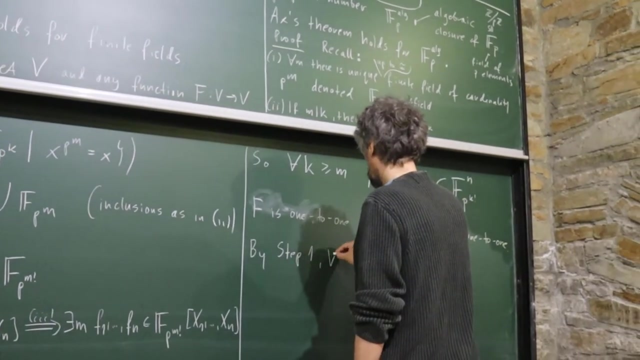 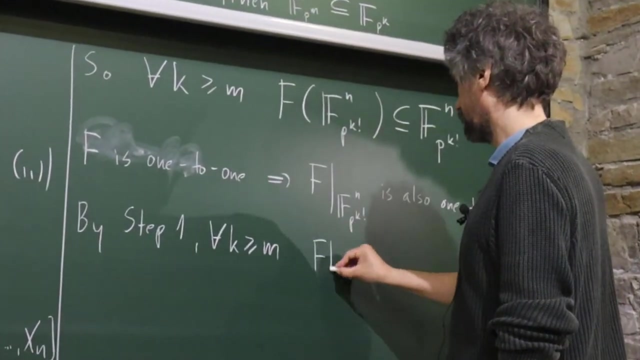 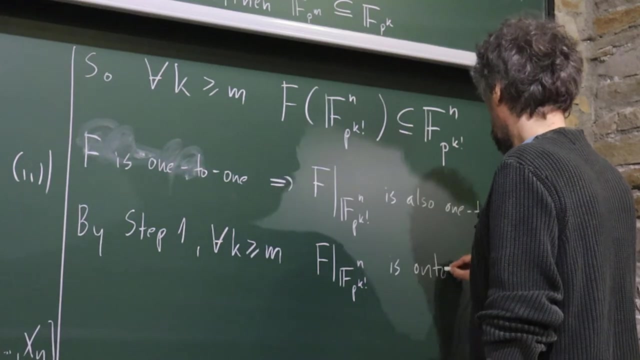 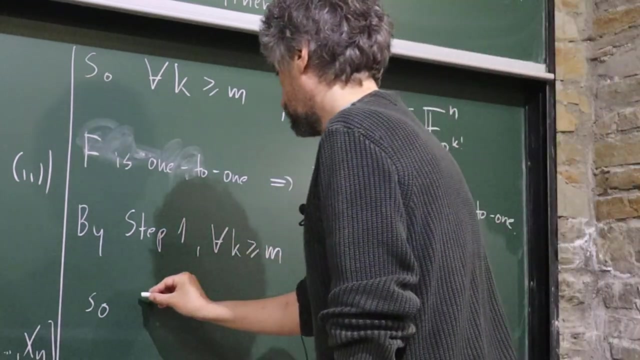 then F, restricted to this, it's also one to one, so we can apply step one to see that this function is onto for all k greater than m, this function, so two. so here we have actually equality, but there is a difference, although we have the first function. 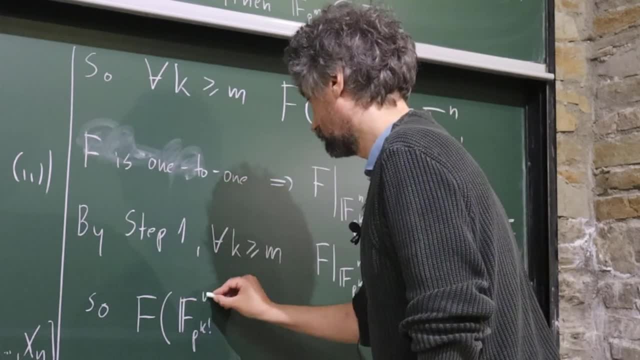 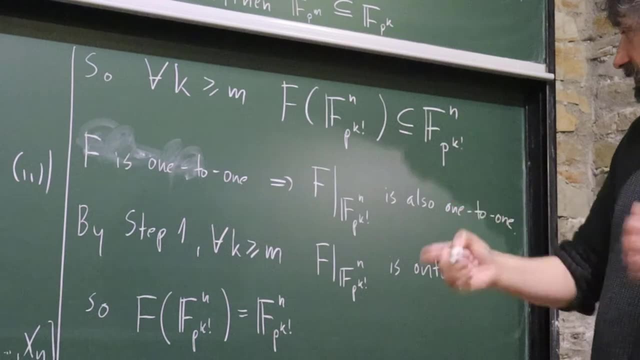 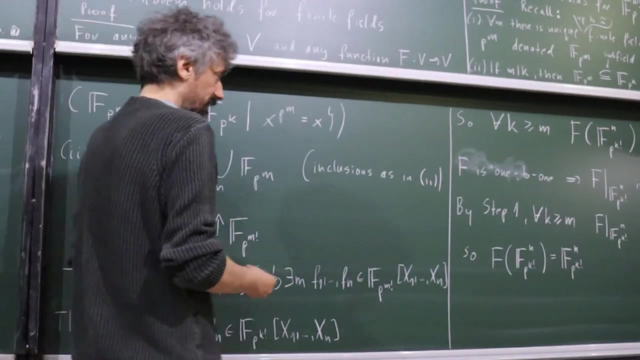 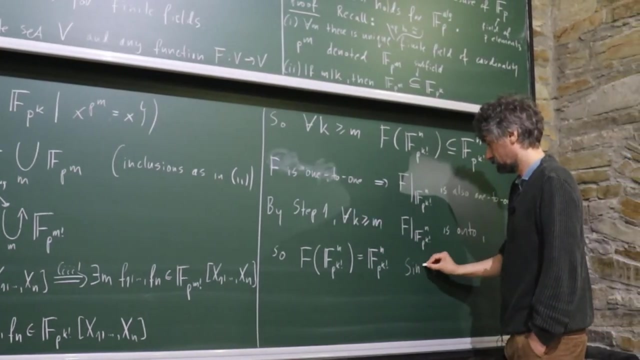 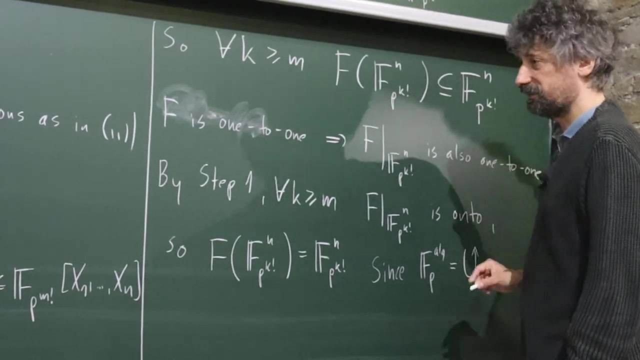 come on, you have the first function and of course you have to come to the nice fundamental term Eb. but then it means if for all k, but now our fp arch is union of all these fields. so since, yes, i can start this union, i don't have to start from the very beginning, i can start on any. 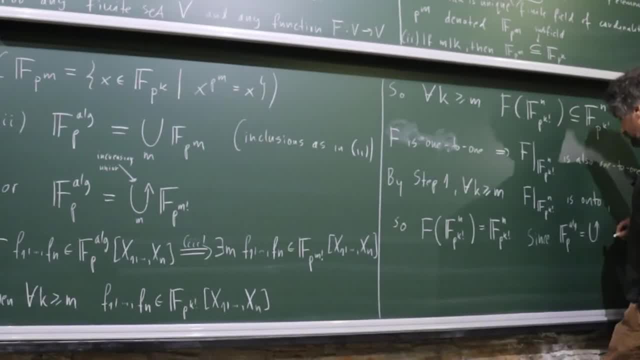 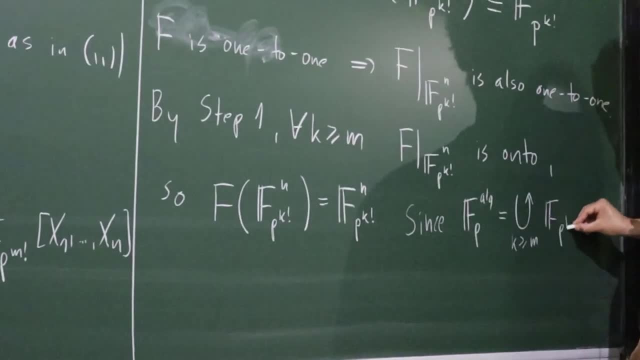 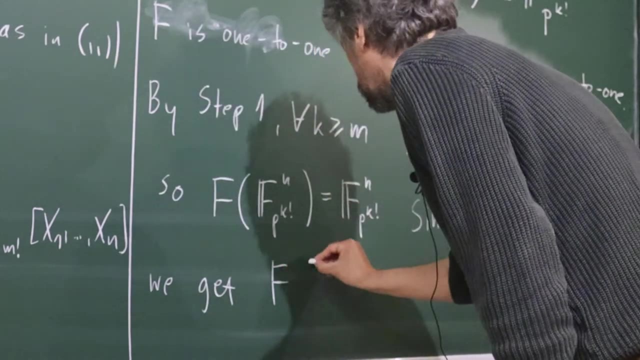 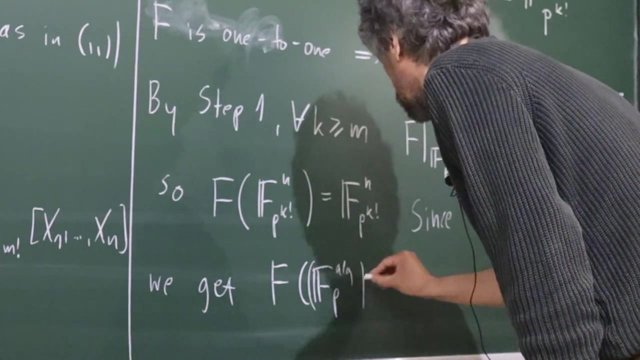 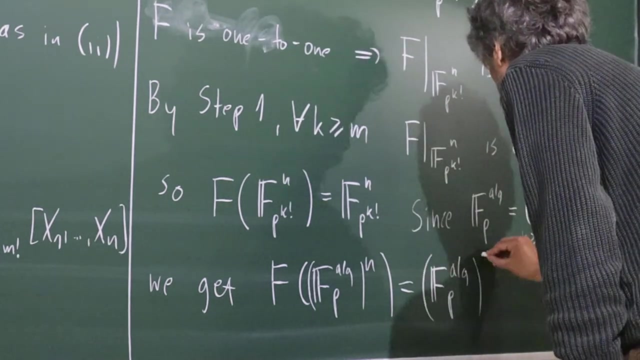 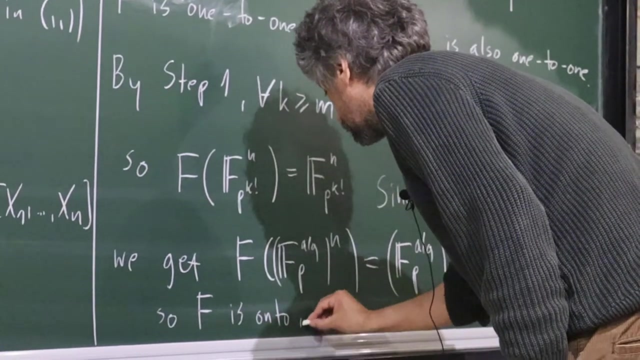 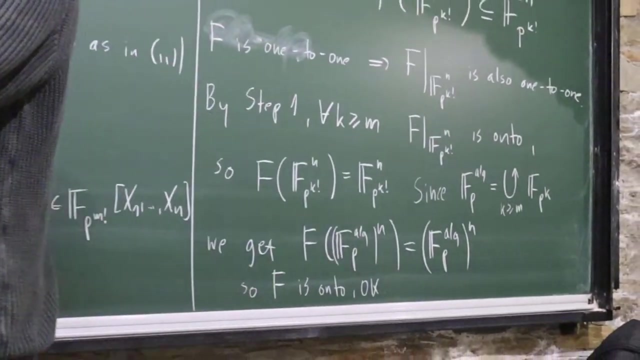 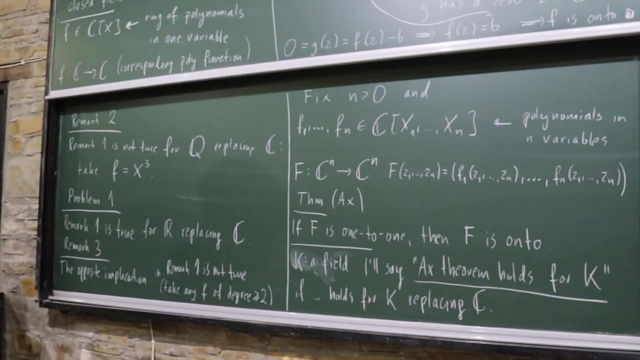 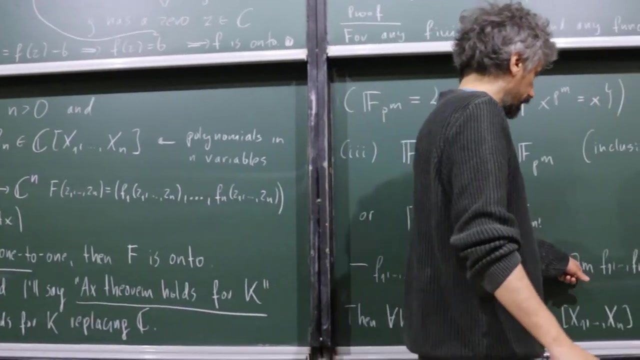 from any moment. so since fp arch is the union, like this, we get that f. fp arch n equals fp arch n. so, okay, f is onto as we wanted, because it was onto on each finite level from some point on. so let me wait any question to that. yes, somehow from some point on from this finite. 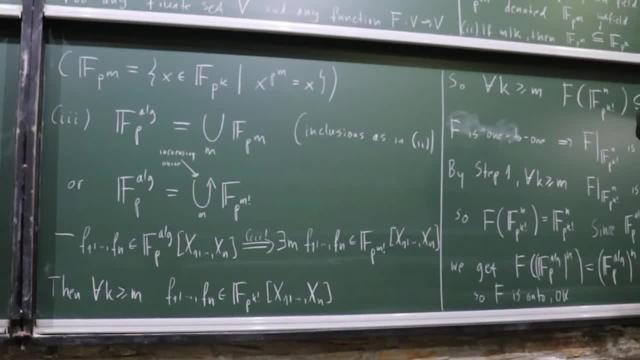 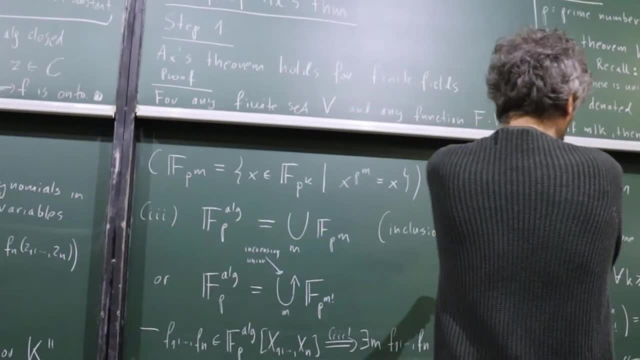 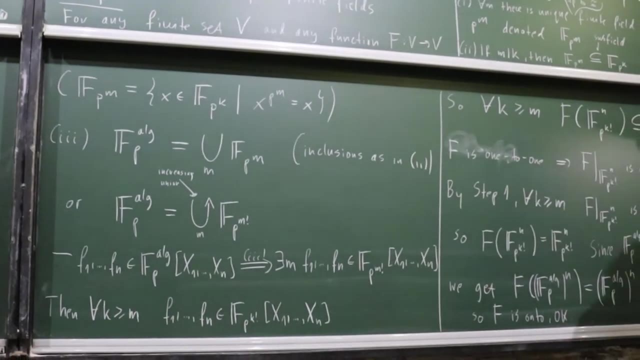 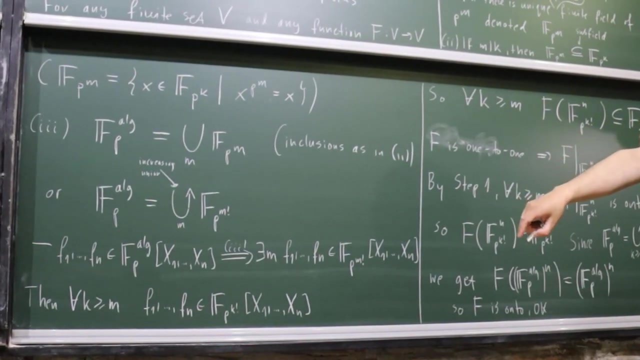 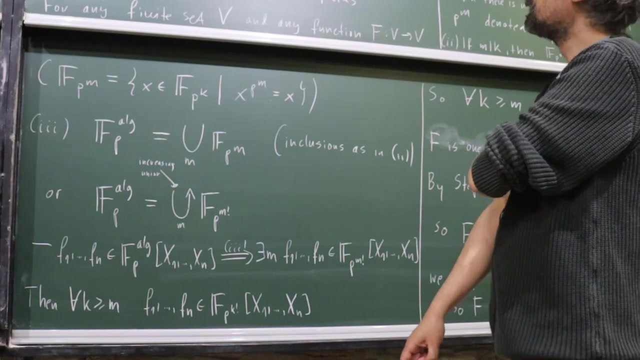 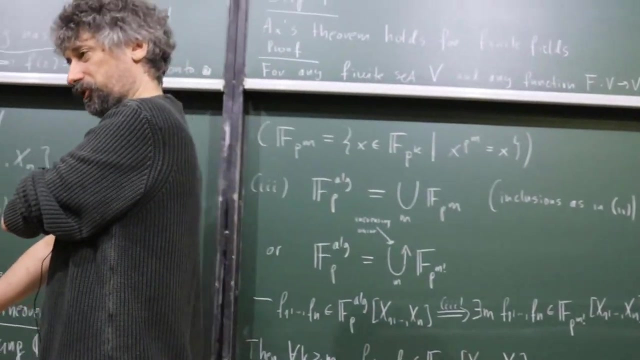 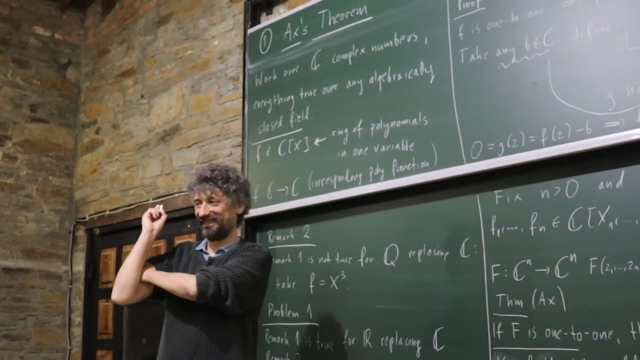 level m, everything was controlled on this finite levels, and on finite levels function was onto by, by step one, so it was onto on on the full field. so question to you: what would go wrong if you were trying to prove that onto implies one-to-one one, because step one is also true. 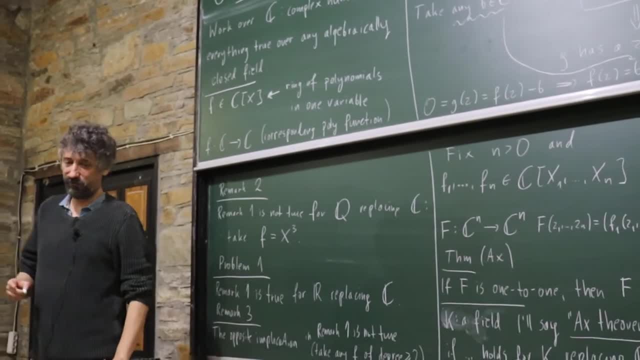 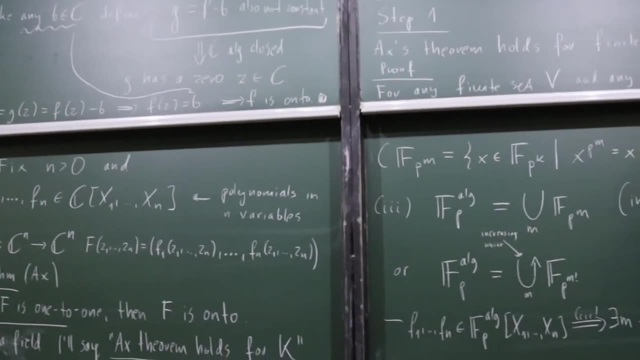 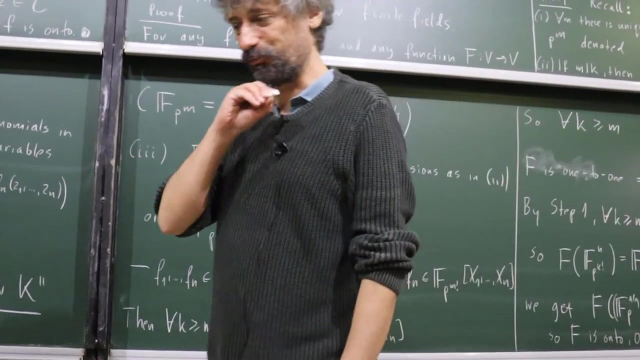 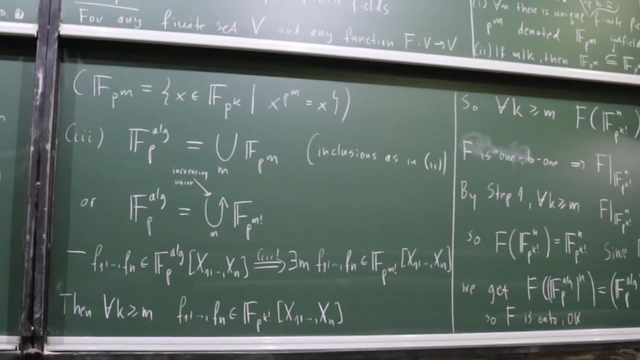 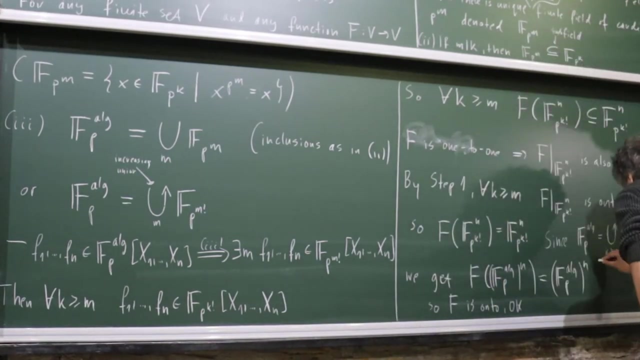 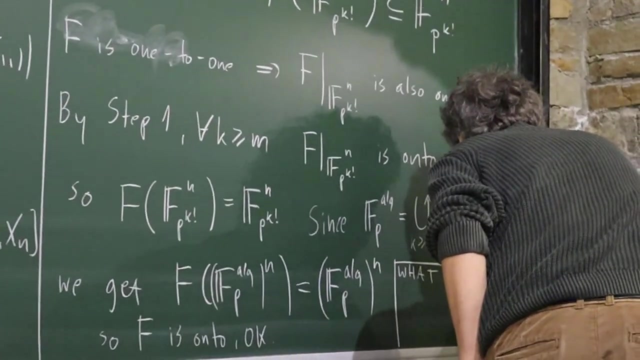 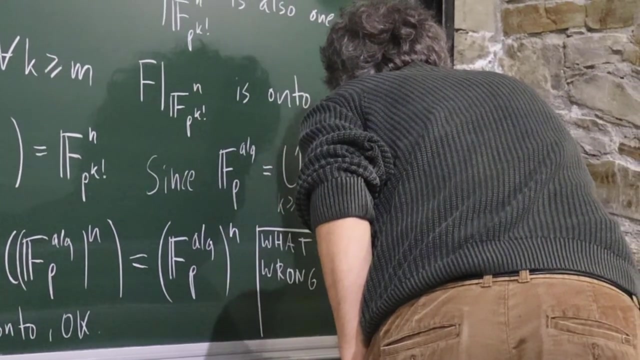 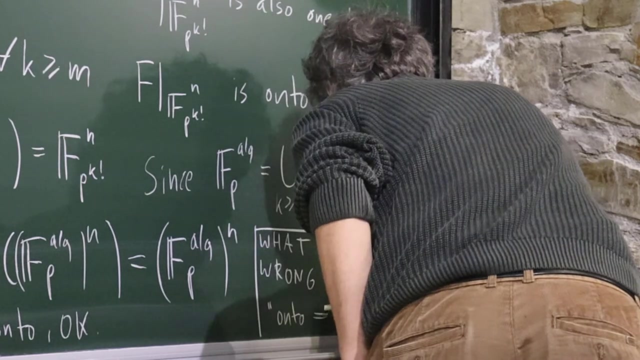 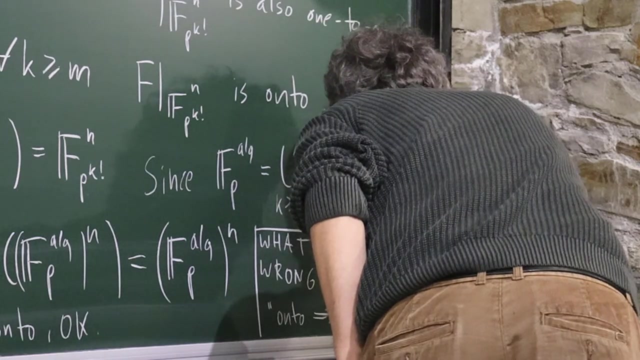 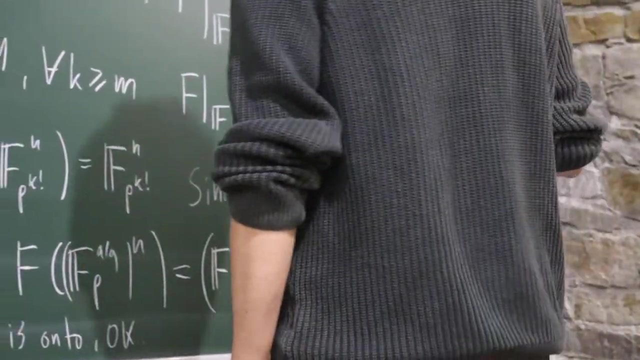 for the other direction, but on fp-alt it is not true. so what would collapse? it's a good moment to pause, so let us think. maybe broadcasting thinking will be will not be so great. so question: false implication. ah, okay, that's so we can think a bit. this may be. 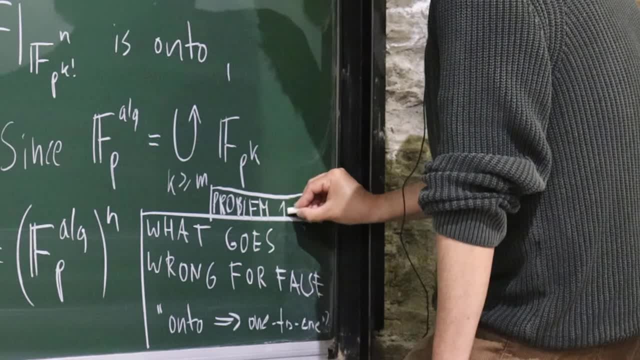 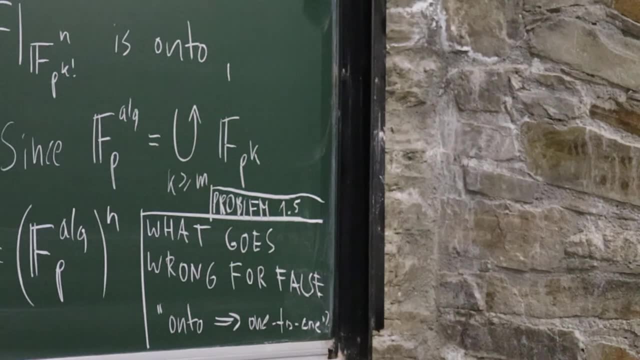 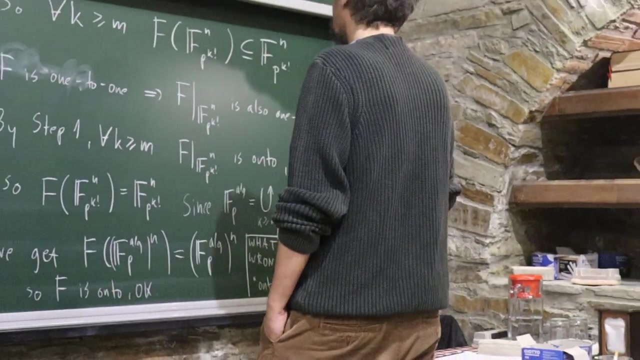 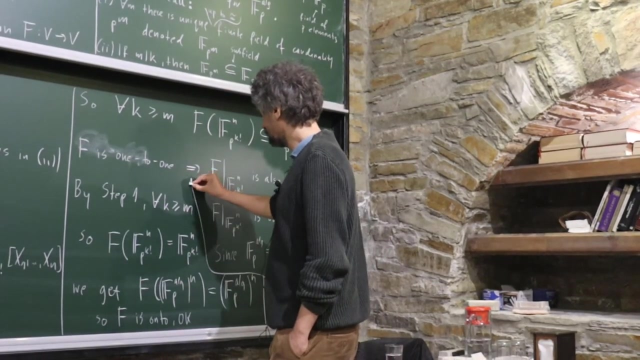 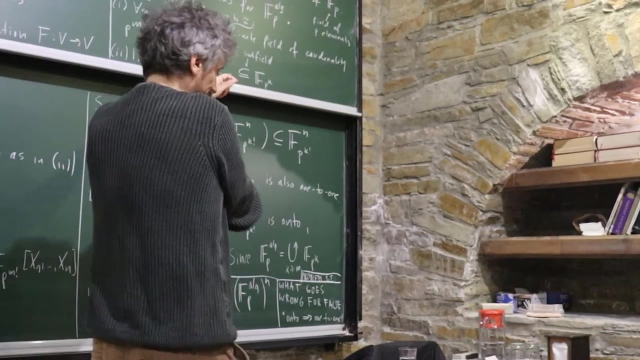 problem: 1.5, one and a half, yes, yes. so what is wrong? yes, so one-to-one goes to, goes to smaller things, but on on to ness does not. so it's not. so this one, okay. so the answer is this: this implication would not be true if we yes, so this is how the other thing breaks. 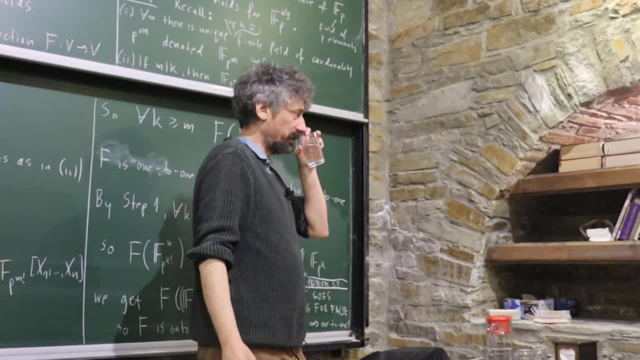 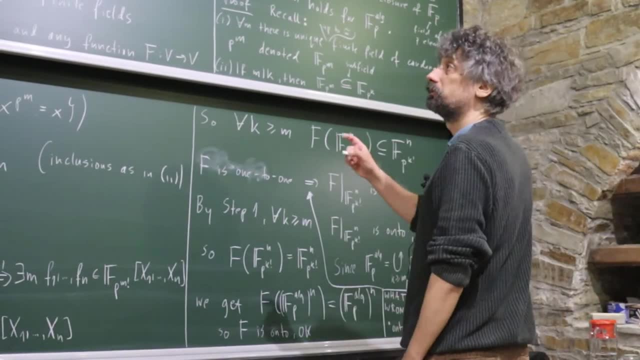 that we cannot. we cannot kind of lift this other implication to, to the union. okay, so we have step two. now, finally, the last one: 2.0, 1.8, 1.9, 1.8, 1.9, 1.9, 1.9. 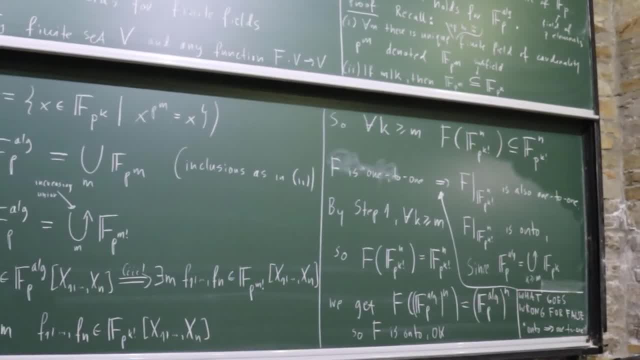 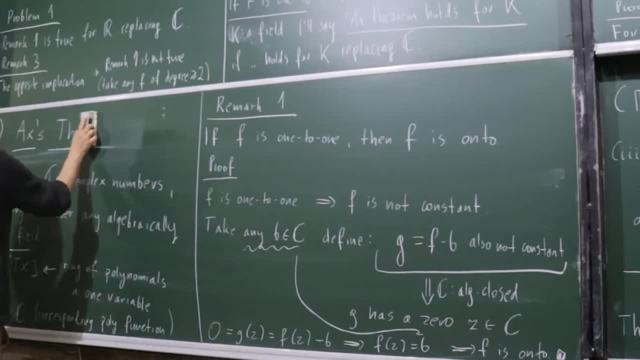 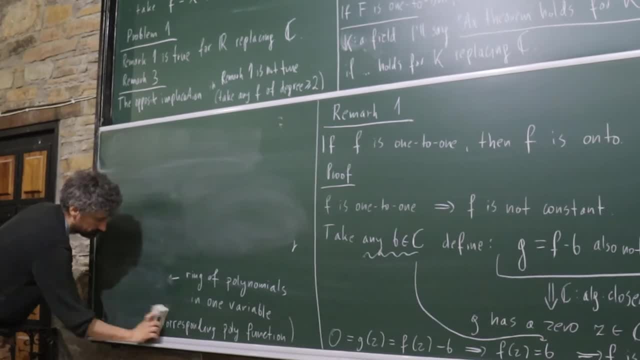 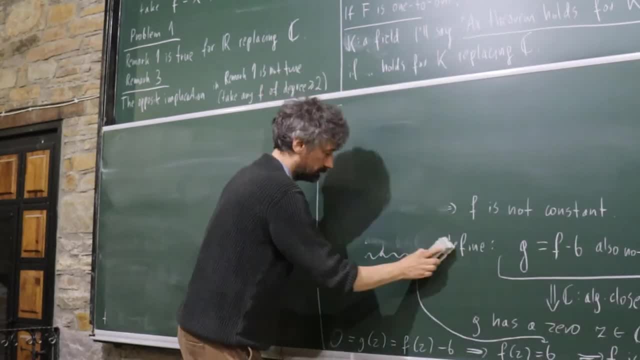 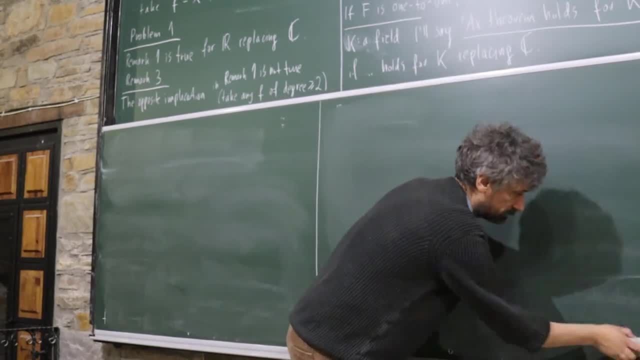 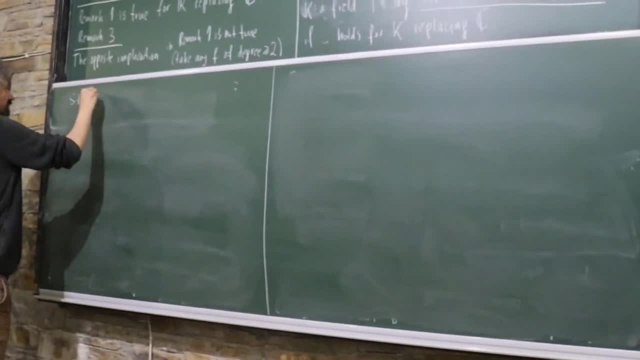 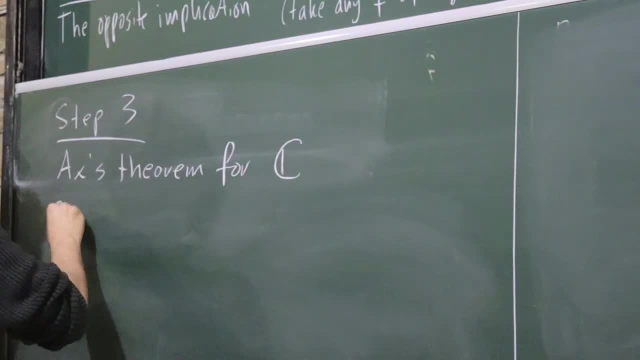 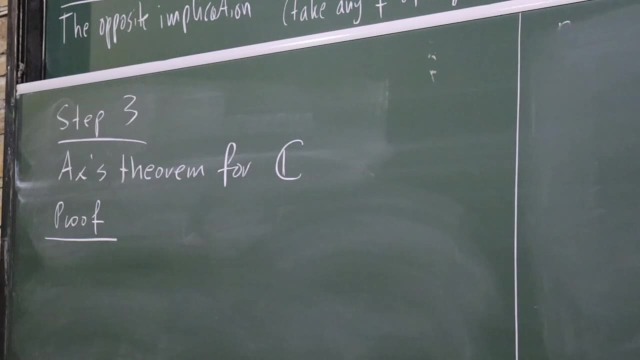 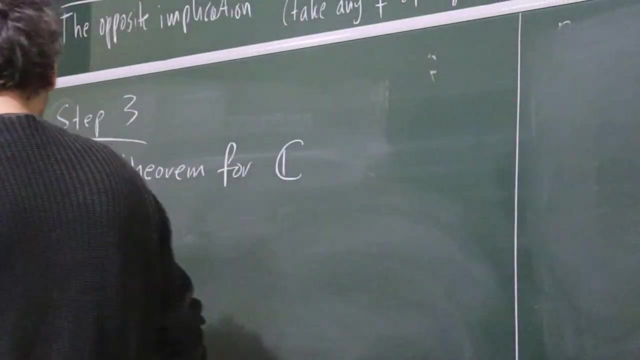 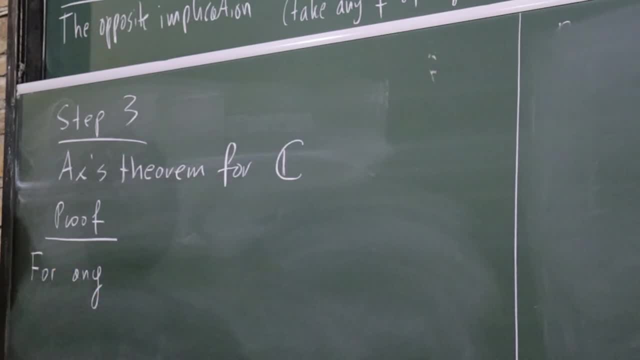 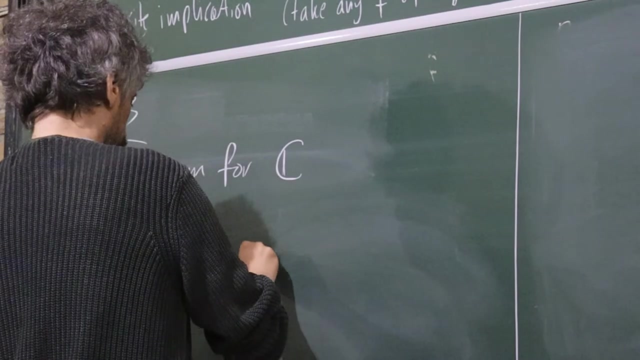 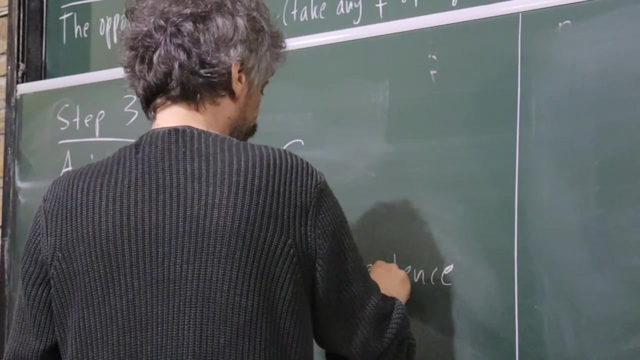 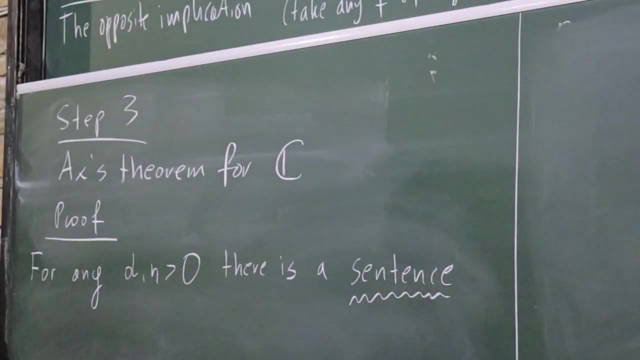 what I mean by this. so I'm saying that for any d which hasn't appeared yet, it will be like degree and our end. there is sentence, so this will have a proper meaning, like sentence. you know what is sentence in a language like English, Turkish or Polish, but this will. 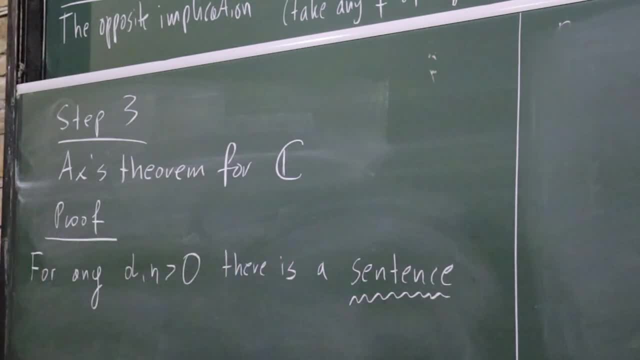 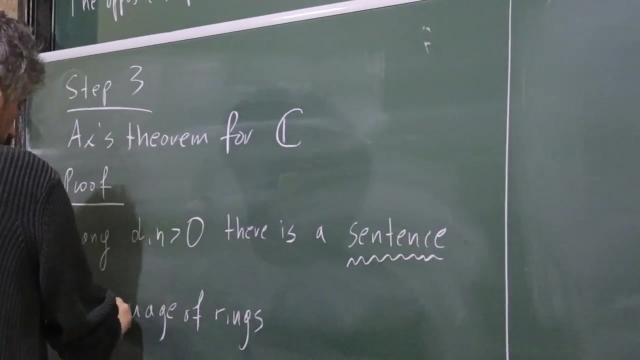 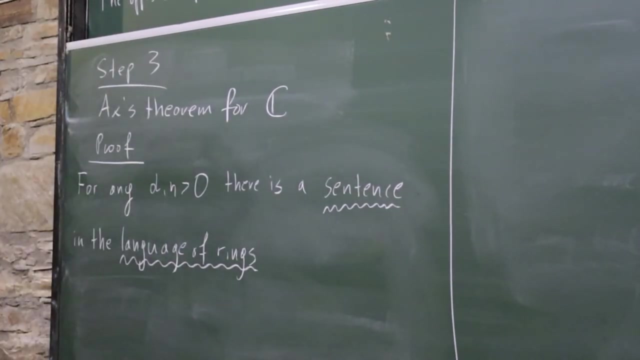 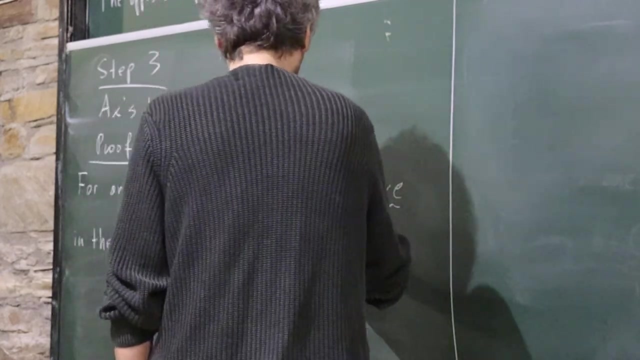 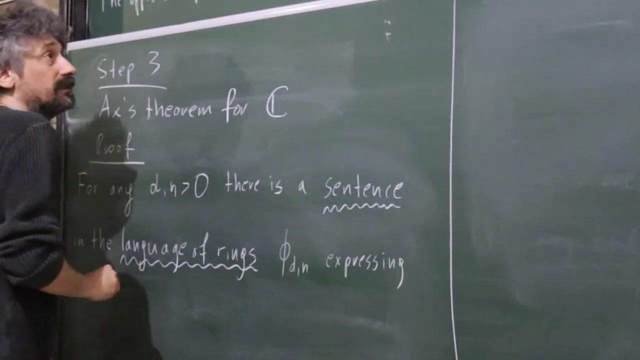 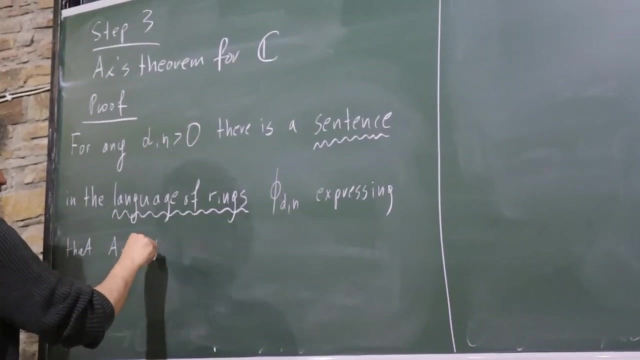 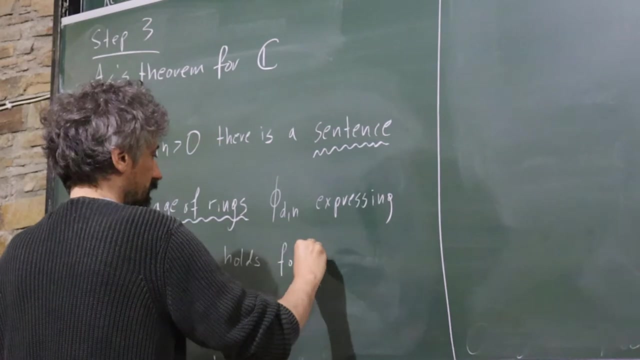 be something very precisely defined in next lectures. there is a sentence nd in the language of rings, so this will be also properly defined. now we will just have some intuitive meaning. let us call it v? dn, expressing that access theorem holds for those f1, fn, but with extra restriction. 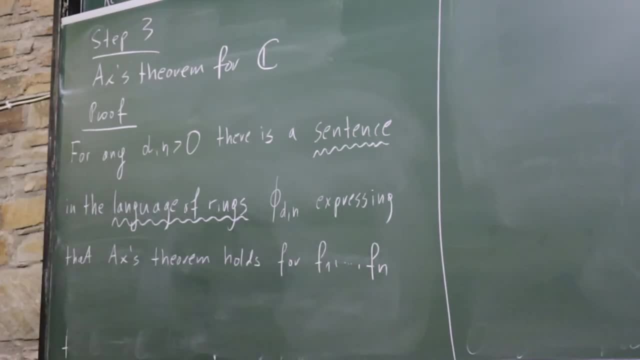 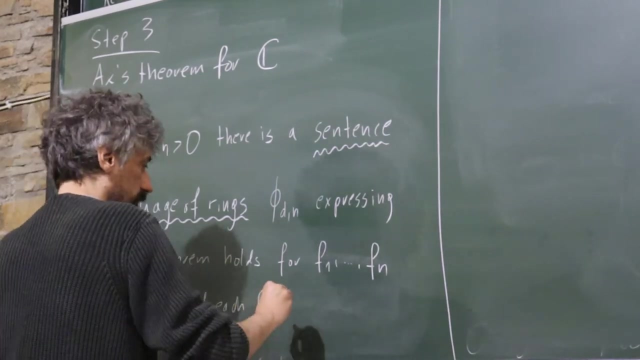 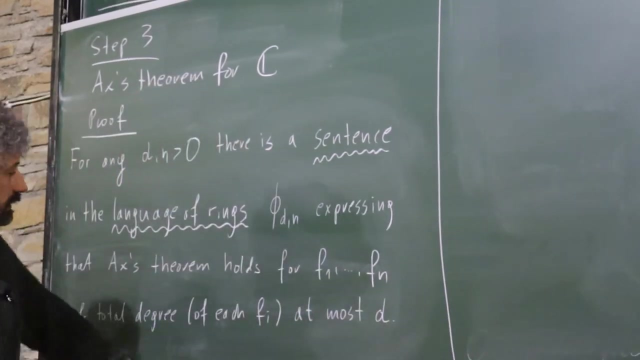 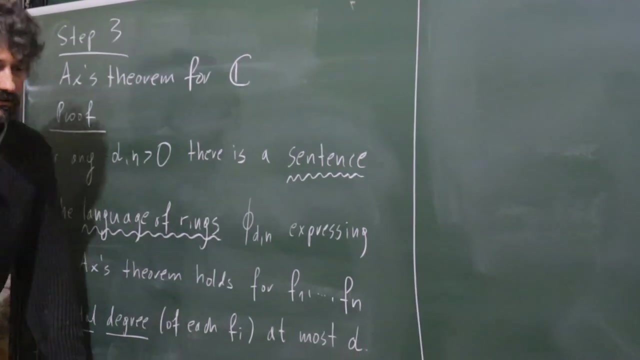 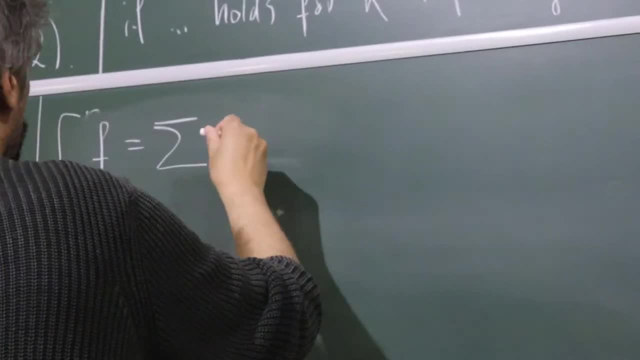 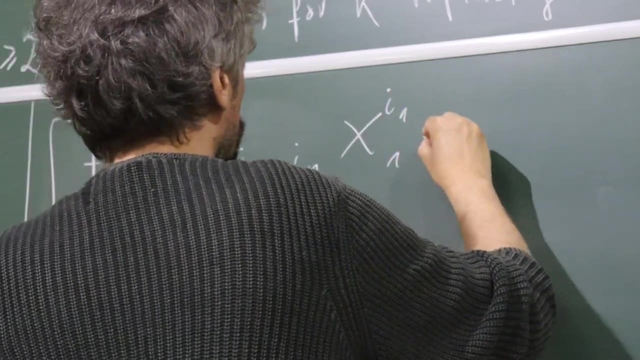 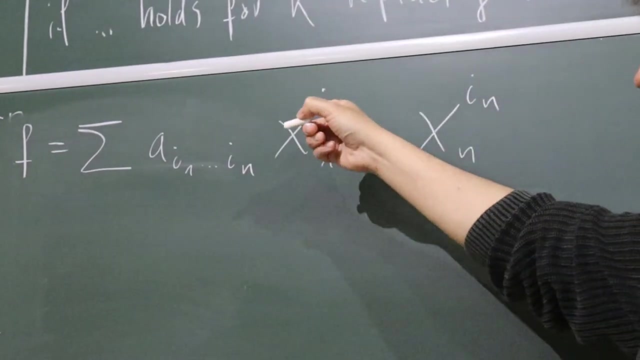 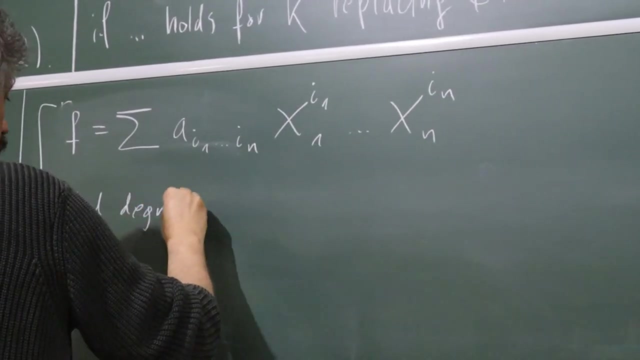 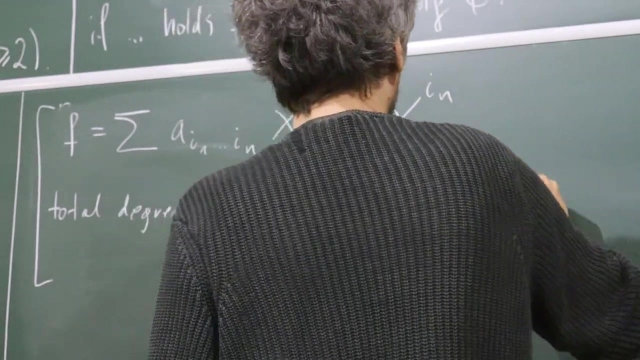 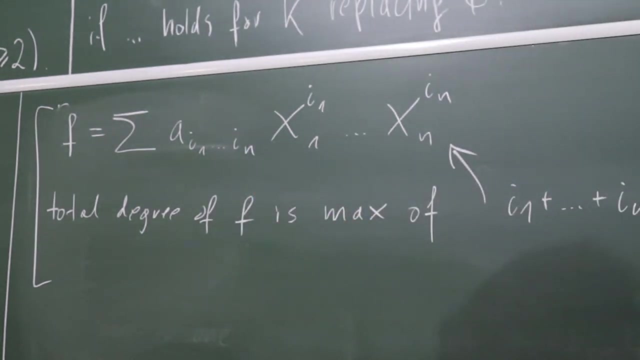 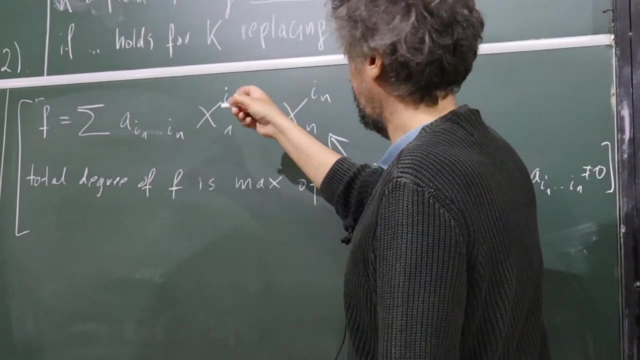 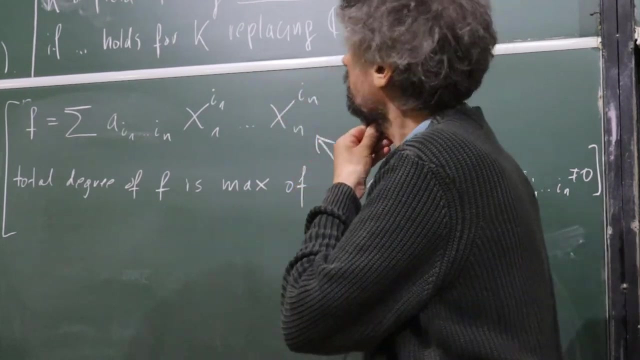 then total degree is just sum, maximum of the sums. when you so, I mean of course such that, yes, so just the sum of the degrees of the monomials which appear. ok, so at this moment, ok, you may ask what do I mean? and I will not explain it to you. 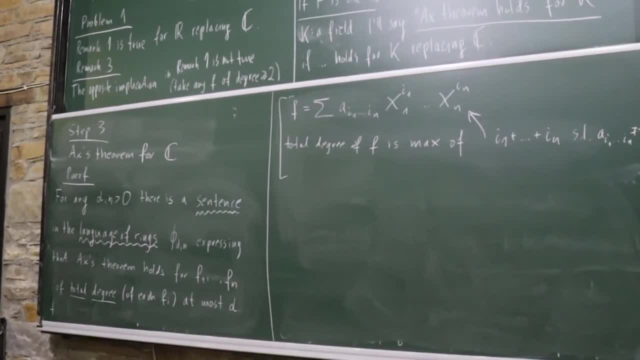 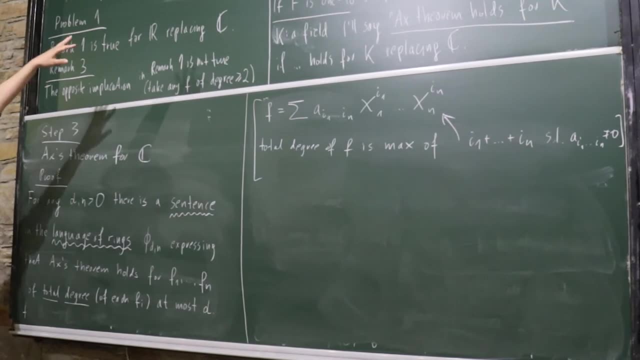 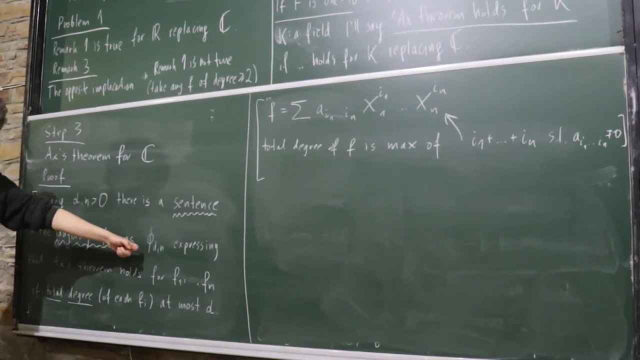 I will explain it now. I will explain it a bit later, but if we, the point is that if we bound the degree for each- but always of course any such f1, fn, they belong- there is some d which bounds the total degree, so there is always. 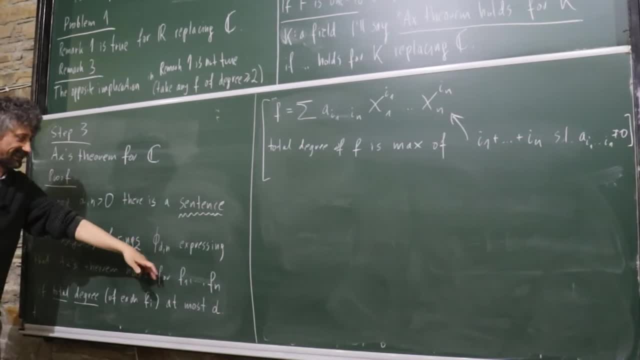 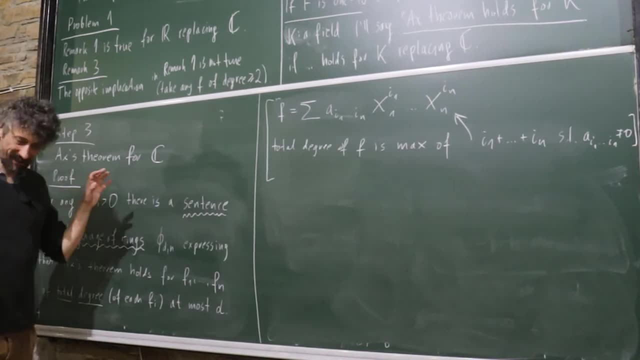 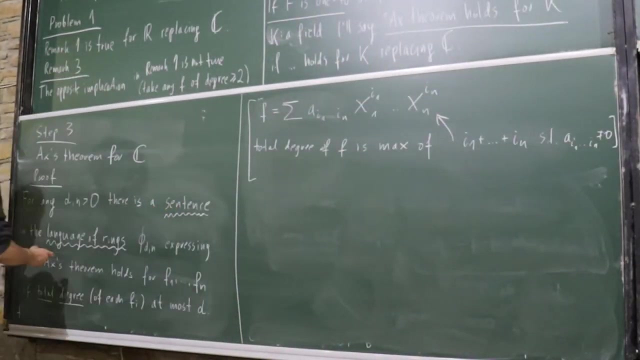 for any given capital f. there is a sentence like this expressing that access theorem is true for this kinds of capital f. ok, but there is no one sentence for all possibilities. f is not possible, fs- we will understand it later, so first we have to accept it. this notion makes sense. 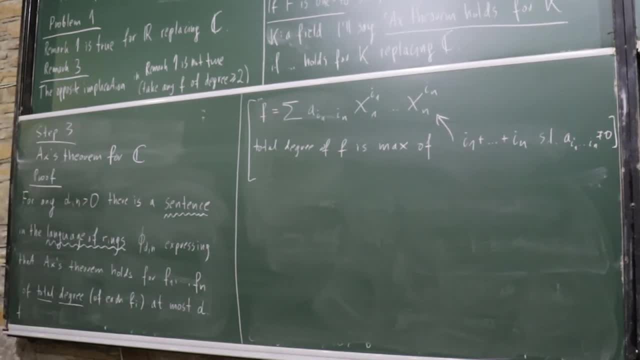 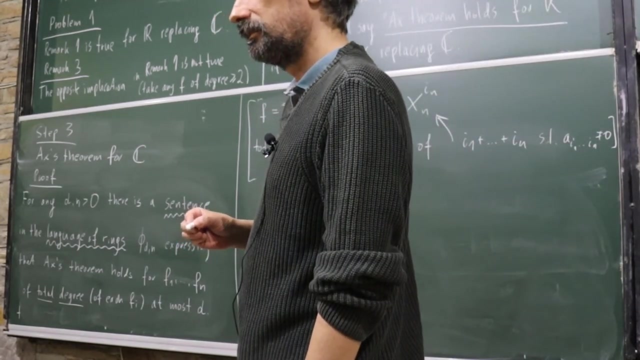 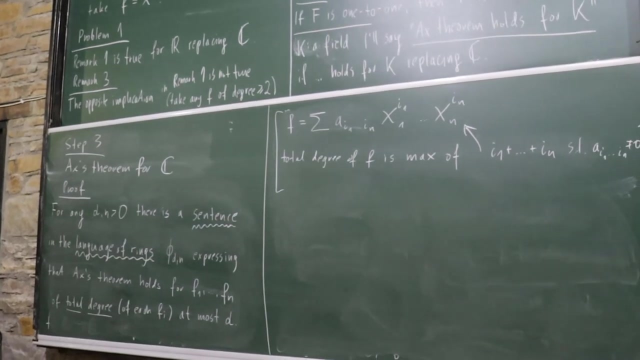 and such a sentence exists. I will describe what it means after this and the second example. and then there is a theorem, model, theoretic theorem. it's not hard thing to write, this first order sentence. ah, there will be, it is. it's not. it's not hard to understand, it exists. 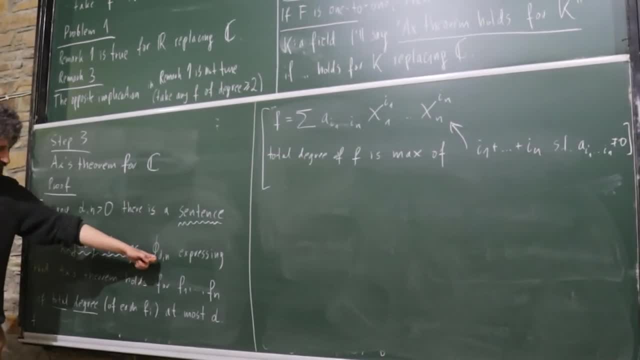 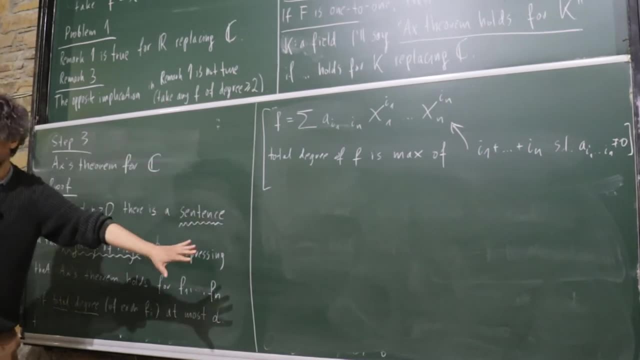 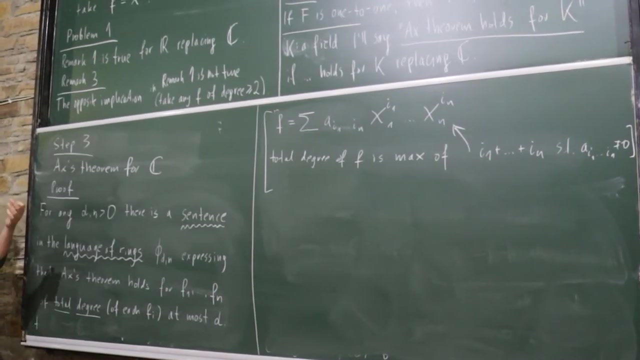 but we will soon see example. we will write this sentence for d equal 1 and n equal 2, and I think this board will be barely enough. ok, because it's clear how to do it, but when you start writing, it suddenly gets long, long, long, long long. 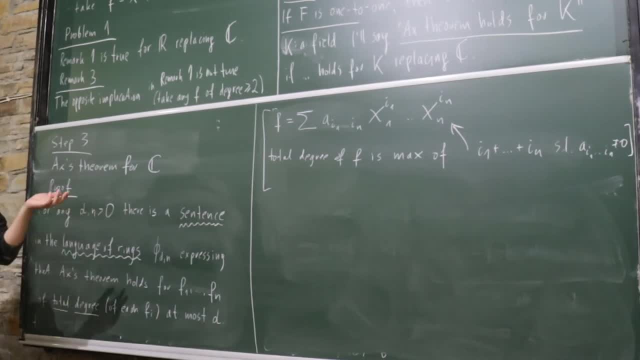 ok, so it depends what you write. what do you mean by easy? anybody can do it if you have a big board and time. I was thinking writing statements: yeah, probably if you have some experience, you see it's possible already. yeah, but I'm assuming you don't even know. 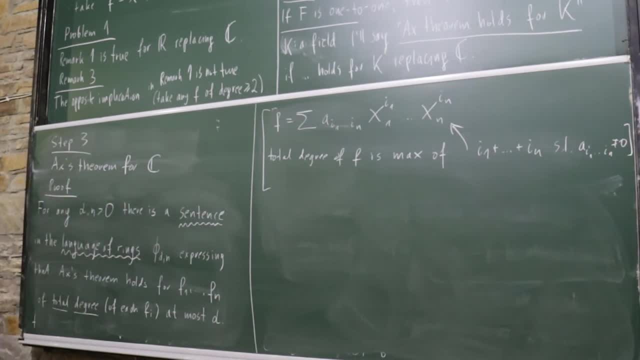 people don't even know what it means. is there a trick? do we need any trick to write? yeah, so you can also see. probably it's impossible to do it for all possible degrees at once, but if you bound the degree, it's possible. ok, but still it's not over, of course. 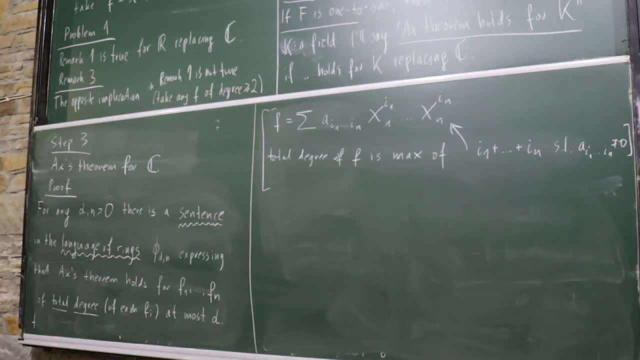 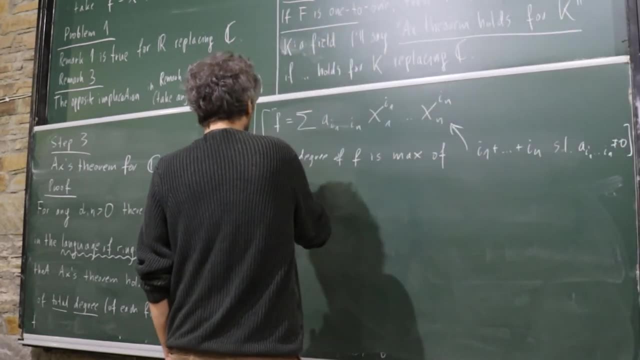 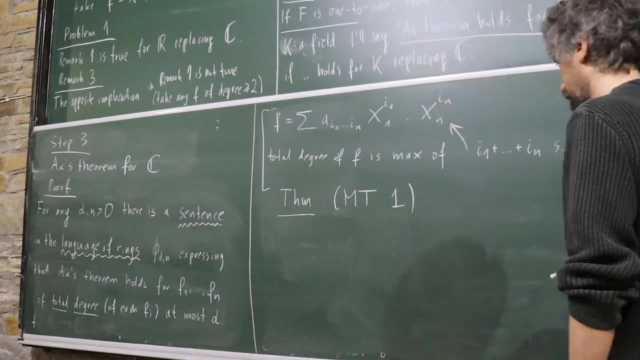 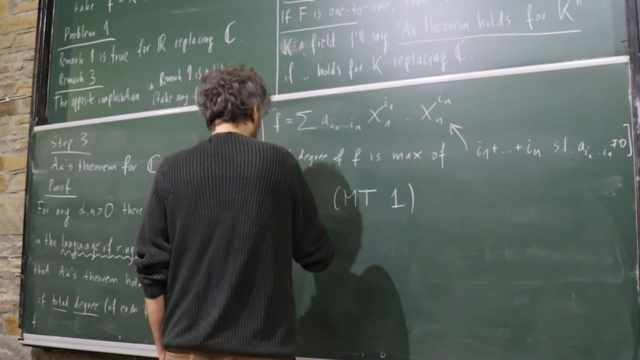 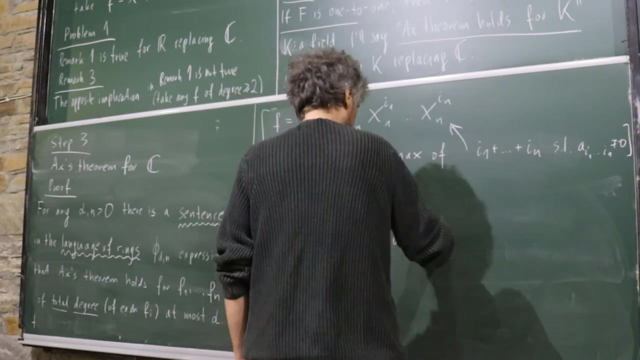 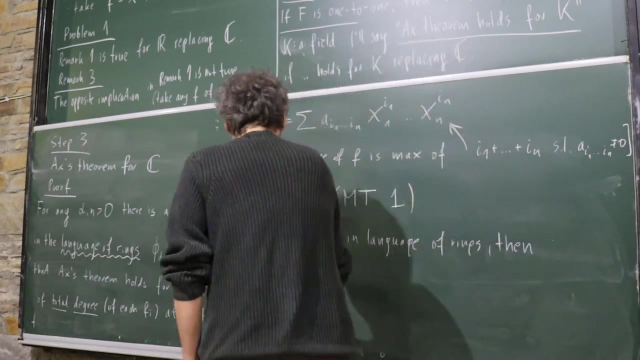 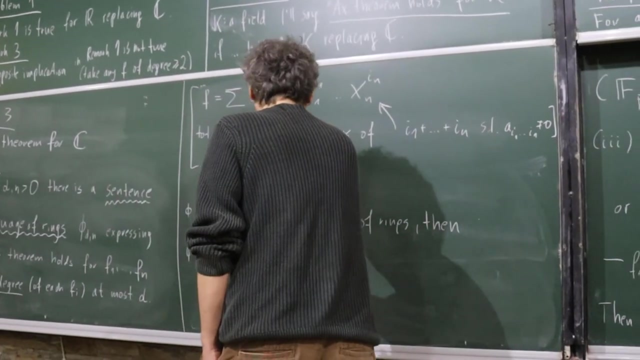 what's the time? ah, so I have two minutes maybe, so I'm so theorem. so this will be model theoretic theorem number one. so for any. so if phi is any sentence in language of rings, then phi is true in complex numbers if, and only if, for. 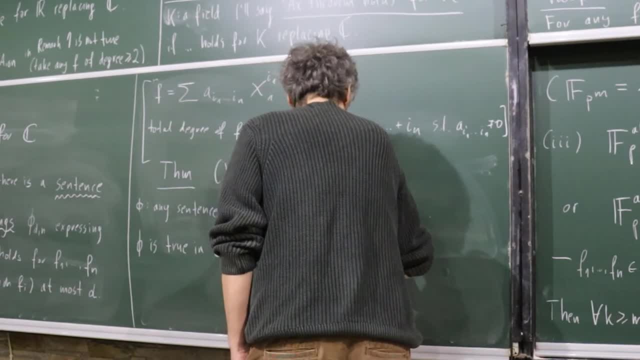 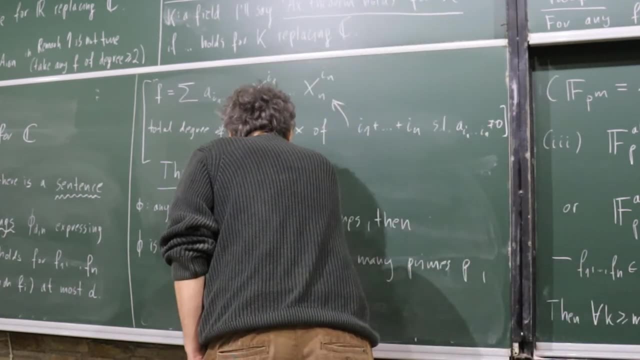 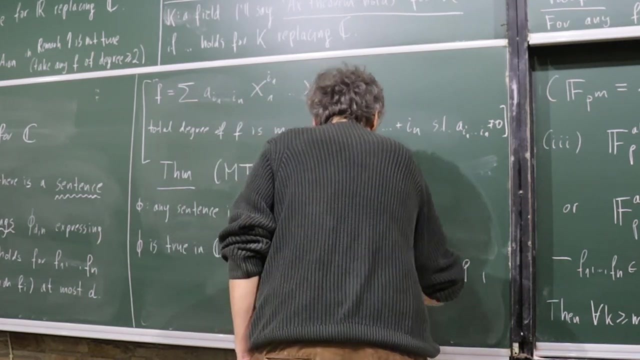 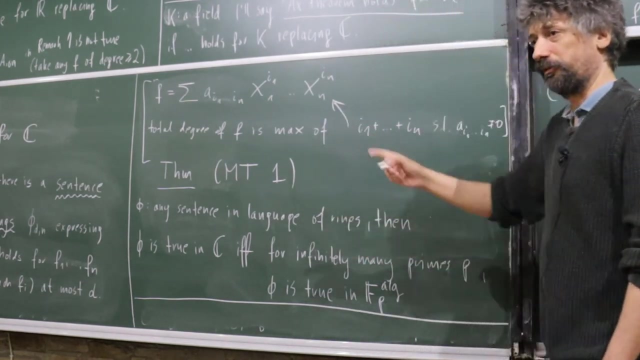 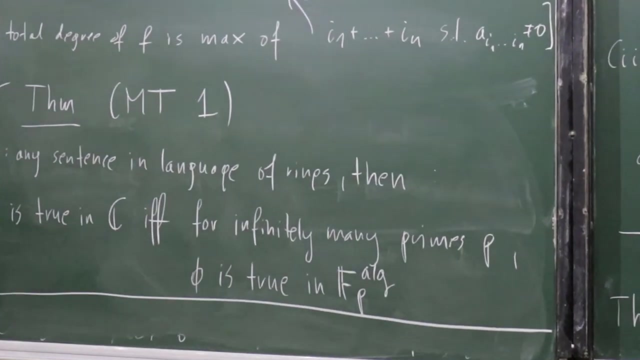 infinitely many times p is true in fp arch, so that would require a bit of, so we will prove it maybe in in the third or fourth meeting. yeah, so this is like example of model theoretic statement, something talking about sentences and how are they true in one piece? 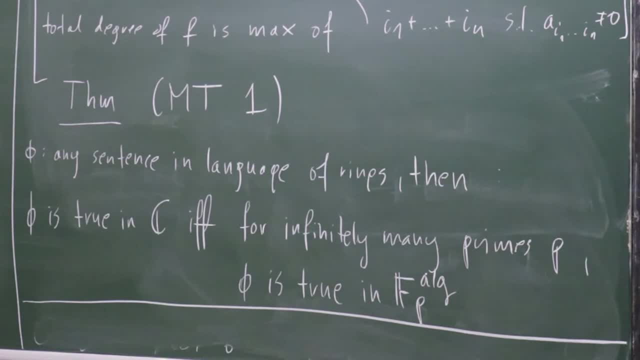 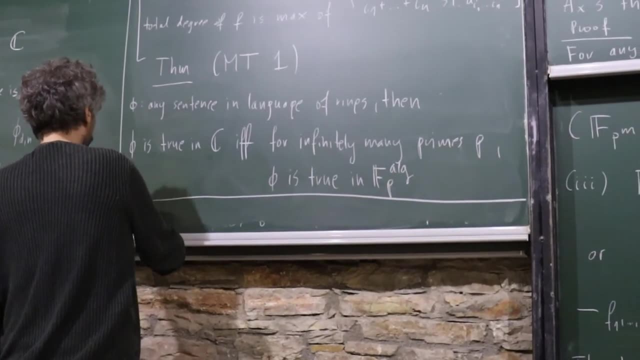 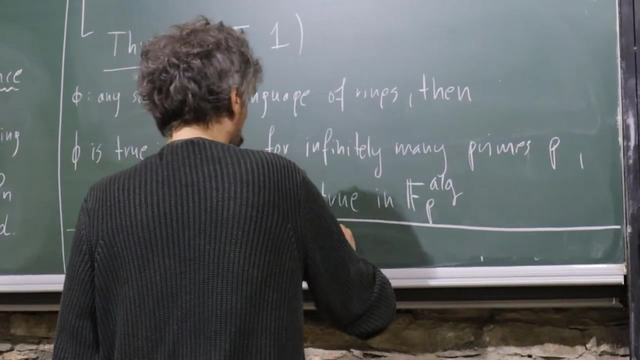 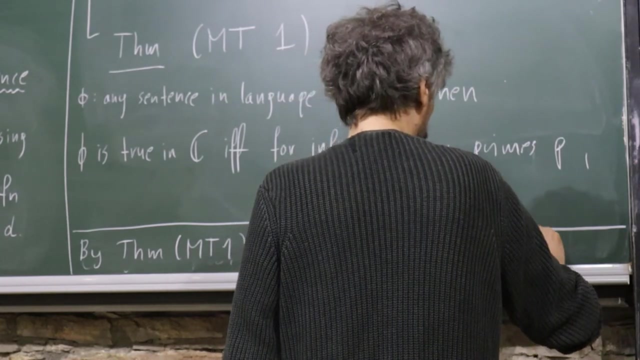 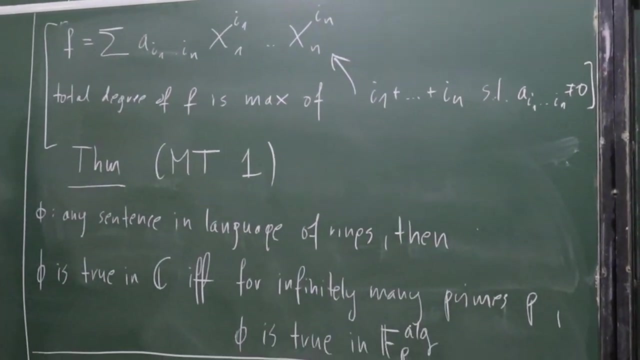 and in the others. okay, it's also called Lepchet's principle. so then I hope it is clear that by theorem empty one and step two we are done okay. so okay, this may be good moment for break and maybe 45 minutes passed, so okay. but 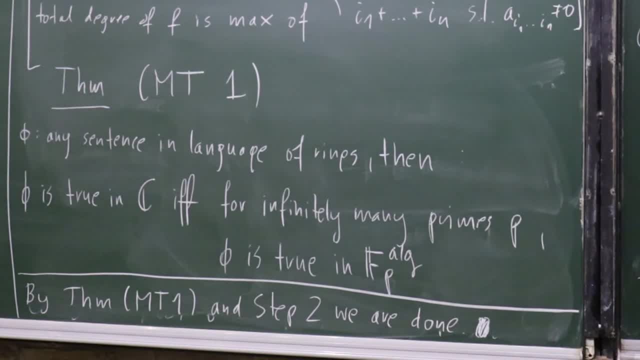 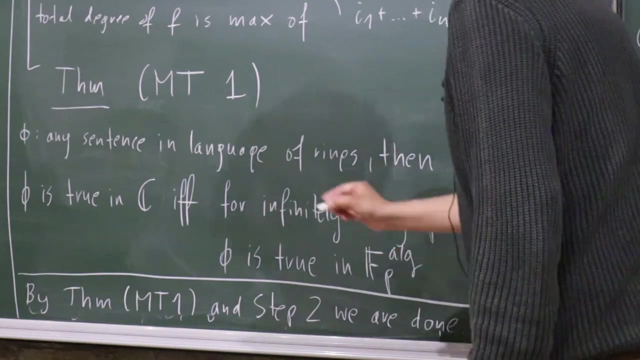 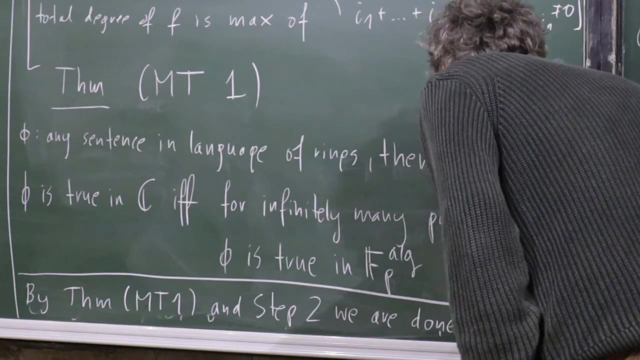 okay, if we can, questions for that, for that, for that theorem you. you have proved that by theorem empty one and step two. we are done. for theorem empty one, right, so so we are done. meaning step three is done, step three, okay, sorry, I thought that we are not already.